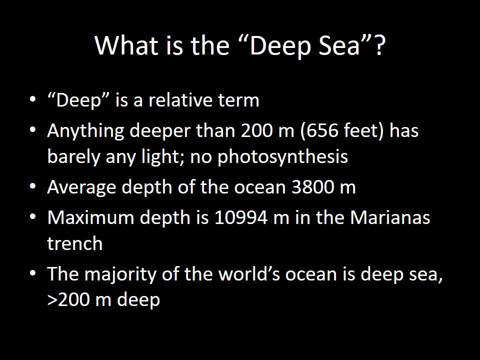 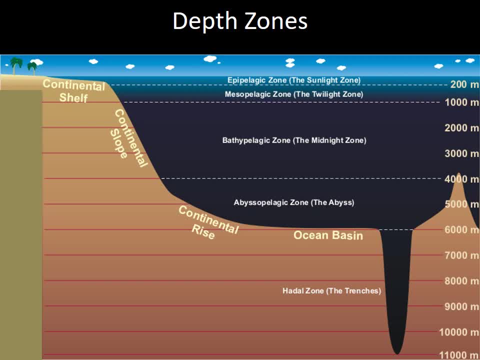 those are small potatoes in size anyways, compared to the deep sea. So this is subdividing the deep sea into a few more depth zones. So this surface waters go by various names. Some people call that the epipelagic zone, Some people call it the euphotic zone or the sunlight zone, And that's the waters above 200 meters depth where there is some light for photosynthesis. Some light does reach below 200 meters And the zone between 200 meters and 200 meters is the deep sea. 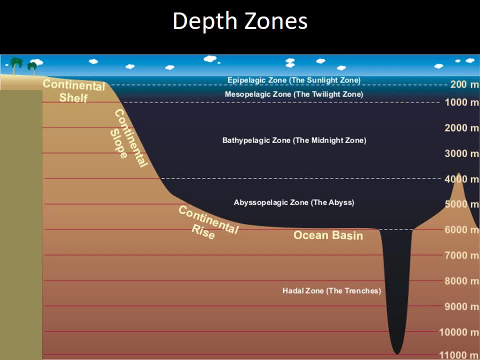 200 and 1,000 meters is referred to as the mesopelagic zone or the twilight zone, meaning that it's got traces of light but not enough light for photosynthesis. Below 1,000 meters there's definitely no light at all, And that's the bathypelagic zone or the midnight zone. Below 4,000 meters, which is deeper than the average depth of the ocean. you call the abyssopelagic zone very deep waters, And then the hadal zone after the Greek Hades is the very deep waters found in the ocean. 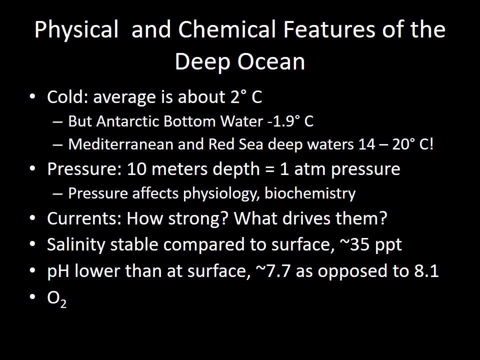 So the deep sea is cold. The average temperature is about two degrees Celsius, but it's not always exactly the same temperature. It depends on where you are in the deep sea and what water mass you're in. So scientists, oceanographers- classify the ocean into different water masses depending on their physical and chemical characteristics, And one of the characteristics that defines different water masses is their temperature. So there's a water mass. 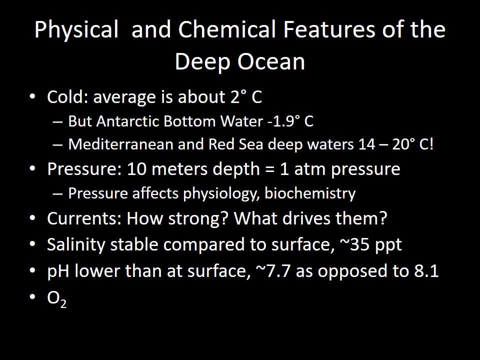 found in the very deep sea that originates in supercooled surface waters of Antarctica And then, because those supercooled surface waters are so dense, they sink to the deepest parts of the sea And they call that the Antarctic bottom water. And that Antarctic bottom water is the coldest water in the deep sea. It's almost freezing: negative 1.9 degrees Celsius. On the other hand, there are some deep waters that are relatively 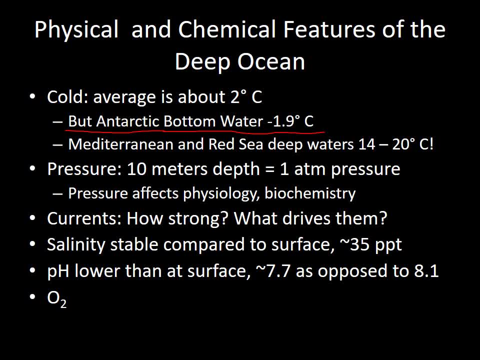 warm, like the Mediterranean and Red Sea deep waters, which are able to be dense enough to be in the deep sea, below the surface waters, because they're very salty. So even though they're relatively warm- and normally warm waters would be less dense and be at the surface- because these Mediterranean and Red Sea waters are salty, they can be dense enough to very salty. they can be dense enough to be deep in the ocean, despite having relatively warm waters. 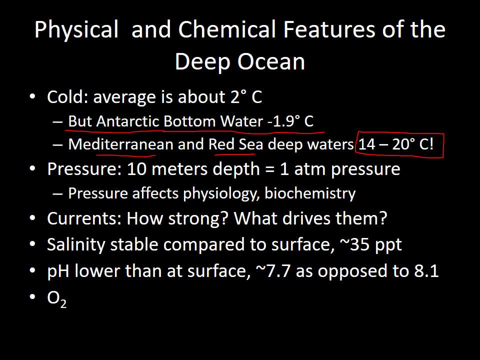 temperatures: 14 to 20 degrees Celsius. there would be a little chilly, but you could swim in that, if not for being killed by the pressures of the deep sea. So pressure, yeah, the deep sea has a lot of water pressure, because every 10 meters deeper in the water that you go, you're adding an entire atmosphere's worth of pressure. So the atmosphere of the Earth. 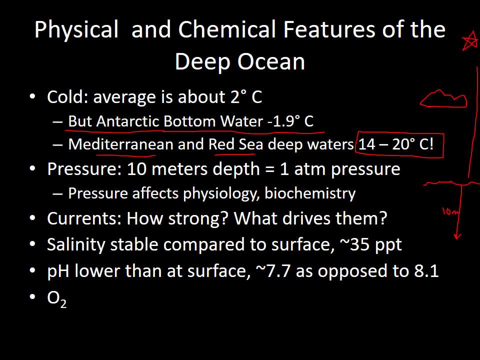 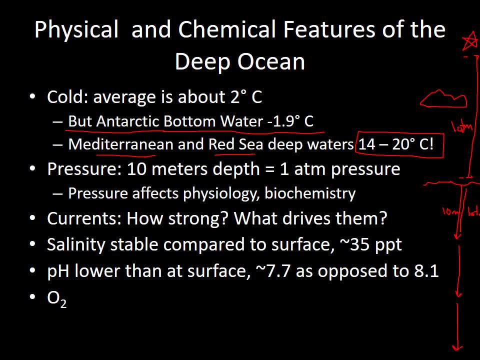 in the water you're adding another atmosphere of pressure. So by the time you get to the typical depth of the deep sea- 3,800 meters- you have many, many times atmospheric pressure crushing down on you. So that affects sea life in many ways. It affects physiology and biochemistry. One of the obvious ways that humans can perceive the pressure change is when we dive into the ocean. the water pressure squeezes the air spaces in our body, So we feel pressure in our ears and sinuses. 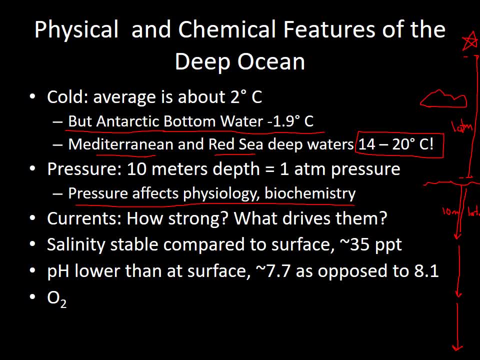 So we feel pressure in our ears and sinuses And we need to hold our nose and blow or do something else to equalize the pressure of our internal air spaces with the pressure pushing in from outside. Fishes that have swim bladders and marine mammals- any type of marine life that has an air pocket in its body- it needs to do something to adjust the air pressure in that air pocket as it rises and falls in the water so that it's not exploding or getting crushed. 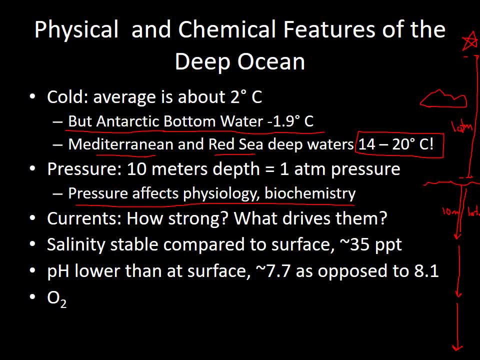 Things that don't have air spaces in their bodies are still affected by the pressure of the deep sea, though, because water under very high pressure changes the way biochemicals react with each other. We'll talk a little bit more about that when we talk about the deepest in the ocean that fish can live, but there are sort of physical, chemical effects of pressure on the way biomolecules like proteins and lipids interact. 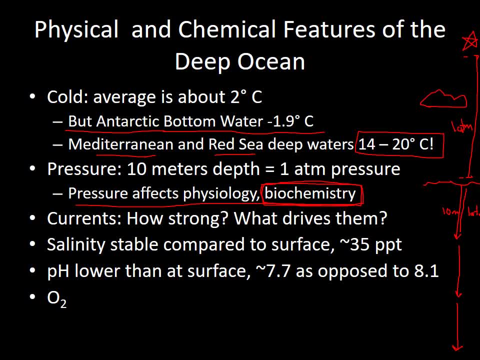 So adaptations for biochemistry that works well at low water pressures don't work at high water pressures. Moving on to currents, there are some currents in the deep sea, but how strong are they? They're generally not as strong as currents in the shallow ocean. 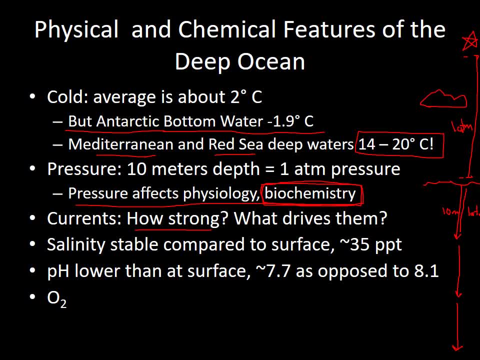 You're not affected by wind driven waves in the deep sea and so you generally don't have those wind driven currents Like the Gulf Stream. and what drives currents in the deep sea is mostly the third global thermohaline circulation, So they're sort of these large scale but usually slower strength currents driven by sort of the slow slumping of denser water masses down and lighter water masses being pushed up or up well to the surface. 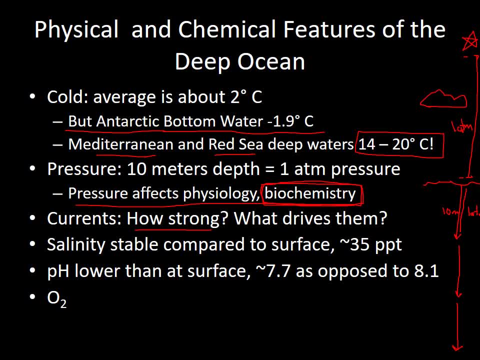 So there are some spots in the deep sea where currents are a little bit stronger, But for the most part they're not as strong. For the most part there's not as much current in the deep sea as in the shallow ocean. The salinity in the deep sea is stable and high compared to the surface. 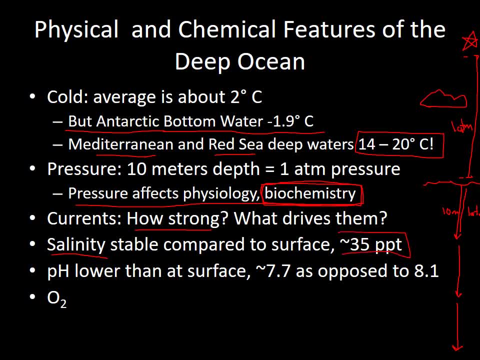 So, on average, the deep sea is about 35 parts per thousand. But, as I mentioned, there are some deep sea waters that are saltier, like in the Mediterranean and Red Sea waters, because those deep sea waters form from really salty surface waters that sink down to a deeper depth. 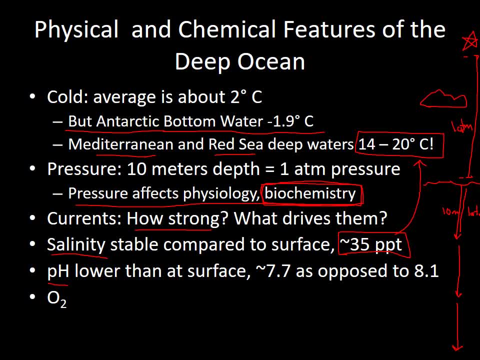 They are a little higher in salinity. The pH, the acidity of the deep sea is generally lower than at the surface, So the average surface salinity of the ocean is 8.1.. It used to be 8.2 before anthropogenic ocean acidification. 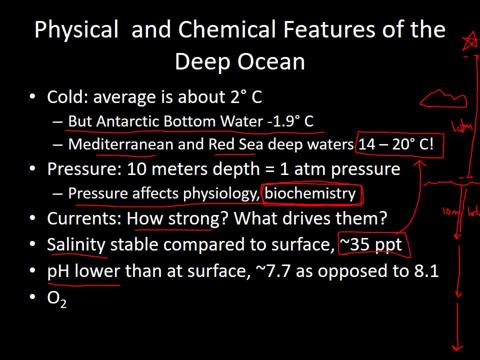 But the deep sea is naturally more acidic. So lower pH, about 7.7 on average. The pH of the deep sea is lower because in the deep sea there is a lot of decomposition of organic matter And no photosynthesis or exchange with the atmosphere. 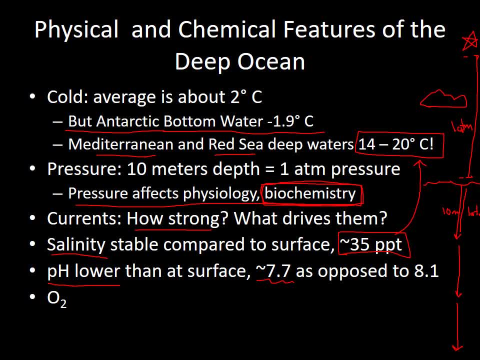 And that over time, causes a buildup of carbon dioxide in the deep sea, which becomes carbonic acid and lowers the pH of the deep sea. Oxygen levels in the deep sea vary from place to place. In the very deep sea, oxygen levels tend to be pretty high. 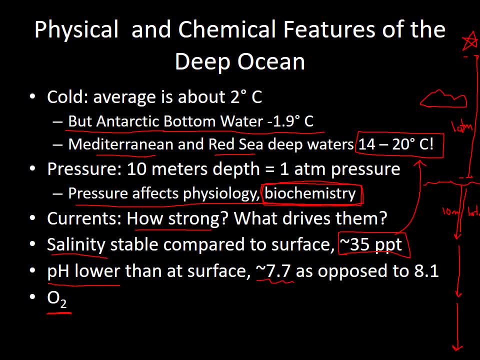 Because that deep sea water usually forms at the surface in well oxygenated water In the cold parts of the world like the Arctic and Antarctic, And so when that water sinks into the deep sea after being super cooled at the surface of the Arctic and Antarctic, 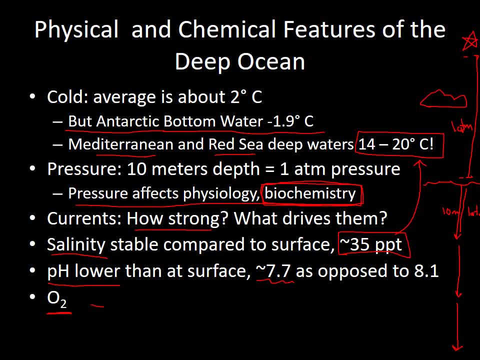 it keeps its high oxygen levels. So here's Antarctica. This is the Antarctic continent. So I'll make a little penguin on here. It's supposed to be a penguin. Give him some wings. So off the coast of Antarctica And there's some ice sticking off the coast. 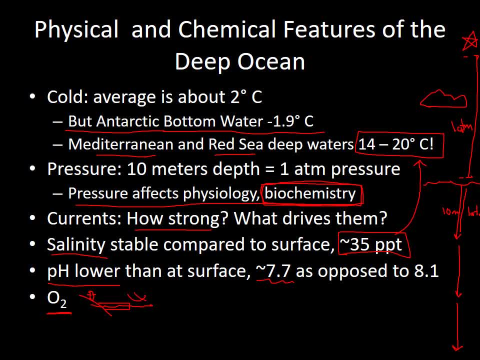 The cold winds blow on the water and cool it off, And that cold water then sinks to the bottom of the ocean. And this cold, well oxygenated water has a lot of oxygen in it, And so, even as it drifts and spreads through the deep waters of the ocean, 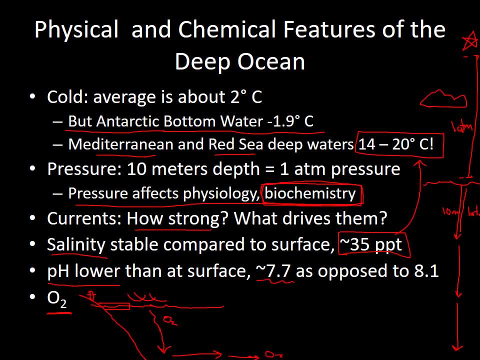 it still retains a lot of the oxygen that it had when it was well oxygenated at the surface. So even when you get towards- you know the equator, you still have this deep water in the deep sea that is rich in oxygen because it formed in cold parts of the deep sea. 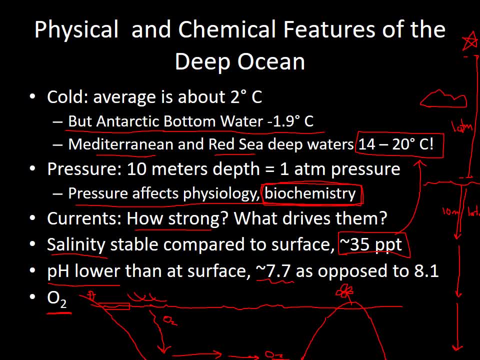 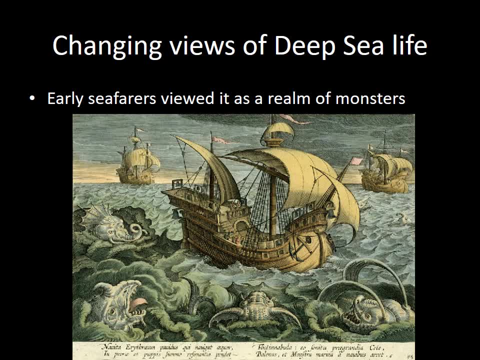 No, sorry, It formed in cold coastal waters off of the Arctic or Antarctic. All right, So changing views of deep sea life. We always were interested in what was in the deep sea, And back in the day before we had much reliable data on the deep sea. 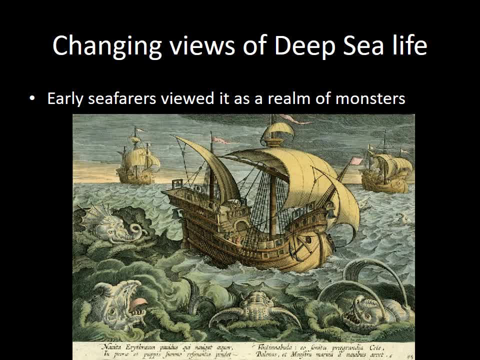 aside from the tales that sailors would tell when they came back from their voyages of what they'd seen out in the ocean, we speculated that the deep sea was full of monsters, dragons and serpents and whatever this elephant looking thing is. So when scientists started to actually investigate the deep sea, 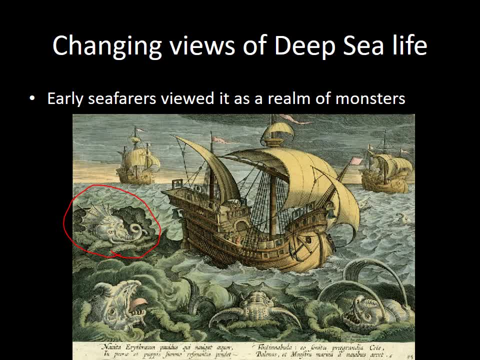 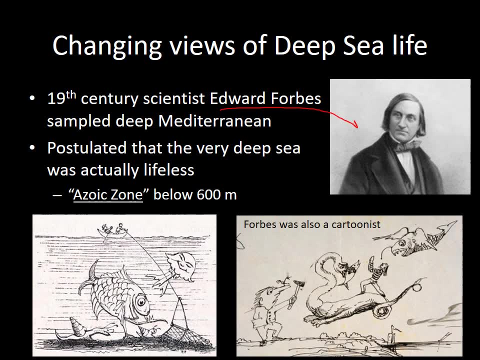 it was sort of anticlimactic because some of the first scientists, like this Edward Forbes fellow who actually started sampling at deeper and deeper depths in the ocean, what they noticed was that the deeper they sampled, the less abundant life they found. And so they sort of extrapolated back based on the fact that the deeper I sample, 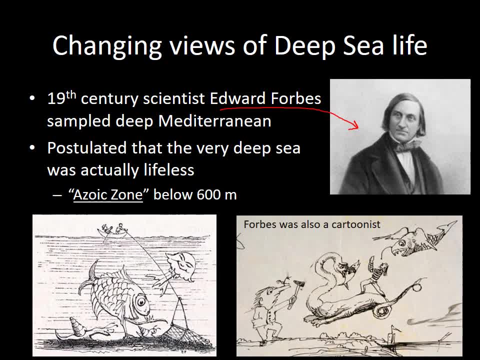 the less life I'm getting. that by the time you get to a certain depth- and Edward Forbes thought it was 600 meters- you're in a zone where there's actually no life at all. So, Edward Forbes, you know, even though in the moderately deep sea, 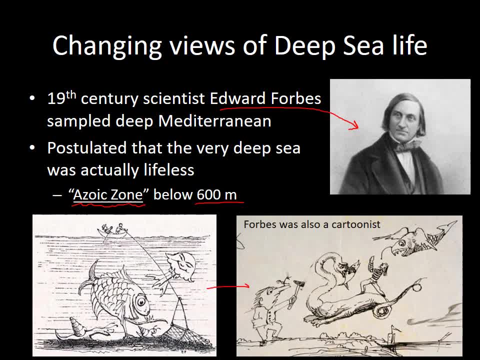 he was finding some interesting organisms which seemed to be have inspired some of his cartoons that he liked to draw here. He figured that, even though there's some interesting stuff down there, when you get below 600 meters it just fizzles out and it's a lifeless zone. 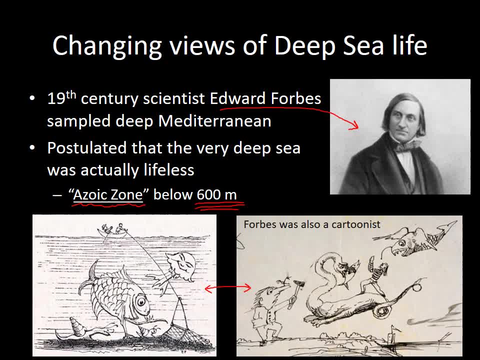 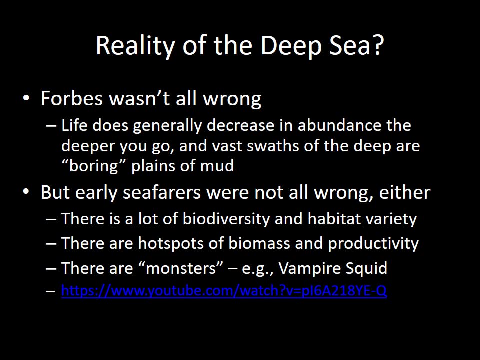 So what we have found when more scientists have sampled more places of the deep sea is that both the old view of the deep sea being full of monsters and the new view of the deep sea not having very abundant life- they're both right to some extent. 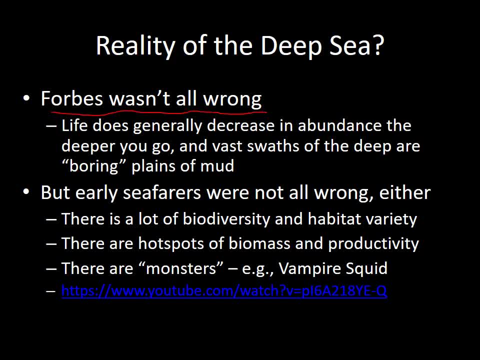 So Forbes wasn't wrong about the fact that life generally decreases in abundance the deeper you go and that a lot of parts of the deep sea are relatively devoid of abundant life. So they're these sort of boring plains of mud that we call the abyssal plains. 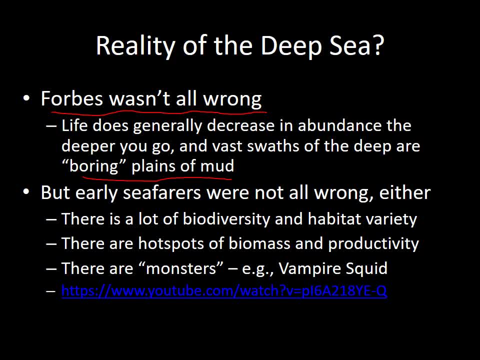 But those early seafarers who imagined monsters filling the deep sea were not entirely wrong either, because there are a lot of really cool organisms in the deep sea. There's a high biodiversity, many species, and we're discovering more all the time. 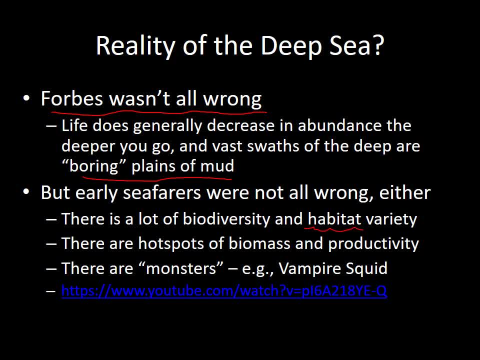 And there is a diversity of habitat. So it's not all boring mud plains. There are deep sea reefs, hydrothermal vents, seamounts and all kinds of interesting things in the deep sea, if you look hard enough. And there are monsters. 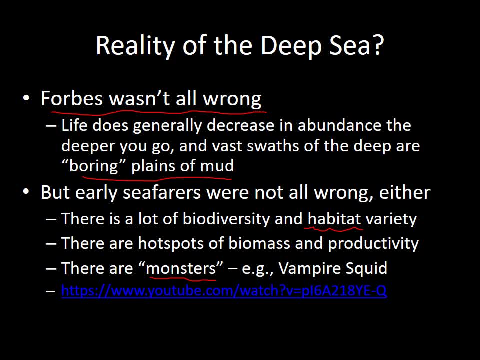 You can click on the YouTube link to see one of the monsters, the vampire squid. If the YouTube link doesn't work, just Google vampire squid and you'll find other cool videos of it. So the way we have learned about the reality of the deep sea. 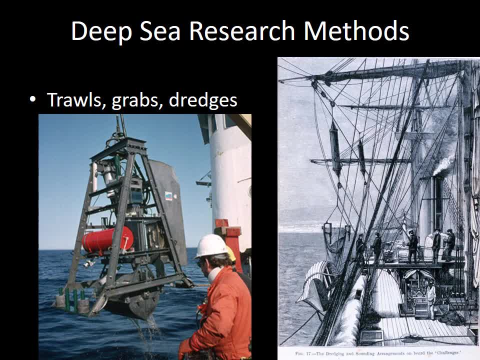 is through a variety of deep sea sampling methods. So we use trawls, nets that are dragged along the bottom. We use grabs, which are sort of clamshell-like samplers that we drop down to the seafloor, and they grab a chunk of the seafloor. 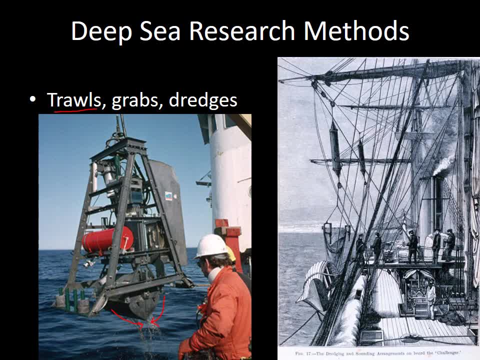 and pull it up in their jaws so that we can examine the seafloor organisms, And then dredges, which are kind of like nets towed over the seafloor, except dredges are made of a rigid structure rather than a flexible net. 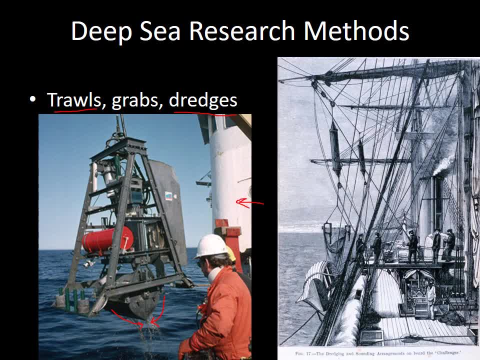 So we use these in modern times, but some of these trawls, grabs and dredges were used in the 19th century on this HMS Challenger vessel- And the HMS Challenger was a British vessel that was one of the first to explore the deep sea. 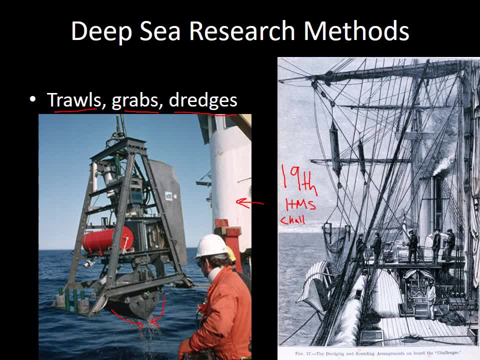 and sample there. So a lot of the classic deep sea organisms that we now imagine, like the anglerfish and the dragonfish and the deep sea goldfish, the gulper eel, those kind of things were discovered for the first time on this HMS Challenger expedition. 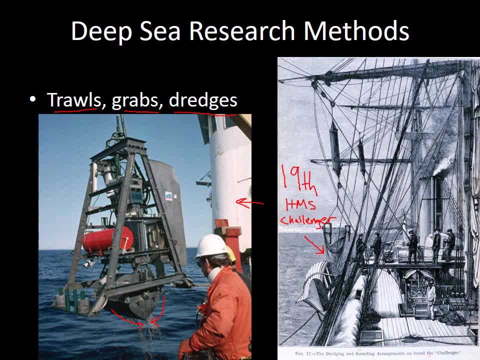 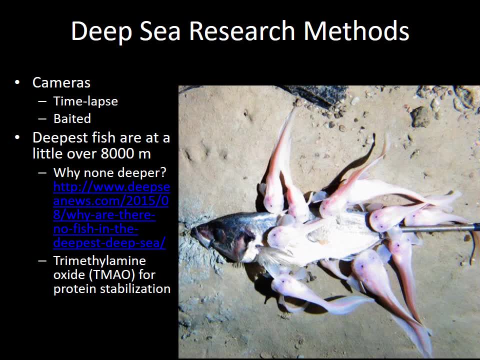 and some of those specimens are still stored in the museums of the world. So this was a very important expedition. We have some methods now that they didn't have back in the 19th century, when people first started sampling the deep sea. For example, we have cameras. 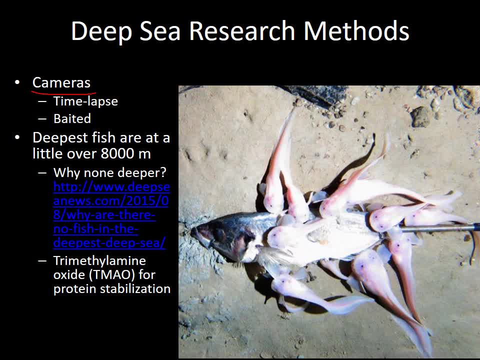 that we can lower to the deep sea, And sometimes you have to be very patient to see the action in the deep sea. We have these time lapse cameras that will take one picture every certain number of minutes or hours or days and can see things that are slowly changing. 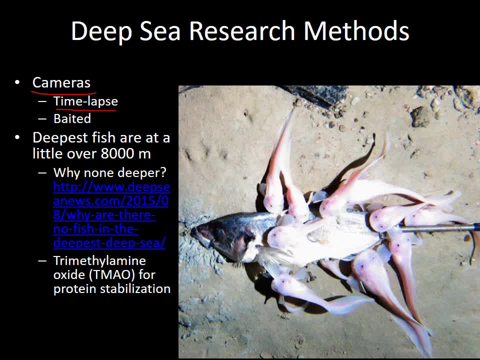 or happening over time. Sometimes, to concentrate life, we will bait the cameras, And in this picture here, what we're seeing is a picture from a baited camera. So this fish here is a surface dwelling fish that was put on a stick and lowered with the camera. 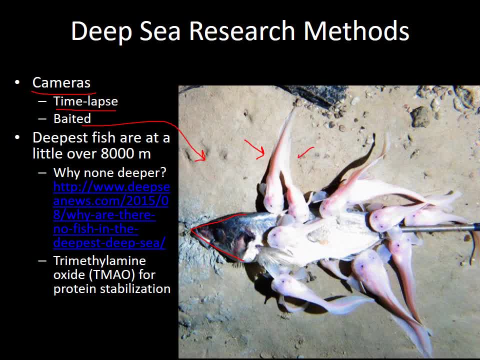 But these fish here are snail fishes which live very deep in the sea, a little over 8,000 meters at the maximum depth, And these seem to be the deepest living fish in the ocean. So 8,000 meters more or less is a physical limit, it seems. 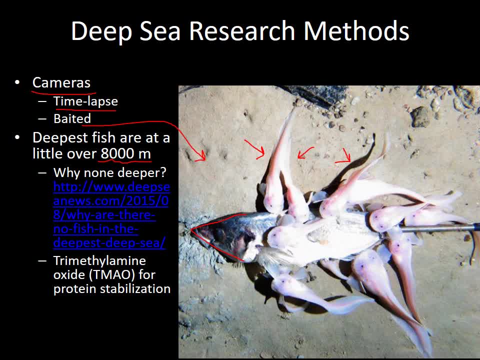 for vertebrate life And there's an interesting article, if you follow this link, on what the sort of physiological factors are that prevent fish from surviving any deeper in the ocean than 8,000 meters, even though some invertebrates can survive down there. 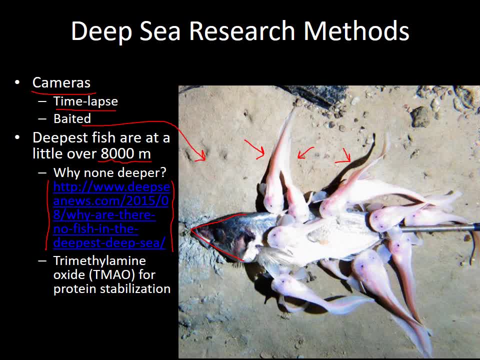 So the CliffsNotes version is that there's this problem that fish have where their proteins are being disrupted by high pressure water molecules pushing in between the cracks and folds of the proteins and preventing the proteins from working right. So one of the adaptations that the fish have. 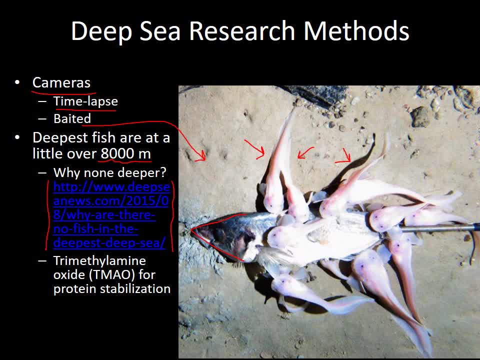 in the deep sea to prevent water from sort of messing up their proteins is they have high concentrations of this compound called TMAO in their cells And the TMAO keeps the water molecules from getting into the cracks and crevices of the proteins. 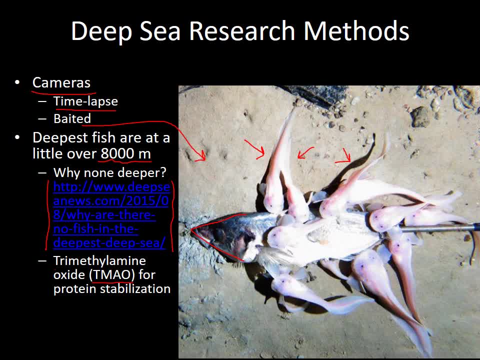 and allows the proteins to function. The only thing is that there's a limit on how much TMAO you can have in your cell before the cell becomes so hyperosmotic that it is absorbing that- the osmoregulatory balance between the cells and the surrounding water. 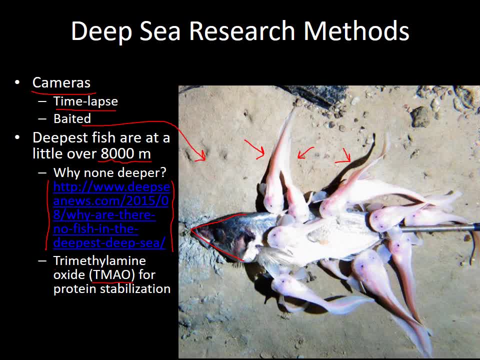 is untenable and the organisms can't survive. So I'm not quite sure how invertebrates get around this, but I think they have some other biochemical mechanism for dealing with the problem of high water pressure and protein folding differences. But this TMAO thing is the way. 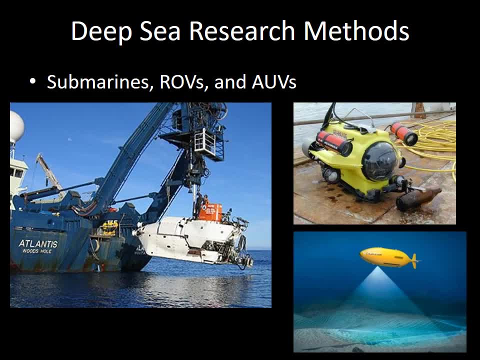 that vertebrates do it All right. Another method that we have for studying the deep sea, besides lowering cameras down there, is lowering submarines down there. So this submarine is called the Alvin. It's a famous deep sea submarine that was the one that discovered 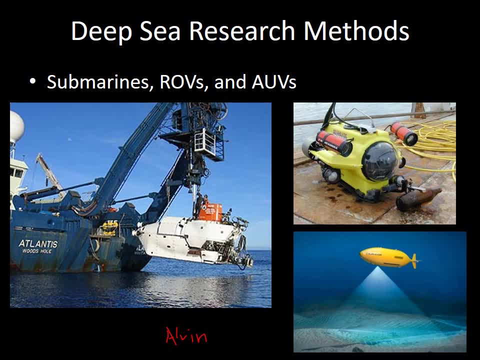 hydrothermal vents for the first time on the Mid-Atlantic Ridge, And that is a submarine. And then an ROV stands for remotely operated vehicle And there's a remotely operated vehicle And AUV stands for autonomous underwater vehicle which is not operated by remote control. 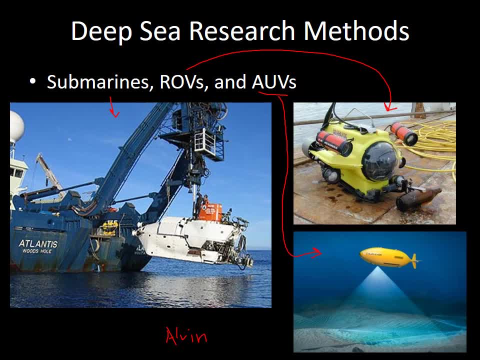 It's a robot that has its own robot brain And you just program it and send it down there and it will operate itself to survey the ocean. So there's most of the deep sea exploration that we do now is not with submarines, because they're so expensive. 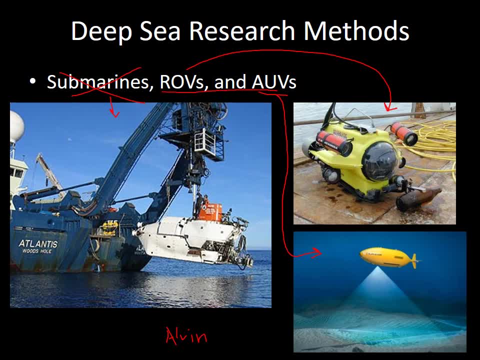 and it's dangerous for the submarine pilots, But it's with ROVs and AUVs that are more affordable and allow us to go down there longer and survey more of the deep sea. All right, So let's talk about the ecology of the deep sea. 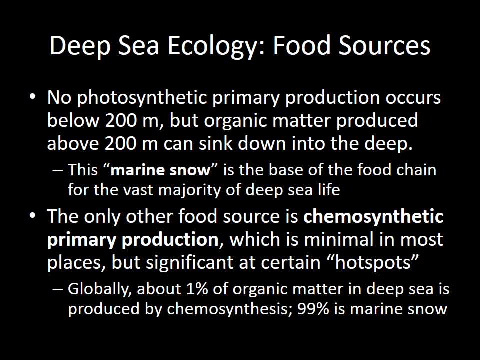 And the fundamental limiting factor for life in the deep sea is the availability of food. Because there is no photosynthetic primary production in the deep sea, All the organic matter in the deep sea, for the most part anyways, had to be produced in the shallow ocean. 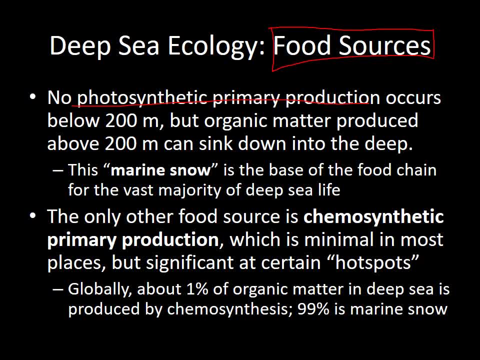 and then sink down into the deep. So they call that sinking of organic matter from the surface down into the deep marine snow, because it's these flakes and flecks of organic matter, Some of them small like individual phytoplankton cells, Some of them larger, like dead fish. 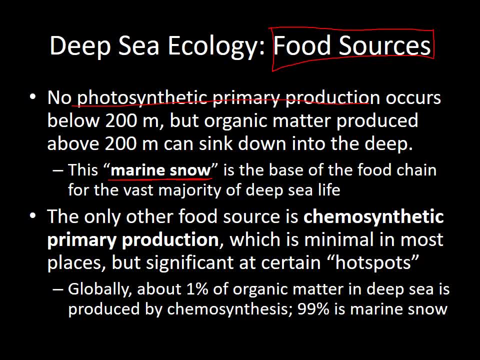 As those sink into the deep sea. that is what supplies food to the deep sea. There is one other food source to the deep sea and that is chemosynthetic primary production, where there's primary production created by microbes that feed on energy rich chemicals. 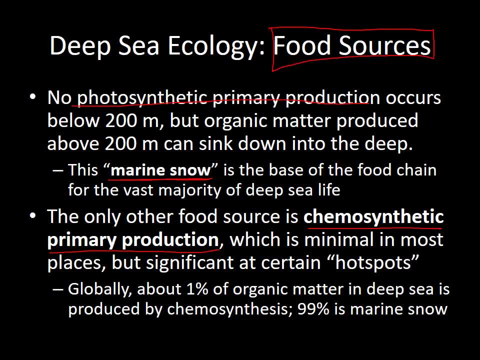 And there's a lot of chemosynthetic primary production in certain hotspots in the deep sea like cold seeps and hydrothermal vents. But overall only a tiny proportion of the organic matter in the deep sea: 1% or less of the organic matter deep sea. 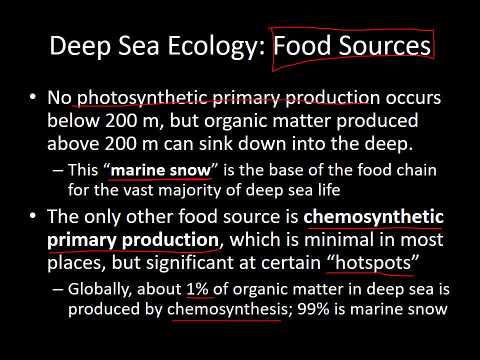 is produced in the deep sea by chemosynthesis. So really the vast majority of the foods to the deep sea on a global scale originates in the shallow waters and snows down to the deep sea. So chemosynthesis is very interesting. it's very cool. 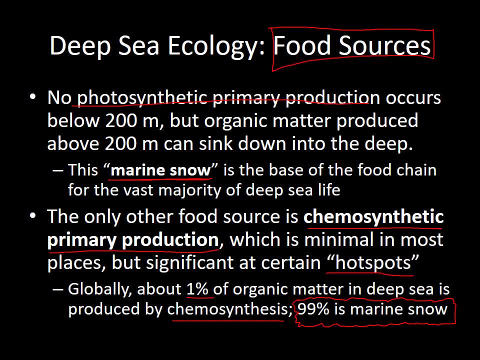 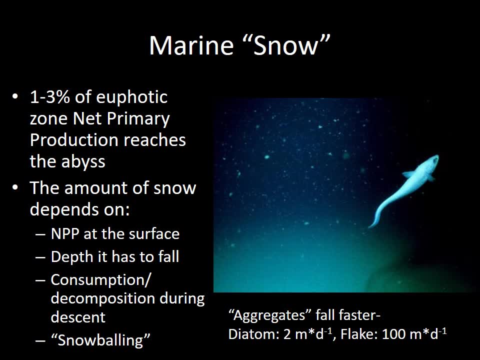 and it's locally a big source of production. But if you look on the overall scale, most of the food in the deep sea came from the surface Alright. so let's talk about that marine snow. Very little of the marine snow, of the primary production. 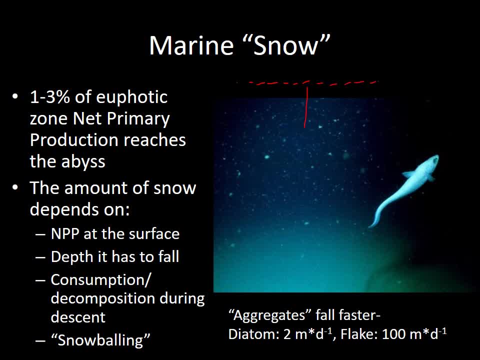 that's happening at the surface is actually making it all the way down to the deep sea. So here's the surface and there's a lot of phytoplankton there that are producing, and so you know, you've got 100% of the primary production. 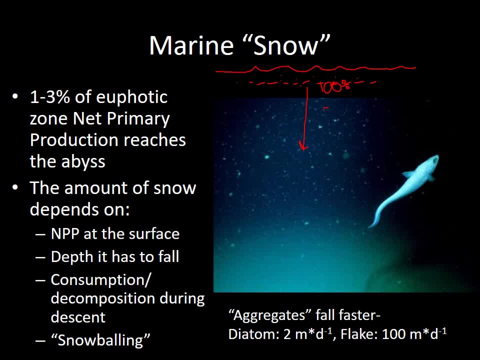 when you're in the surface waters, but as you go down deeper, there's less. as you go down deeper, there's less. as you go. by the time you get to the bottom of the deep sea, you might only have 1-3% of that primary production left. 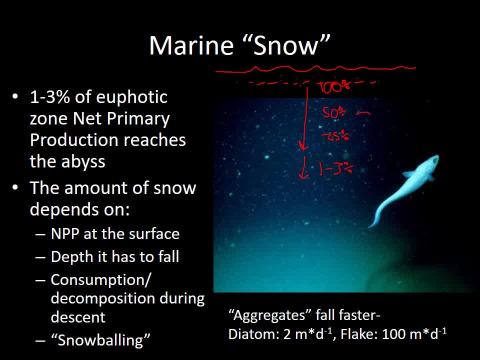 because a lot of it gets eaten or decomposed on the way down and it doesn't make it all the way to the bottom. So the consumption or decomposition during the descent of the marine snow is very, very significant in determining how much of it, if any, is left. 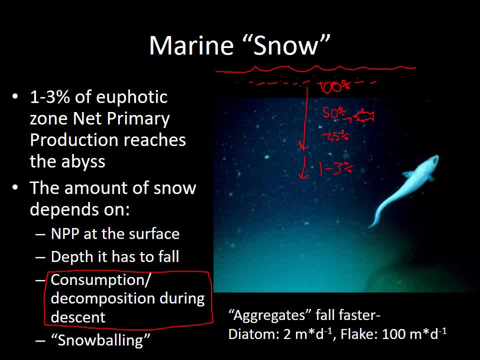 at the bottom of the ocean. So also the depth that it has to fall is important. So if you're really deep in the ocean you're not getting as much marine snow as if you're only kind of deep in the ocean. Also, the amount of productivity. 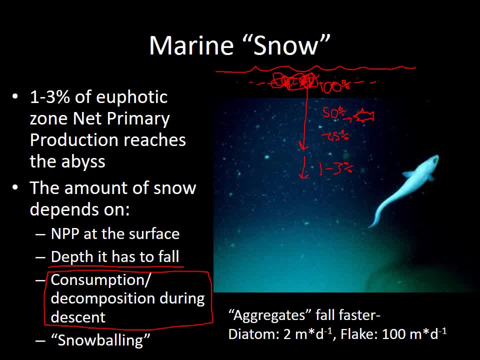 at the surface influences how much gets to the bottom. So if there's a lot of primary production at the surface, then even though only 1% is getting to the bottom, it's 1% of a lot, which is more than 1% of a small amount. 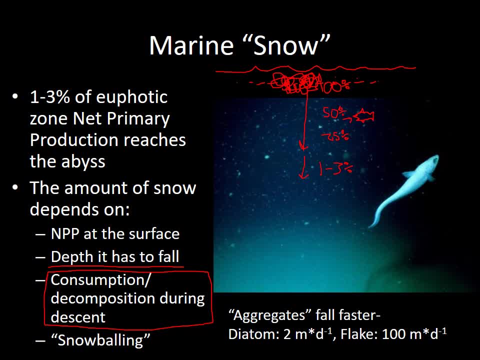 Another thing that can affect how much, what percentage of the production reaches the deep sea is how fast it falls. and how fast it falls is influenced by this thing called snowballing. So an individual diatom cell falls very slowly, But if you have a clump, 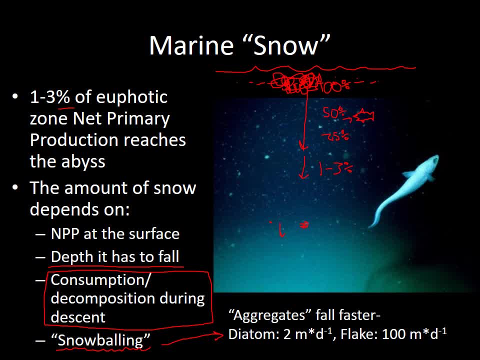 of lots of diatom cells and other debris and slime. it makes this larger particle with a lower surface area to volume ratio and that large aggregate will fall much faster. as much as a hundred meters a day versus two meters a day, So at a hundred meters a day. 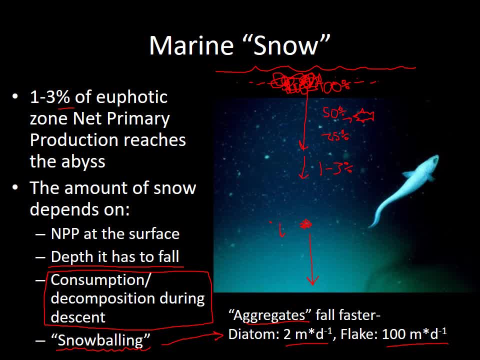 it would take about 38 days to fall to 3,800 meters at the deep sea, which is over a month. So even a clump takes a long time to get to the deep sea, But a single diatom cell would take a very long time. 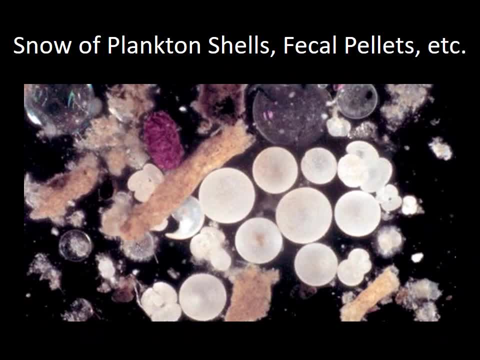 at just two meters per day. All right, so what does marine snow look like up close? It looks like this. So here you can see a mix of plants, Plankton, shells and skeletons. like these are dead diatoms And these are fecal pellets. 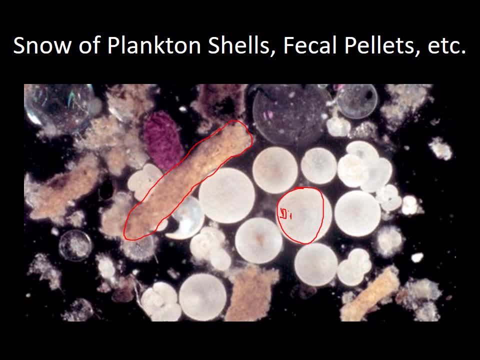 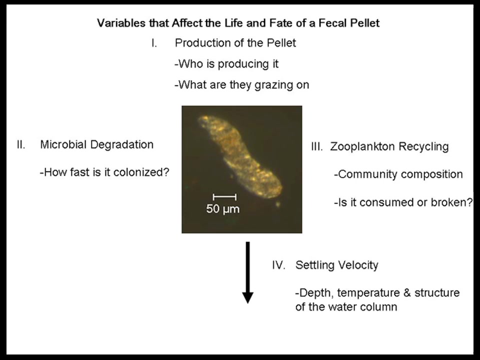 of zooplankton. So this is a piece of poop And there are various kinds of fecal pellets because everybody poops differently and some types of organisms make different shapes of fecal pellets. This is a diatom, So these fecal pellets- 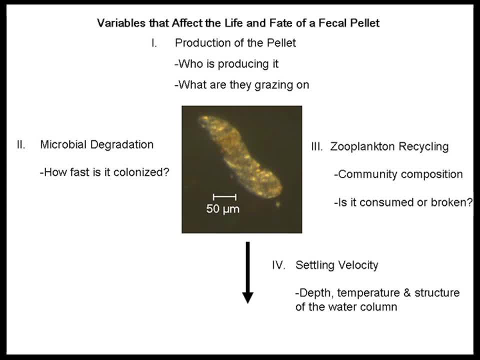 turn out to be very important, because a fecal pellet, particularly if it's a big and densely packed one, will fall a lot faster than a dead algal cell. So if there are organisms that are grazing on phytoplankton in the surface waters, 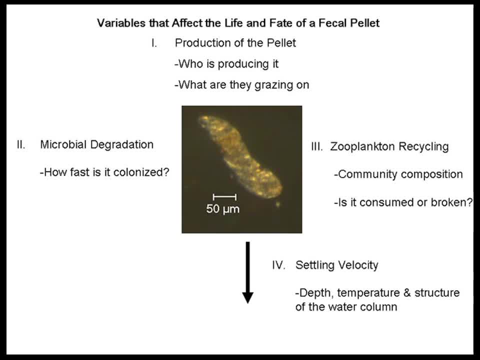 and packing that phytoplankton into big solid turds, then that means that a lot more organic matter is being exported to the deep sea than if you don't have those grazers that are repackaging the stuff as turds. So there are scientists. 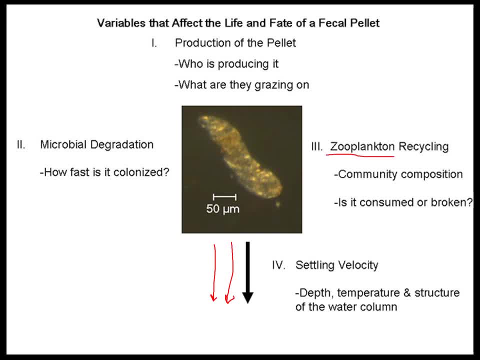 who spend their entire lives studying these zooplankton communities and how much phytoplankton they eat. how well do they pack it into turds? what's the difference between the fecal pellets of one species of phytoplankton versus another species? 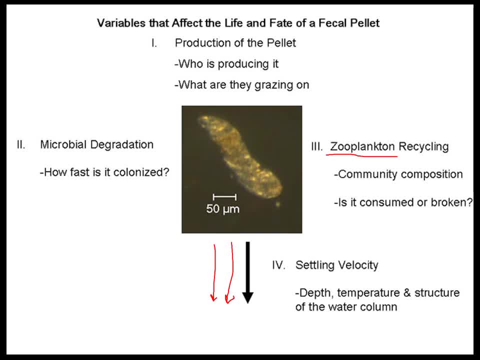 of phytoplankton. how much are these fecal pellets degraded by bacteria that feed on them as they're falling? So there's all kinds of interesting processes that determine what percentage of the surface primary production actually reaches the deep sea, And this has huge implications. 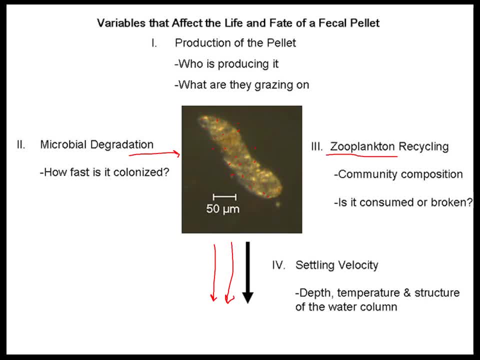 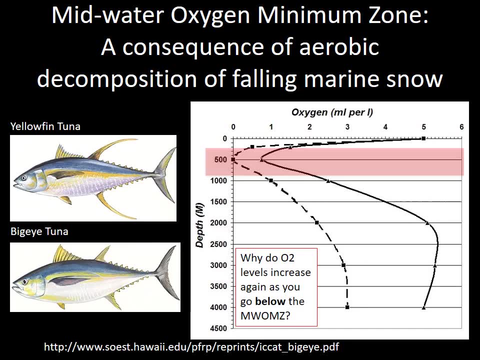 for how many fish there can be in the deep sea and things like that, because it's all dependent on how much of this surface primary production is actually making it down to the bottom. All right, so another consequence of the marine snow processes is that there is this zone. 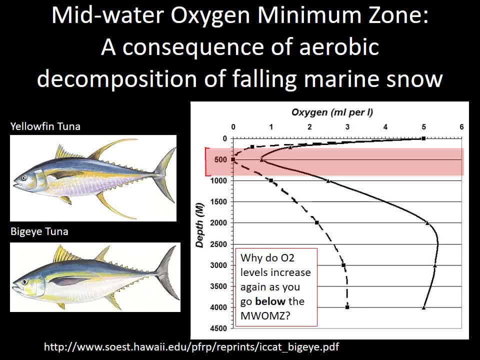 in the moderately deep sea, in what we call the mesopelagic zone, where there is very low oxygen levels. It varies from place to place in the world, but in some places it almost becomes anoxic in that moderately deep sea area. So that can be a really tough place. 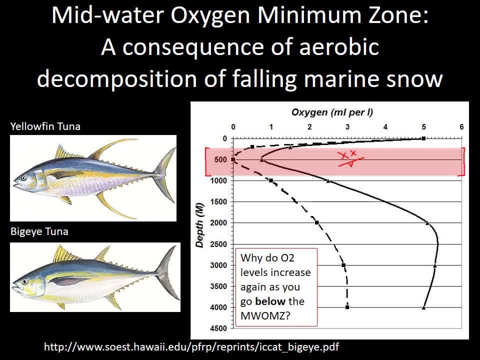 for a lot of organisms to survive. So in the surface waters you have a lot of oxygen And in the really deep waters you have a lot of oxygen, But in this midwater oxygen minimum zone you do not have much oxygen. 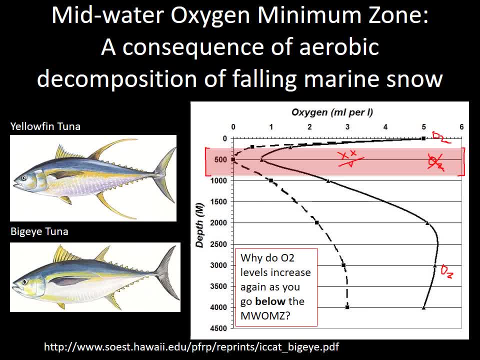 So it's a consequence of the decomposition of falling marine snow. So there's a lot of production of organic matter in the surface waters, photosynthetic production, and there's also a lot of exchange of oxygen between the atmosphere and the ocean in the surface waters. 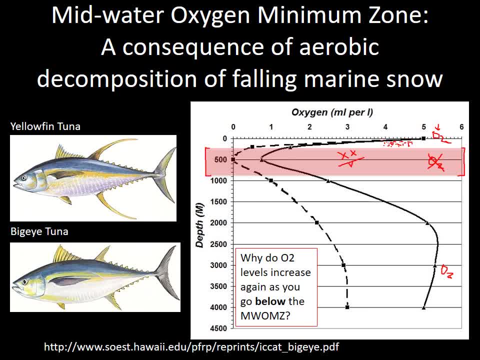 So that's why there's a lot of oxygen in the surface waters. But when you get a little bit deeper, as that organic matter sinks, then there's no longer any primary production, So there's no longer any creation of oxygen and you're also further from the surface. 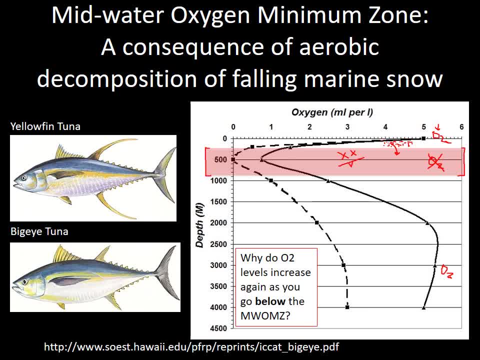 so you don't have any diffusion of oxygen from the surface into those waters, And so there's still a lot of organic matter there. it's just none of it's being produced, it's only being decomposed, And so all this decomposition is what depletes oxygen levels. 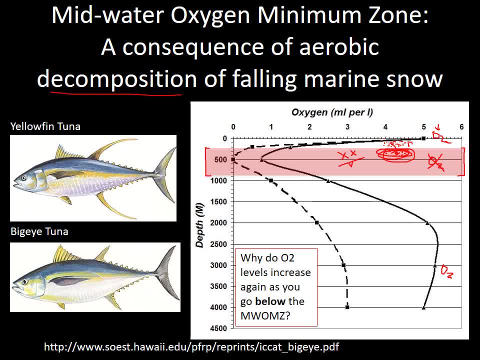 in this area that's sort of just below the photic zone. So there's a big drawdown of oxygen when you're right below the zone of primary production. And so the question I have here is: why do oxygen levels increase? Why do oxygen levels increase again? 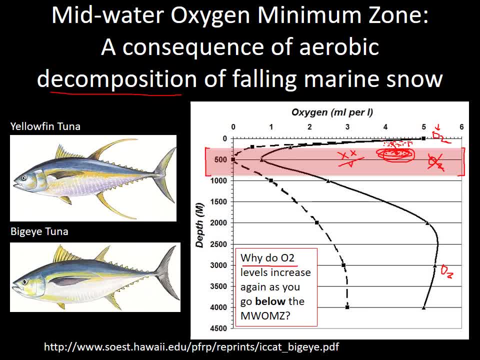 when you get below the midwater oxygen minimum zone. So what's the source of oxygen to the deep sea? It seems like if oxygen was getting lower as you went deeper, it would just keep getting lower and lower all the way to the bottom. 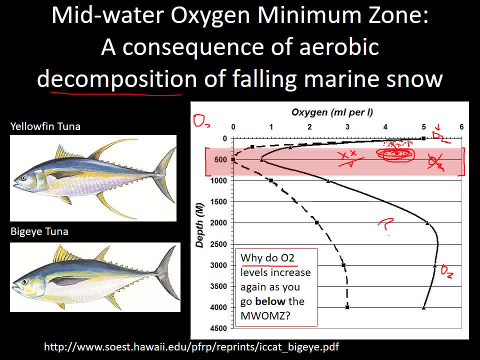 Well, the secret is that oxygen is getting into the deep sea waters in the parts of the world where deep sea waters form, like the Arctic and Antarctic, and then those waters spread through the rest of the deep sea and retain their oxygen. This is a very large volume of water. 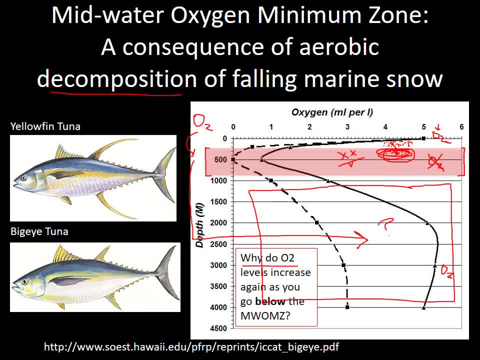 and the life here is sparse because there's not a lot of organic matter. So even though it might be thousands of years since this water was, at the surface, exposed to oxygen, it still has the load of oxygen in it that it had when it formed in the Arctic or Antarctic. 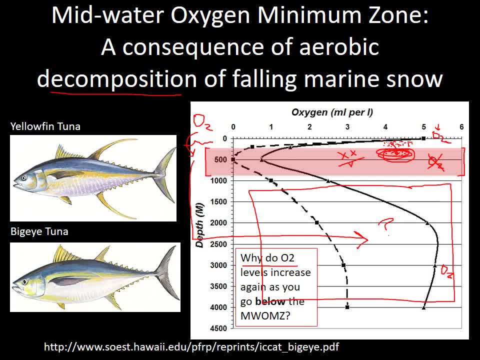 and that's why the very deep sea waters still have oxygen. There's just not enough decomposition happening there to fully deplete them of oxygen before new water is brought in. I hope that makes sense. I should say that there are some parts of the ocean. 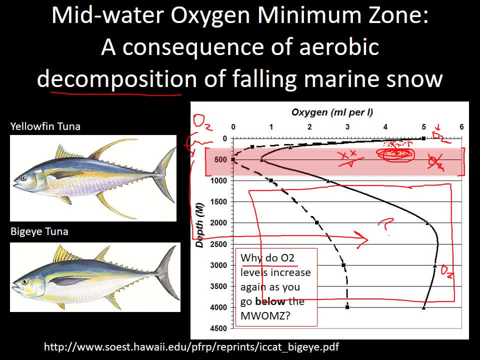 where, because they're cut off from this exchange of oxygen in by the global thermohaline circulation, they don't have oxygen in the deep sea, So isolated chunks of the deep sea, like the Black Sea, which is cut off from this deep water circulation. 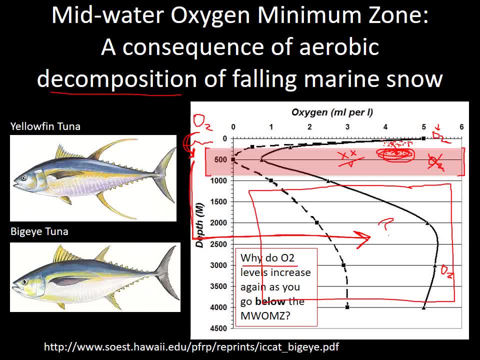 it actually has zero oxygen in the deep, So it depends on where you are in the deep sea whether you are getting this oxygen that's supplied by the cold water currents from the Arctic or not. Okay, so let me clear the writing here. 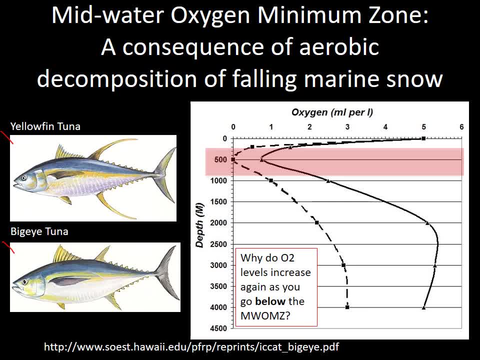 and I want to talk about this. I want to talk about these two tuna fish, the yellowfin tuna and the bigeye tuna. They're both in the same genus and they look very similar. They both look like tuna and they have yellow fins. 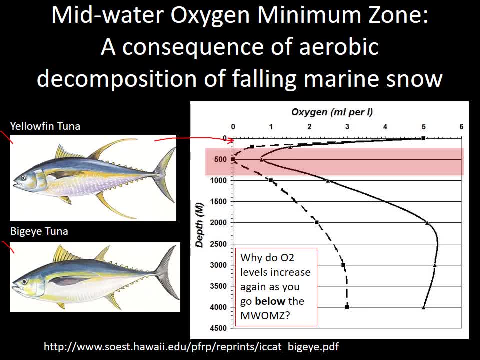 but they're physiologically very different, because the yellowfin tuna is adapted to living in the brightly lit waters of the euphotic zone and the bigeye tuna is adapted to making forays between the surface and the midwater oxygen minimum zone. 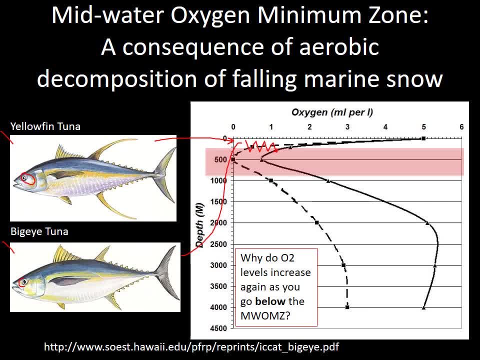 So one of the differences between the fish and the fish is in their eyes. So the yellowfin tuna has eye pigments that work well at detecting fast movement in bright light, but they don't work so well in dim light. And the bigeye tuna 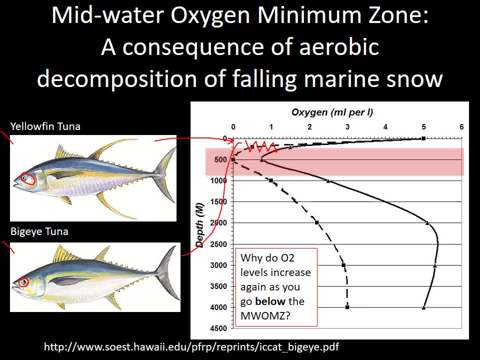 its eyes are not so able to detect fast movement, but they have pigment and light-sensing cells in them that are able to detect slow movement in dim light. so it can feed on slow-moving prey in the dim, dark waters in the midwater oxygen minimum zone. 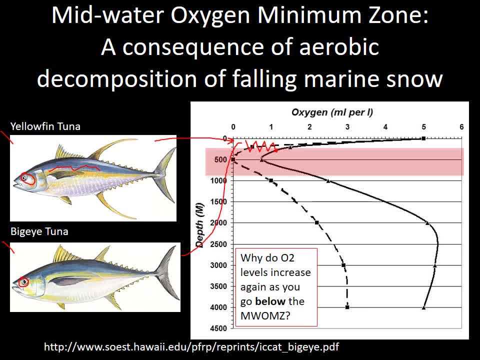 There are also differences in the blood chemistry of the fishes, So this is their blood. The blood chemistry of the yellowfin tuna is adapted for the high oxygen content surface waters and it's able to absorb oxygen where oxygen is abundant and quickly offload oxygen into the tissues. 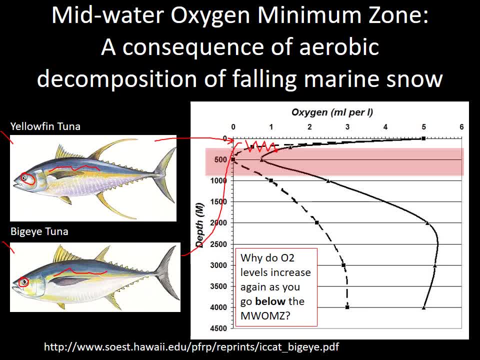 as the tissues become slightly depleted in oxygen and that helps it sort of swim fast and do aerobic exercise in the surface waters. So the bigeye tuna, its blood hangs on to oxygen more strongly, so it doesn't dump off its oxygen into the tissues as easily. 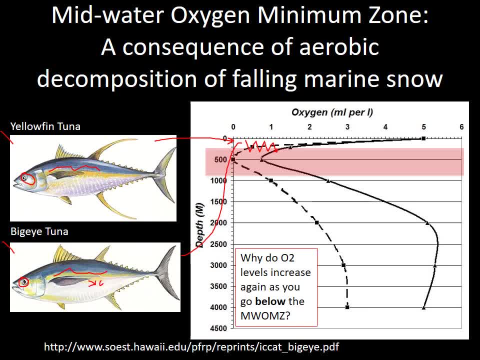 and that means that it can hold on to oxygen a little more and only deliver it to the oxygen to its tissues when its tissues really have a demand for oxygen, and that allows it to keep its tissues supplied with oxygen when it's making these forays into the deep ocean. 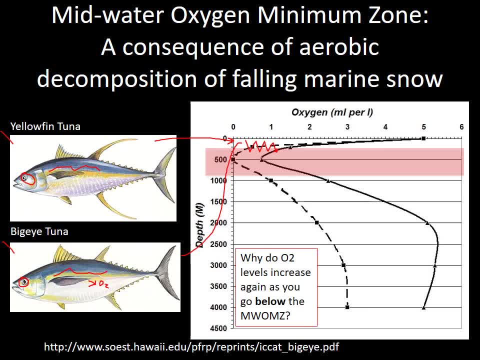 The other thing that's different, besides the chemistry of the blood of the fish, is the pattern of circulation of the blood of the fish. The bigeye tuna has what they call countercurrent circulation of its blood, which means it's able to keep its core temperature warmer. 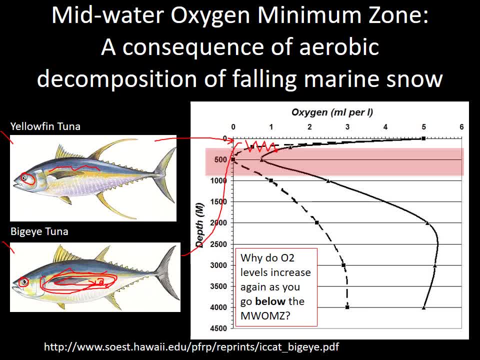 through its blood circulation pattern and that allows it to keep a core temperature that's warm when it makes these forays into the deep water to feed on the invertebrates, like squids and things like that, that live at the edges of the midwater oxygen minimum zone. 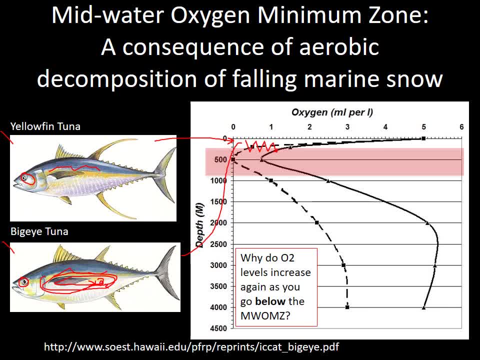 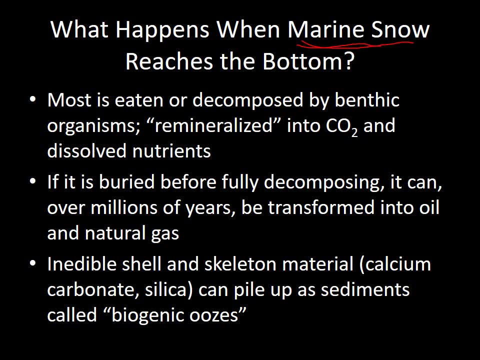 and the yellowfin tuna doesn't have any specialized circulation pattern like that. So same genus, but evolution has given them really different adaptations for the surface waters versus periodically going. Alright, so back to marine snow. What happens when marine snow reaches the bottom? 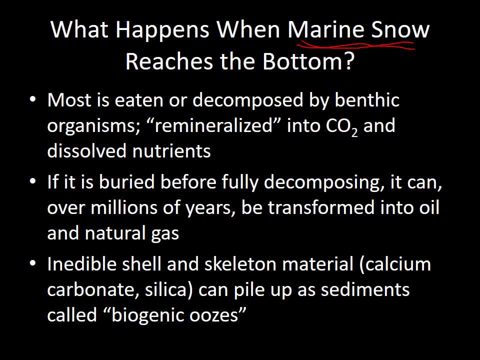 So, first off, most doesn't reach the bottom. It's eaten or decomposed on the way down. but once it does reach the bottom it can be used by benthic organisms and those benthic organisms will break it down and the breakdown process of organic matter. 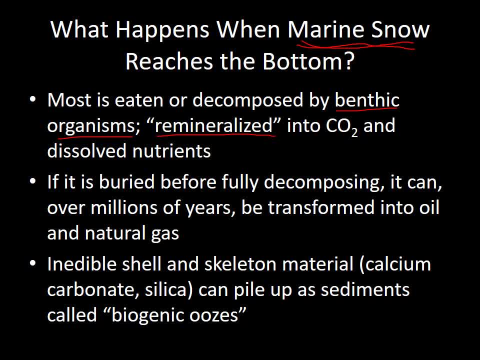 is called remineralization, because you're taking the organic matter and turning it back into the so-called mineral forms of matter, the small, simple molecules like carbon dioxide and dissolved nutrients. So most of that organic matter is basically disintegrated or remineralized, producing carbon dioxide and dissolved nutrients. 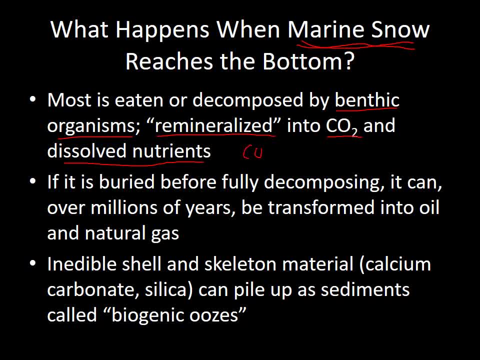 That's one of the reasons that the deep sea is high in CO2 and high in nutrients like nitrates and phosphates. So because all the remineralization of organic matter that's happening on the way down and on the deep sea floor. 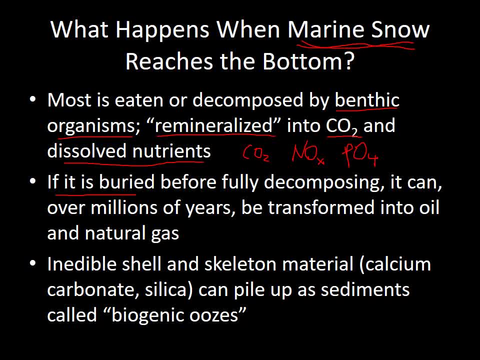 But some of the organic matter, if it's buried before fully decomposing it, can be transformed into oil and natural gas. So deep sea sediments and the organic matter in them, if it's not fully decomposed and it's buried, it will transform into oil and natural gas. 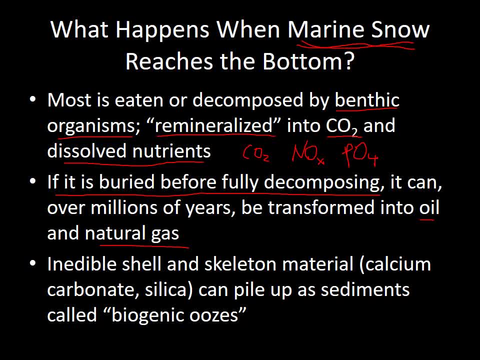 over millions of years. So the oil and natural gas- methane is another name for natural gas- that we sort of harvest from the deep sea through drilling, that's actually derived from the remains of ancient marine organisms that perished and were sort of preserved and transformed into oil underneath the sea floor. 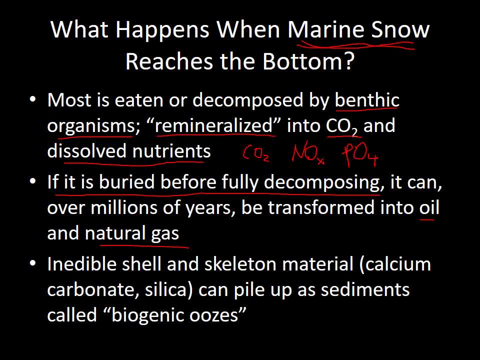 So living things are made largely of organic compounds, but there's also these minerals that some marine organisms have in them, so they'll have calcium carbonate or silica if they're shelled organisms. and those minerals don't decompose, so they can pile up as sediments. 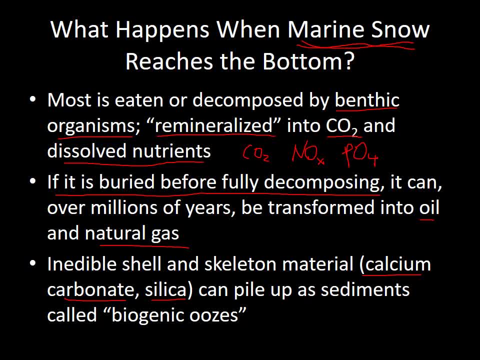 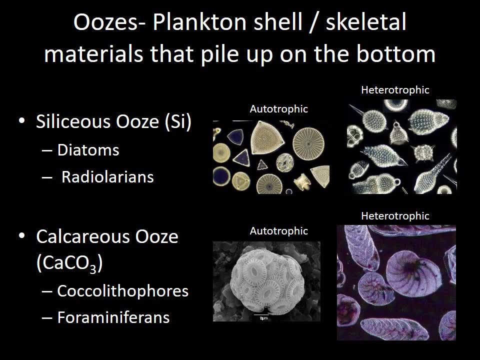 so basically the shells and skeletons of plankton and other marine organisms pile up on the bottom and create these sediments called biogenic oozes. So what kind of biogenic ooze you have on the bottom depends on what kinds of shells and skeletons of organisms. 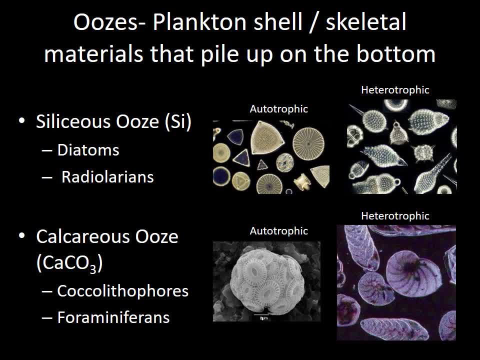 are piling up on the bottom there and it's related a lot to what's going on at the surface. So if there's a lot of diatoms at the surface, then their remains will pile up on the bottom and create siliceous ooze. 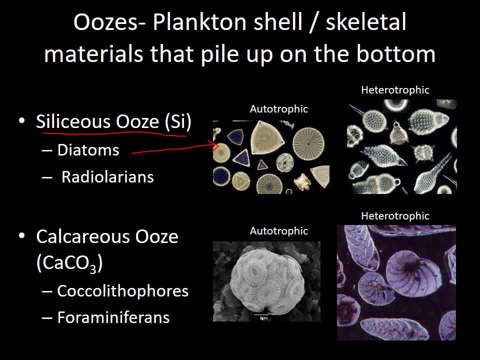 because, remember, diatoms have silica shells. There's some types of heterotrophic plankton that also have glass shells. like radiolarians are heterotrophic protists that have glass shells, and their shells can pile up on the bottom and create siliceous ooze as well. 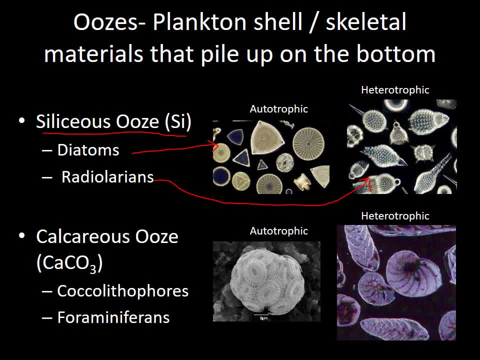 Calcareous ooze is ooze made of calcium carbonate shells, so coccolithophores are an autotrophic protist- type of phytoplankton that has calcium carbonate shells that can pile up into calcareous ooze. Foraminiferins are heterotrophic protists. 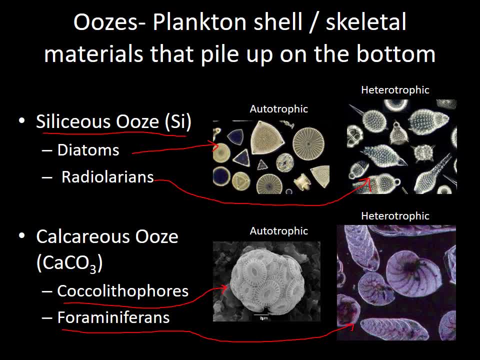 and they have calcium carbonate shells that also pile up on the bottom and create calcium carbonate oozes. One additional factor that affects whether or not calcium carbonate piles up on the bottom is how deep you are and how acidic the deep sea is, because the calcareous ooze. 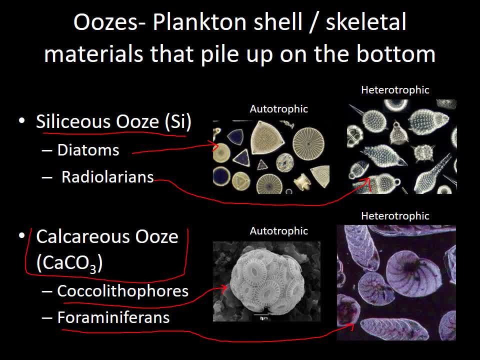 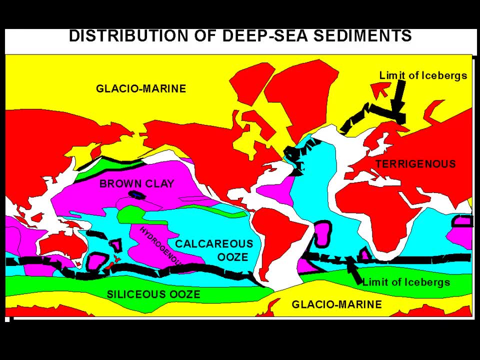 can actually dissolve away and not build up, depending on what the pH and pressure conditions are of the deep sea. We'll talk more about that later Because of these differences in the depth of the ocean and how much primary production there is in the surface waters. 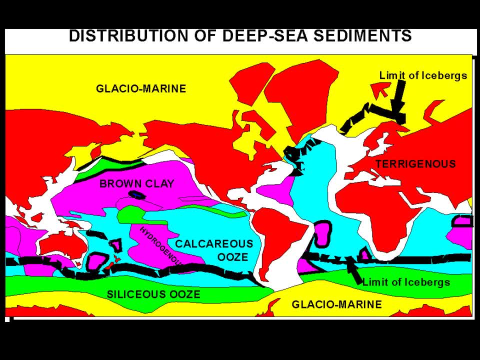 and whether it's diatoms or coccolithophores, what other forms of sediment are reaching the bottom, like if it's gravel on the bottoms of icebergs or dust blown by the wind? Because there's these different sediment sources to different parts of the deep sea. 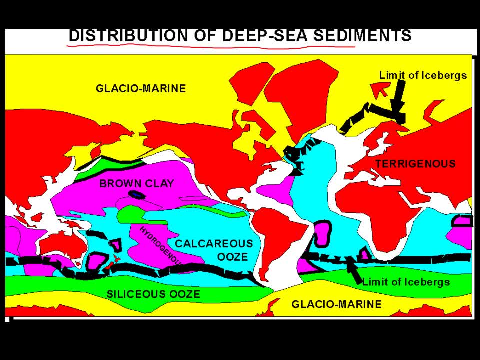 you have this distribution of deep sea sediments that varies from place to place, Like in the waters of the southern ocean, you have a lot of siliceous ooze because there's a lot of diatom production there. But if you get further south, 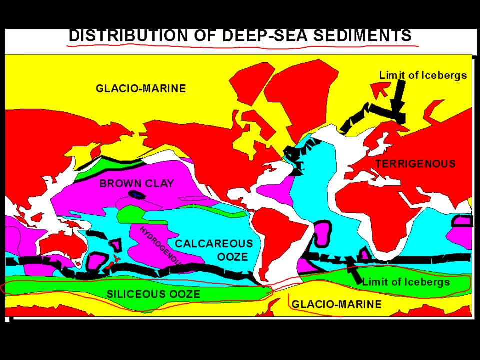 you have glaciomarine sediments, which is where the seafloor is, largely rocks and sand and mud that was scraped off the land by glaciers and then, when the glaciers melted, it dumped that mud down there. So where you are in the ocean, wherever you are on the seafloor, 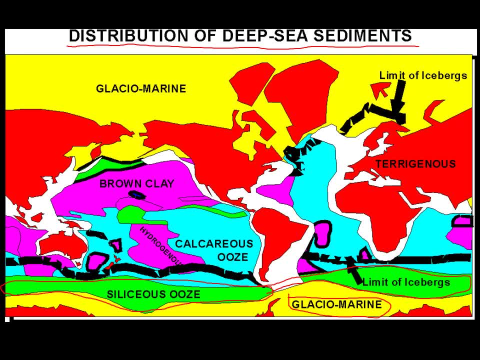 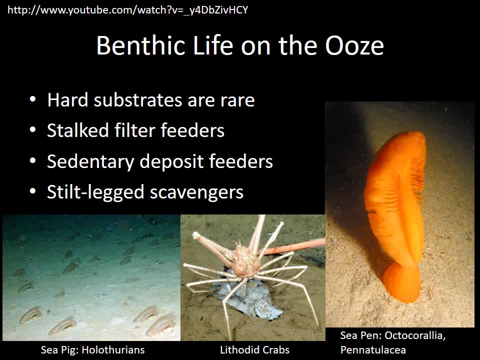 you have different kinds of sediments, depending on what the overlying processes are. Alright, so what's life like down there, on these sedimentary deep sea floors? Well, it's not a place that humans could survive, but it's pretty interesting for some types of marine organisms. 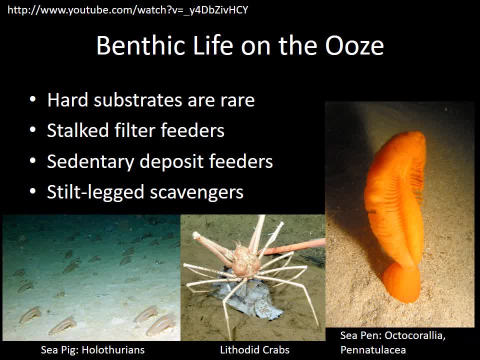 So some hard substrates are rare in the deep sea. There are some places where there's rocky outcroppings, but in a lot of places the millions of years of sediment accumulation have covered the deep sea floor in a very, very thick layer of mud. 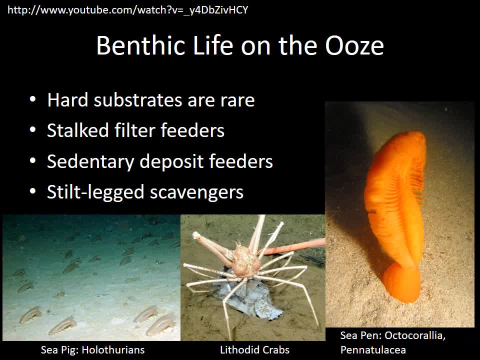 And so you have these organisms like the holothurium, which is another word for sea cucumbers, and this particular type of sea cucumber is called the sea pig, because it's thought to resemble a pig. And if you want to see a funny video on the sea pig, 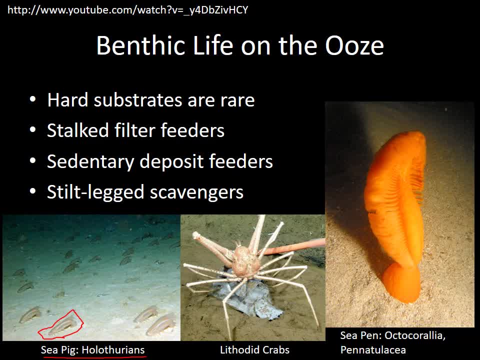 you can look at the YouTube link there. So they're deposit feeders, sedentary deposit feeders. They don't move around very much, but they slowly trundle across the seafloor and they eat the organic matter that they can glean from the sediments. 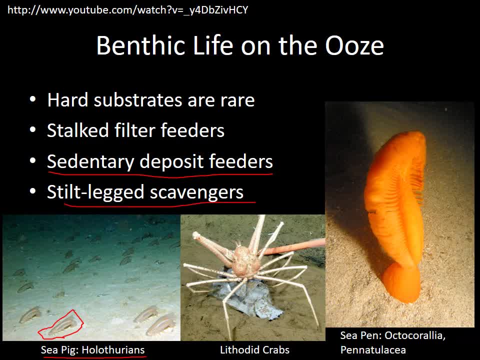 There are some scavengers that walk across the deep sea floor like lithoded crabs, a variety of what we would call spider crabs, that sort of stalk across the deep sea floor and eat what they can And there, although, most sedentary filter feeders. 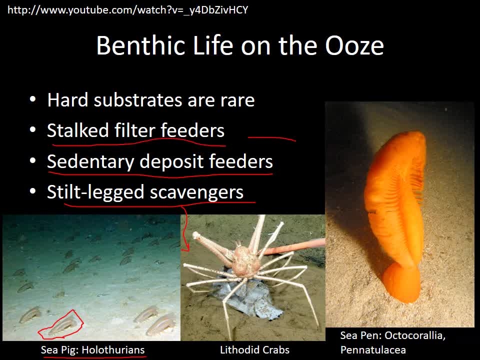 can't attach. there are some stalked filter feeders, like the sea pen, a relative of the soft corals that live in shallow water, that have sort of a stalk that anchors them into the sediment And then they have. they have a bunch of tentacles. 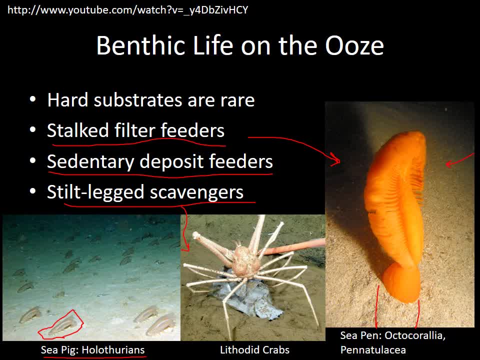 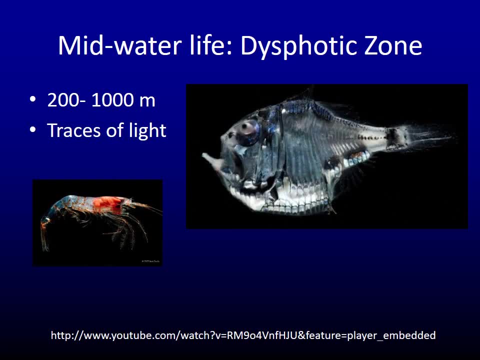 that will catch particles drifting through the currents and that's how they sort of filter, feed and make their living Alright. so, moving up from the seafloor into sort of the mid-central waters of the deep sea, we'll talk about some of the mesopelagic life. 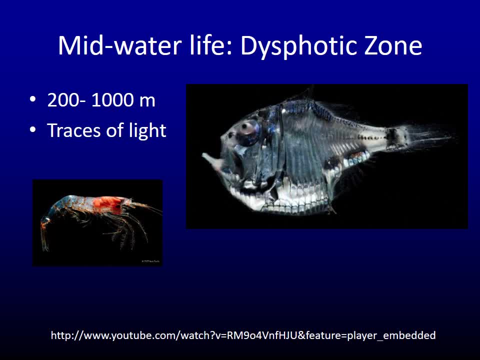 So this is the life of the twilight zone of the deep sea. So we're talking about depths from 200 to 1,000 meters here, where there are traces of light but not enough for photosynthesis. So organisms in this zone may have eyes. 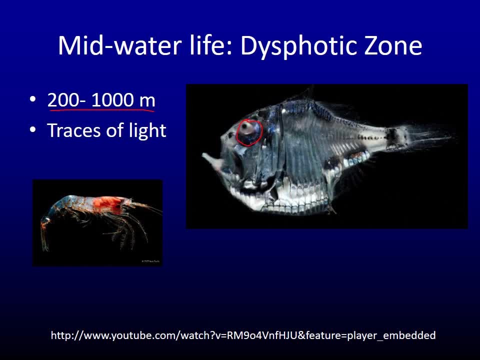 that are pretty good at sensing dim light and looking out for predators or prey, And because seeing and being seen is so important in predator-prey interactions, they have evolved some interesting forms of camouflage. This hatchet fish has special photophores, which are light-producing organs. 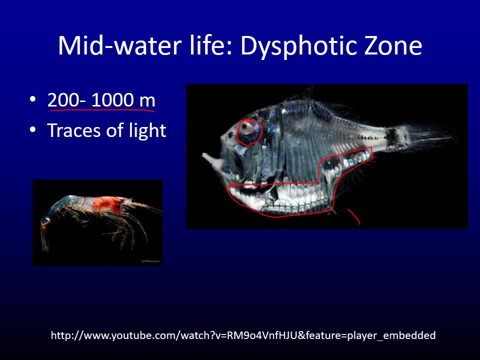 on the underside of its body And they produce a dim glow that is just enough to sort of erase its shadow. So if you are a predatory fish looking for something to eat and you're sort of like looking up at the waters above you, you would be looking for. 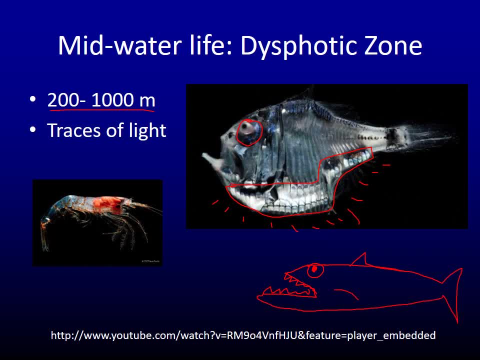 like a silhouette of potential prey. But if you're looking up at the waters above you, if the silhouette is blending in with the exact brightness of the surface, you wouldn't see anything. So you wouldn't see this hatchet fish above and the hatchet fish would escape. 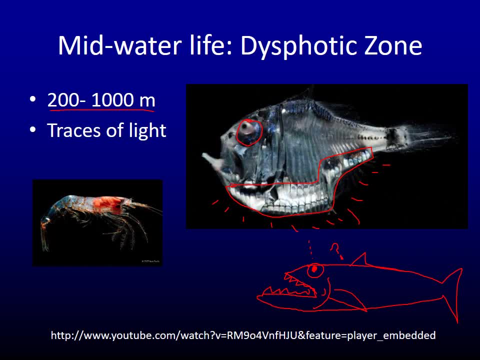 So that's how its special bioluminescence works. Another type of camouflage in the deep sea is to be largely transparent or to have red pigment. So red pigment doesn't seem like it would be good camouflage, because here on the surface of the Earth, 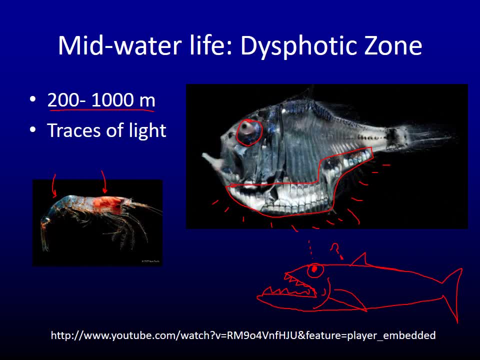 in the bright sunlight we see red very well, But red light doesn't penetrate far in the water, So red actually appears black in the mesopelagic zone, and so it's actually a pretty good form of camouflage. Most organisms can't see red in the deep sea. 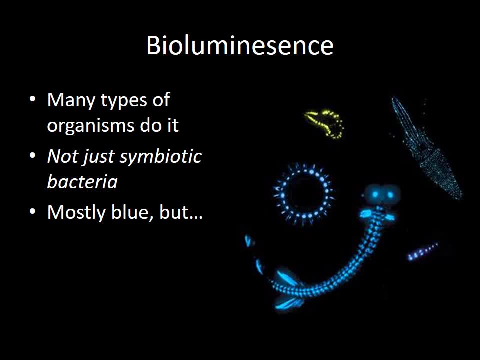 So bioluminescence is not limited to the hatchet fish. There are many, many types of fishes and invertebrates and microorganisms in the deep sea that can make light. So bioluminescence means life-made light. So there's sometimes a false impression. 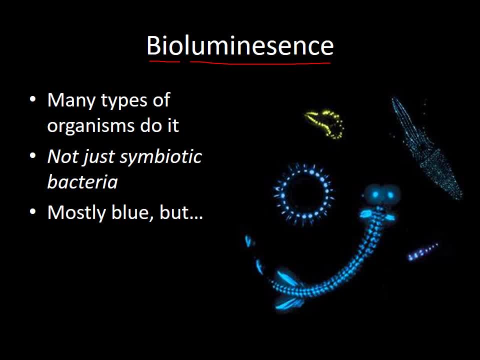 that bioluminescence is all achieved via symbiotic bacteria that create light. but there are actually many different ways that organisms have evolved to make light. So some organisms make light via symbiotics, so symbiotic bacteria and the bacteria make the light. 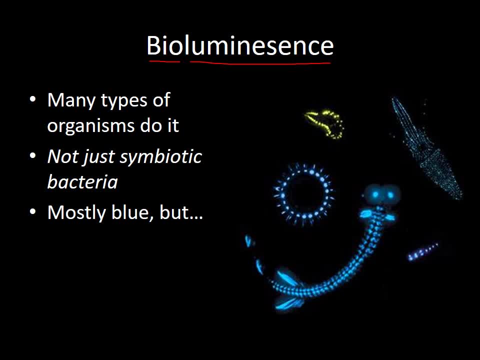 but other organisms. it's their own biomolecules that make the light, So there's a lot of different ways that light is made, And most of the bioluminescent light that's produced in the deep sea is blue. That's because blue penetrates the water the best. 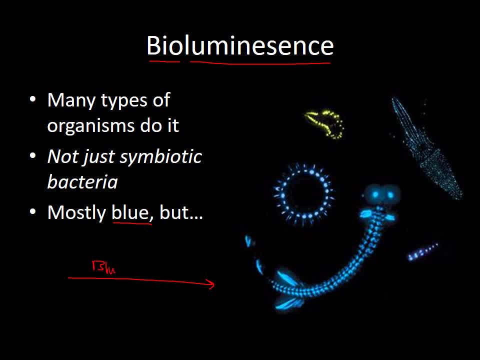 So blue light would go a long ways in the water, whereas red light would not go far in the water. So if you want to see things or be seen over a long distance, you need to make a type of light that will go far. 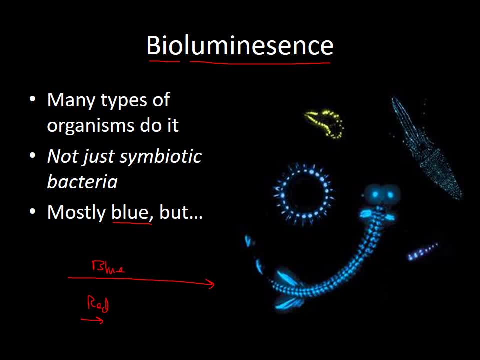 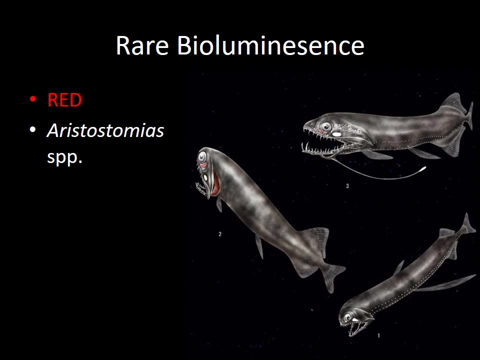 So most of the bioluminescent light is blue, but there are exceptions. There are some organisms that make red light. So this genus of fish, Aristostomias, are predatory deep-sea fishes and they can make red light with special photophores. 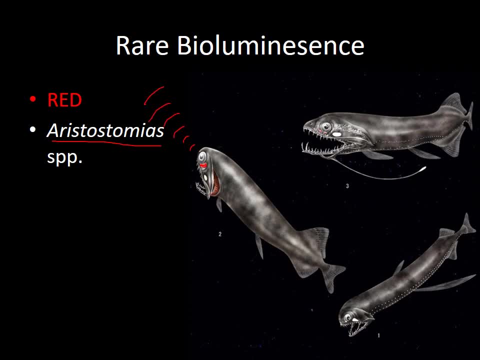 that sort of beam, red light out like red headlights, And so their red headlights are able to illuminate organisms that would otherwise be unseen, organisms that have red pigments, red reflecting pigments- in their bodies. So an organism like this shrimp would be revealed in the red spotlights. 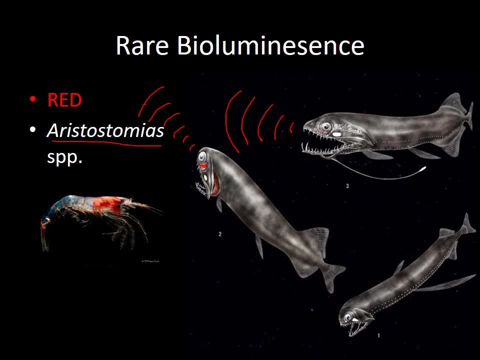 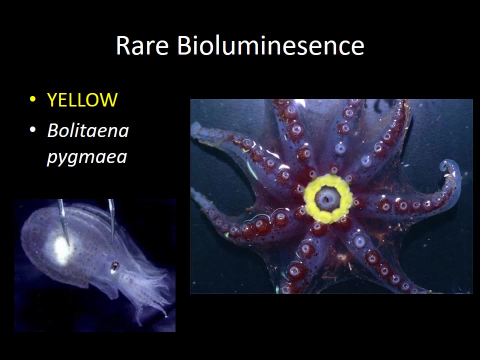 of the Aristostomias And this shrimp. it can't see red light, so it wouldn't even know that it was in the headlights Until it got eaten. All right, I hope that makes sense. Some deep-sea organisms will make yellow bioluminescence. 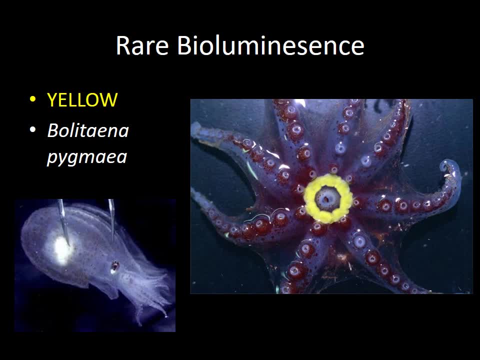 This pygmy squid of the deep-sea, Boletania pygmaea, has a circle of yellow photophores around its mouth, and nobody knows what it's for. So that's just one of the mysteries of the deep sea. All right, so moving into the research. 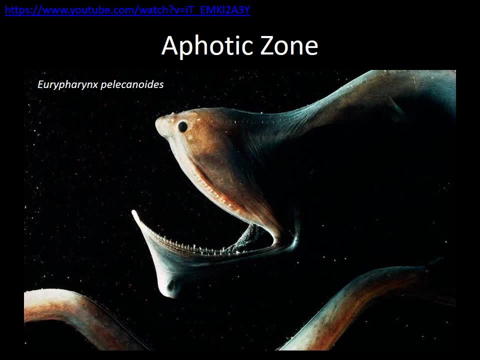 all right, so moving into the really deep waters, there's some very interesting and bizarre creatures there, including the pelican eel, which has a really oversized mouth, with its eyes way up near the front of its head and a mouth that gapes back much further. 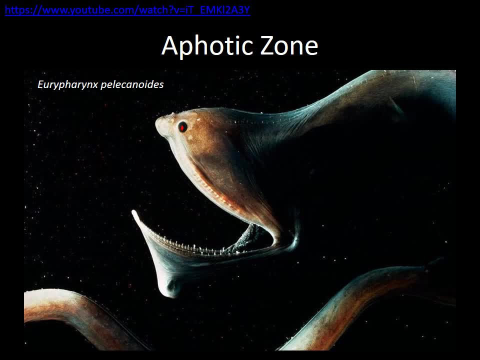 So you would think that this thing eats large prey with that big mouth, but it seems to just gulp smaller prey- that are slow-moving shrimps and things like that. So it has a big mouth, but this particular species doesn't eat inordinately large prey. 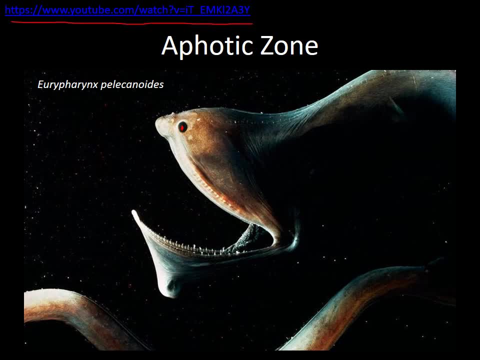 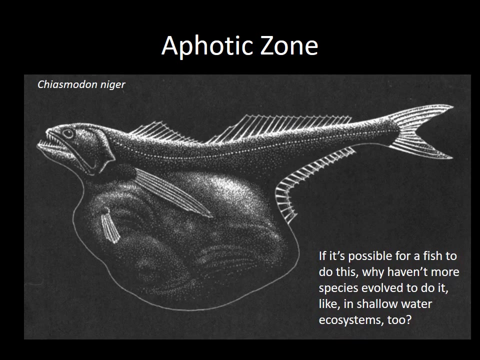 There's a cool video of the pelican eel and we learned some things from this video about how it uses its mouth and expandable throat as a defensive mechanism. So a more fearsome deep-sea organism that does eat very large prey with its unhinging jaw. 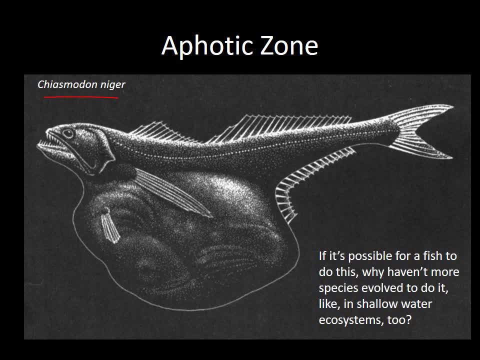 is Chiasmodon nigeri. Chiasmodon nigeri is the black-swallower fish, So this fish is quite small. fortunately, I think it's less than 20 centimeters long, but it's able to eat much larger fish. 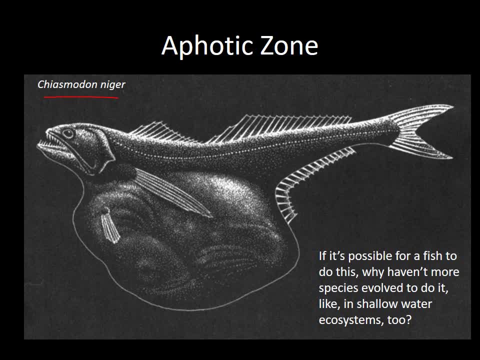 So if it encounters a large fish, instead of being the one that gets eaten, it can be the one that does the eating. So in order to do that, it has a jaw like a snake that unhinges, and it has a flexible, strong stomach. 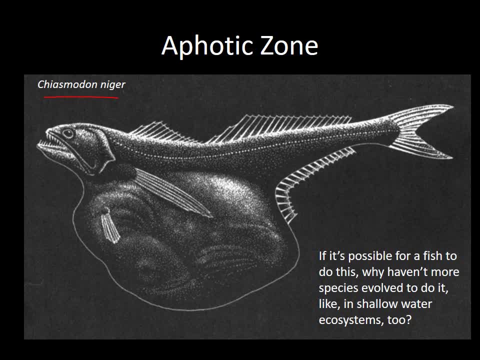 so that it can hold the large prey. So this seems like a genius adaptation and you sort of wonder: if this little fish is able to eat bigger fish, why haven't more species evolved to do that, like in shallow-water ecosystems? Why aren't we worried about small fish? 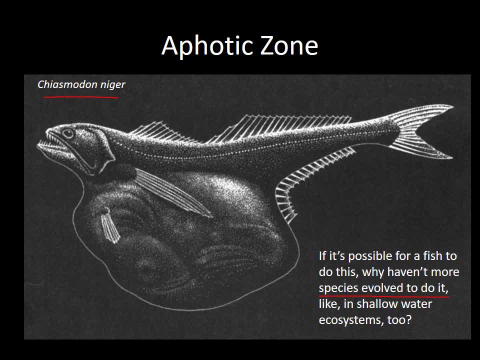 that we see in the water eating us. Well, probably one of the reasons that this strategy of swallowing large prey can work in the deep sea but not in the shallow sea is because fish are few and far between in the deep sea. So one of these fishes that has a large meal like this: 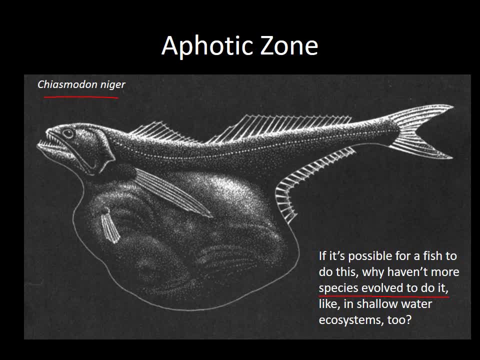 will probably not encounter any other fish for a long time after having that large meal. so it can sort of slowly digest this large, ungainly meal, Whereas if a fish ate such a large prey that it immobilized itself in shallow waters, then this thing would be sort of like a sitting duck. 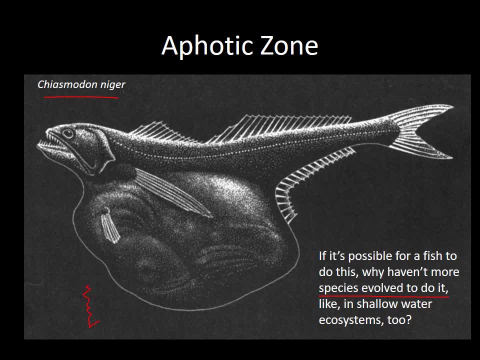 for other fish to come up to and take a bite out. of. So here's another fish that's going to take a bite out of this balloon-like fish here. So you don't want to have a big meal that's going to immobilize you. 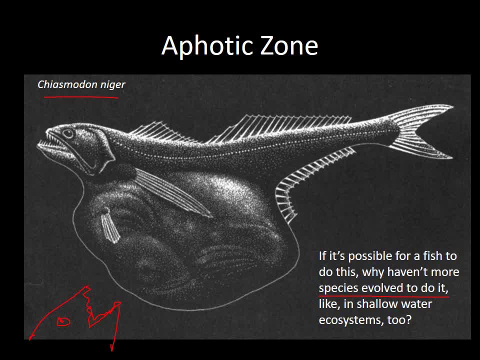 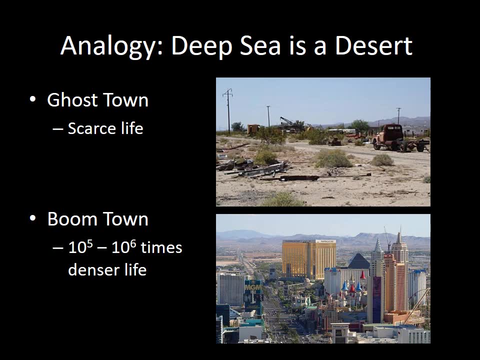 if you're in an area where there's other hungry mouths, because then you'll just be the next meal, All right. so the deep sea environment is kind of a bimodal or bipolar kind of area. You've got some areas. 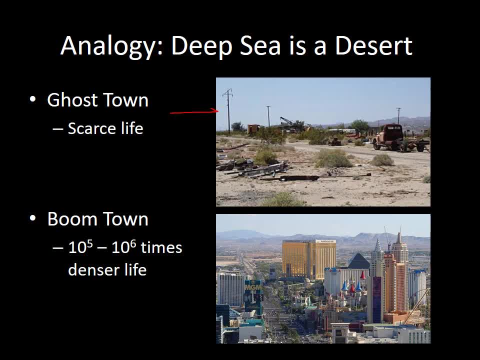 the majority of the deep sea actually- that are like a ghost town where life is very scarce, But then there's certain places in the deep sea where there's a ton of life, And the analogy I like to make is that most of the deep sea is like the desert. 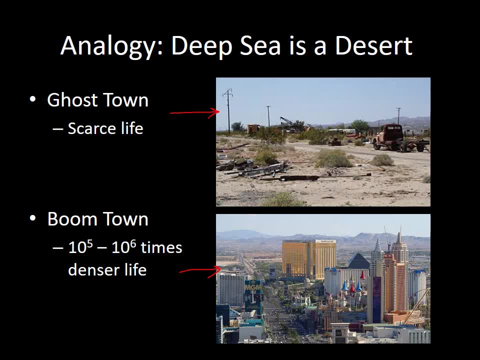 It's sparsely populated, People are few and far between. But then some areas are like Las Vegas or Reno, Nevada, where it's in the desert but there's a huge concentration of life in a small area that's many orders of magnitude more abundant. 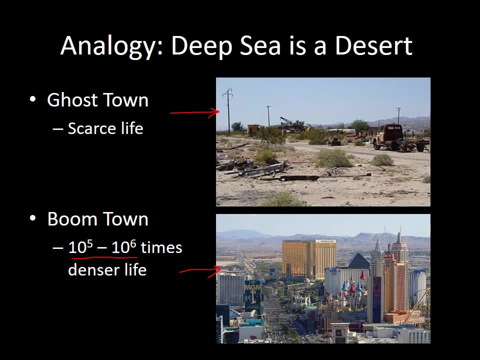 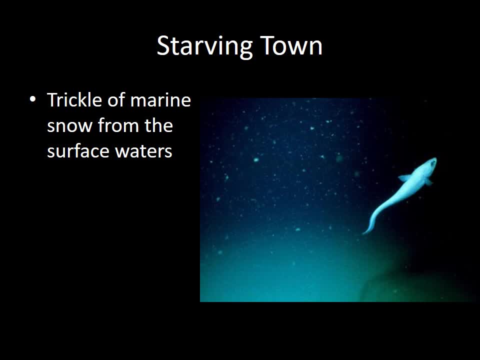 than in the typical desert environment. So this is what most of the deep sea life, most of the deep sea is like. It's this resource-scarce environment where everything is dependent on that slow, sparse trickle of marine snow from the surface waters. 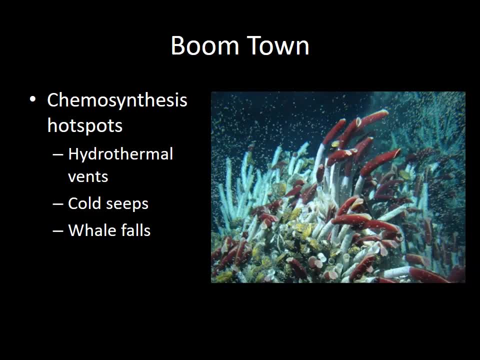 But then there are certain places where there's incredibly abundant life, these Las Vegases of the deep sea, And it's because of sources of extra organic matter in those places via chemosynthesis. So we call these chemosynthesis hotspots, And there's three types that I would like you guys to know. 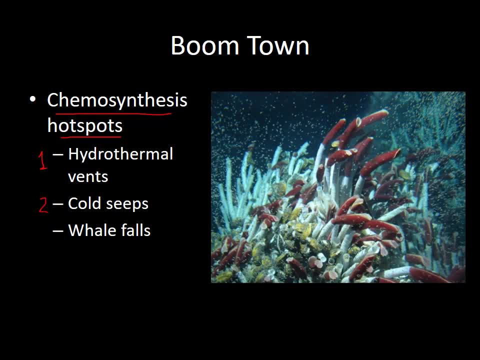 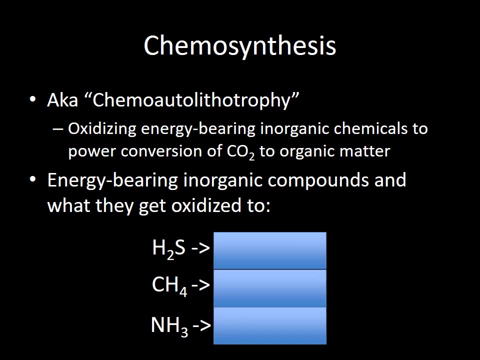 Hydrothermal vents, cold seeps and whale falls. So I'll talk about what each of those chemosynthesis hotspots is like and what the food chains are like in these places. So chemosynthesis- The word's obviously similar to photosynthesis. 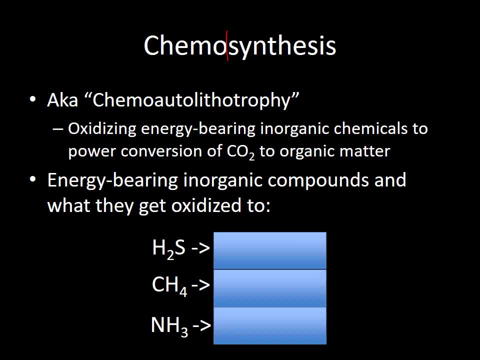 but it's chemo instead of photo. So another word for chemosynthesis is chemoautolithotrophy. So it basically means making organic matter using energy-rich inorganic chemicals as your power source, So instead of using sun as the power source. 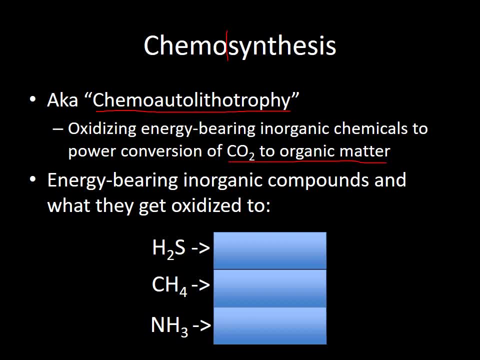 to turn carbon dioxide to organic matter, you're coupling the oxidation of energy-bearing inorganic chemicals with the synthesis of organic matter, And energy-bearing inorganic chemicals can be different kinds of chemicals depending on what's available. So some of the common types of energy-bearing inorganic compounds: 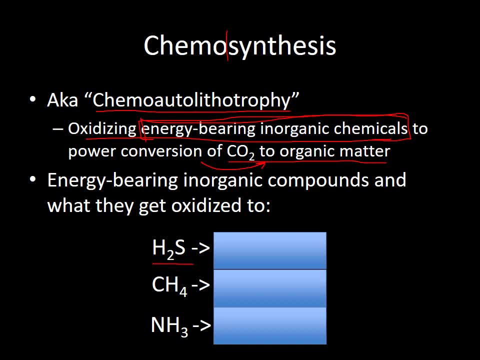 that support chemosynthesis are hydrogen, sulfide, methane and ammonia. All three of these chemicals seep out of the seafloor in various spots and can be oxidized, combined with oxygen, to yield energy that can be coupled with a synthesis of organic matter. 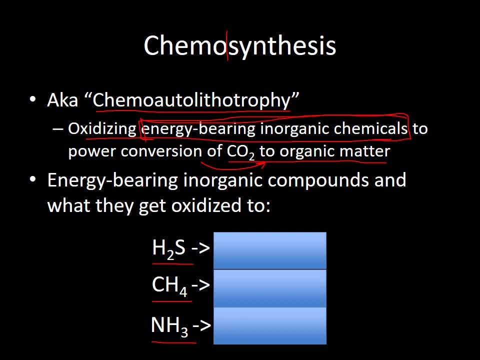 by certain microbes. So when this happens for hydrogen sulfide, it's turned into sulfate. When this happens for methane, it is turned into carbon dioxide. ultimately, When it happens for ammonia, the ammonia is oxidized to nitrite and nitrate. 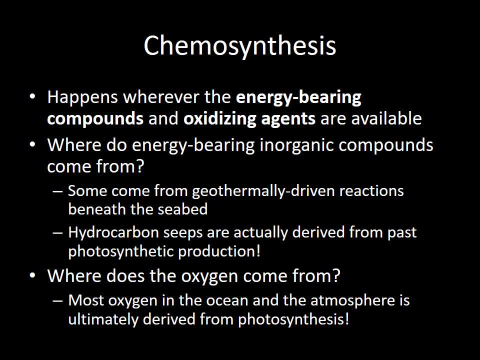 Okay, so chemosynthesis doesn't just happen in the deep sea. Anywhere that you have energy-bearing compounds and oxidizing agents, chemosynthesis will happen. So it can happen beneath the mud in shallow waters, for example, But it's really significant in places. 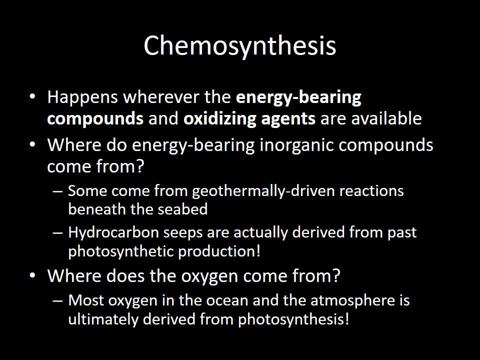 where there aren't a lot of other sources of primary production and where there's a really large source of the energy-bearing inorganic matter, Inorganic compounds. So what would be some of those large sources of energy-bearing inorganic compounds that chemosynthetic organisms can use? 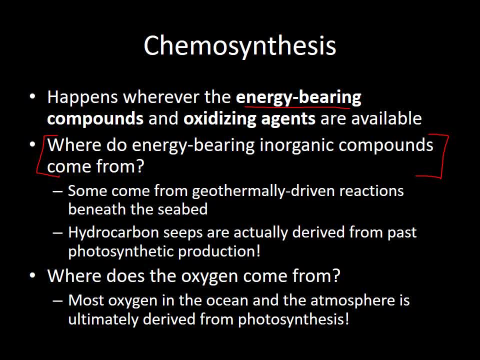 Some come from geothermally-driven reactions beneath the seabed, So heat beneath a seafloor can cause these low-energy compounds to combine into higher-energy compounds that will then seep out of the seafloor and be a fuel. And then there are some places. 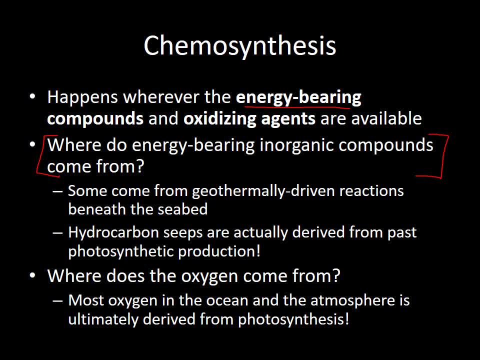 where hydrocarbon seeps out of the seafloor. So methane seeps out of the seafloor. Interesting thing about where these hydrocarbon seeps are- where there's methane or oil seeping out of the seafloor is even though we call that chemosynthetic primary production. 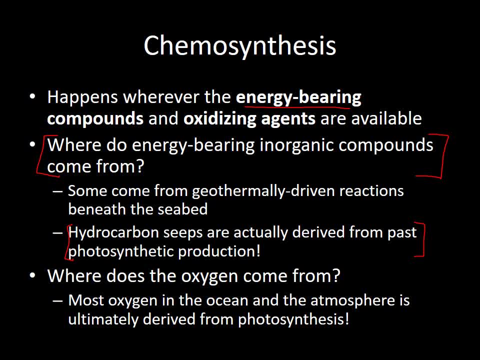 it's actually based on ancient primary production, because those fossil fuels beneath the seafloor are the remains of ancient, largely photosynthetic organisms. Okay, And where does the oxygen come from? in the deep sea that's used in chemosynthesis- Most of the oxygen, ironically. 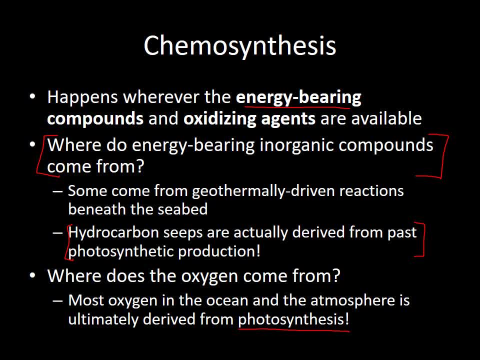 is ultimately derived from photosynthesis. So photosynthesis creates oxygen in the atmosphere which diffuses into the ocean, and then ocean currents carry that to the deep sea. So even though we think of chemosynthesis as being this thing, that's totally separated. 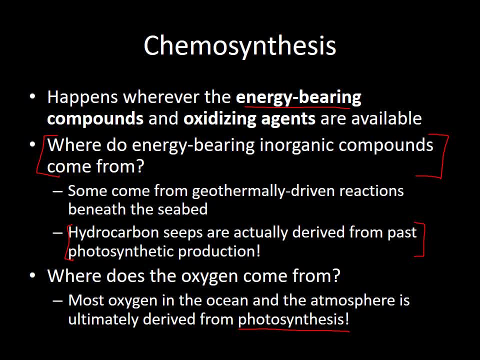 from sunlight and photosynthesis, because some of the compounds that are used in chemosynthesis are ultimately derived by photosynthesis and the oxygen for chemosynthesis was created in other parts of the world by photosynthesis. chemosynthesis is not as independent. 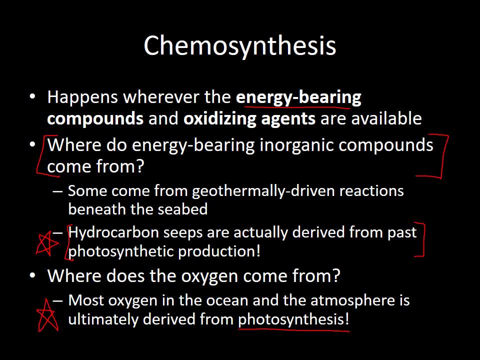 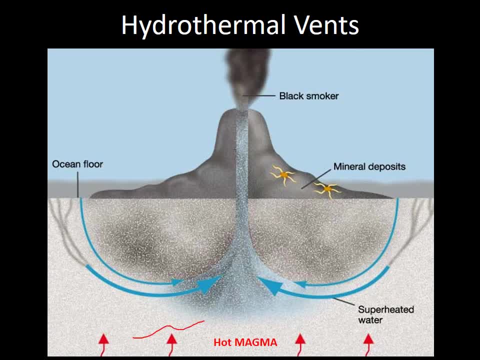 of photosynthesis, as we might think. So this is a diagram of what we call a hydrothermal vent, where there's heat sources beneath the seafloor and that causes warming of water, which rises and percolates through the seafloor. 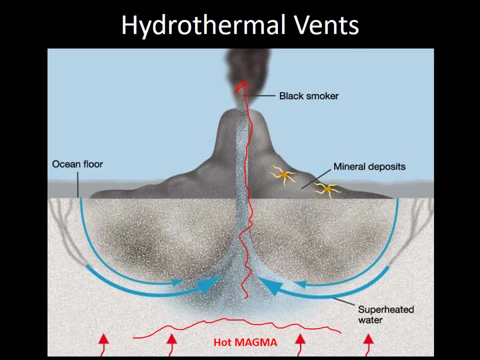 until it comes out at the surface and this sort of creates this convection where water is being drawn into the seafloor in some areas, and then there are these chemical reactions that happen that create energy-rich compounds in that water, and then the energy-rich compounds in that water 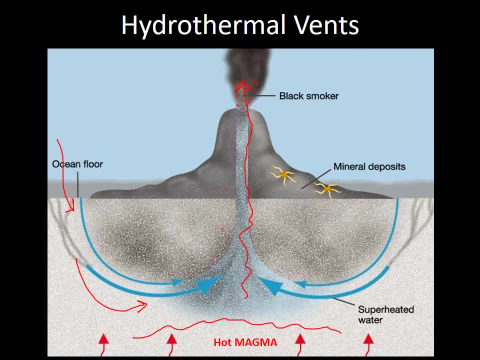 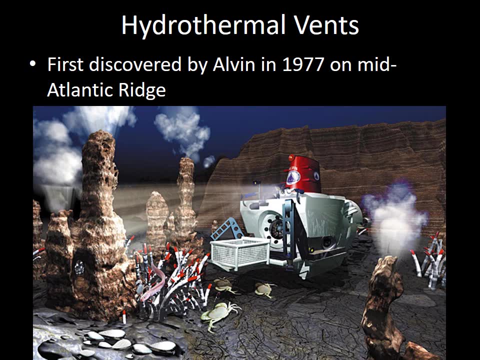 can be used by chemosynthetic bacteria to create organic matter. So these ecosystems were first discovered by the submarine Alvin in the 70s on the Mid-Atlantic Ridge. So the submarine was just down there to look at the geology of the Mid-Atlantic Ridge. 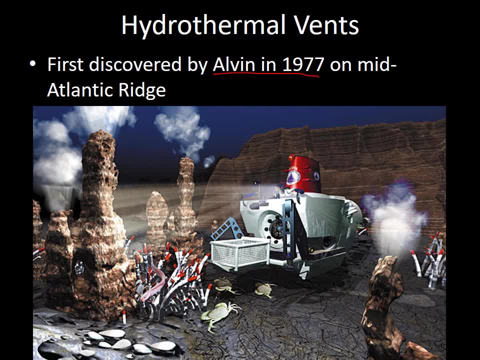 to learn more about plate tectonics and things like that, and they were not expecting to find a lot of deep-sea life there, but they found these incredibly rich and weird communities of life and later learned that it was chemosynthesis. 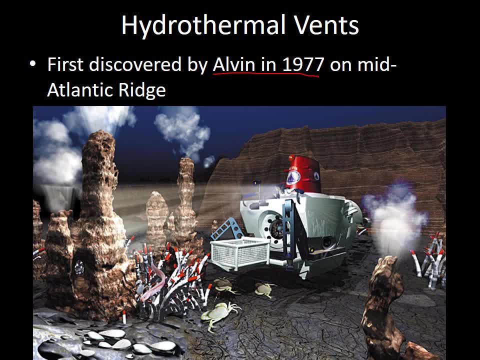 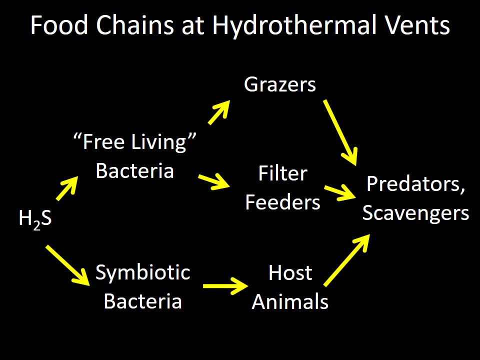 that was supporting that abundant life. So how do the food chains work based on chemosynthesis? Well, it all starts with the energy-bearing inorganic compound, which, for this example, is hydrogen sulfide, So chemosynthetic bacteria. 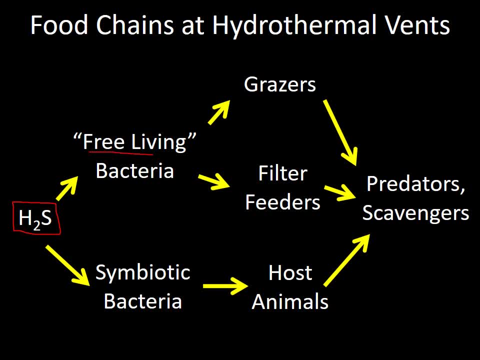 which can be just out in the environment, which we would call free-living bacteria. they can use that hydrogen sulfide as their energy source and increase their, their own abundance, And so they grow based on that chemosynthetic, autotrophic primary production. 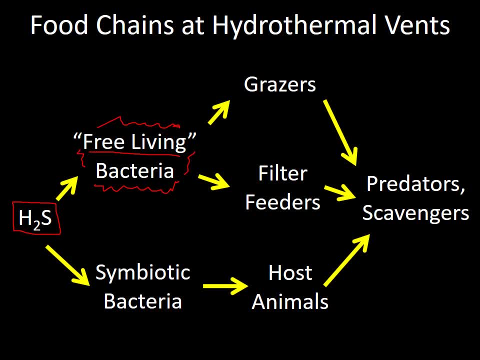 And then they can in turn be eaten by grazers or filter feeders. Free-living bacteria could be on the bottom, attached to surfaces, or they could be just drifting around in the water, So free-living doesn't necessarily mean that they're drifting around in the water. 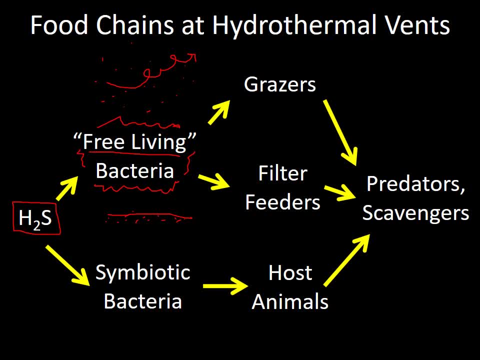 It could mean that they're attached to the bottom or in the water. So if they're attached to the bottom, they're going to be eaten by grazers, which would be little things that like a snail that trundles along the bottom. 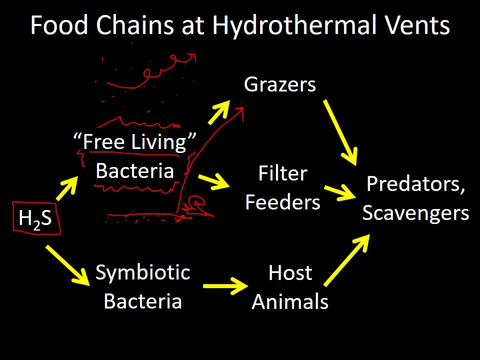 and eats the bacteria that's attached to the bottom, Whereas if if there are free-living bacteria that are drifting around in the water, they can be eaten by filter feeders, which would be things like I don't know. let's say it's sea anemone. 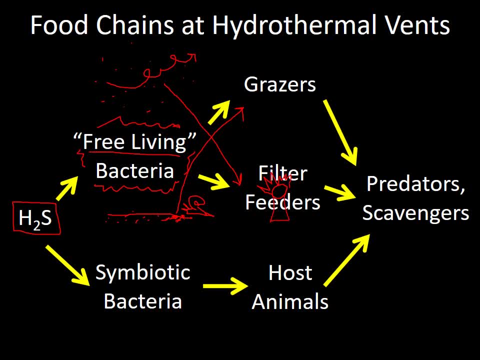 that is filtering the water and collecting the free-living bacteria in its tentacles. Okay so, or it could be a barnacle, could be any kind of filter or suspension feeder. Okay, so that's how free-living bacteria gets eaten. 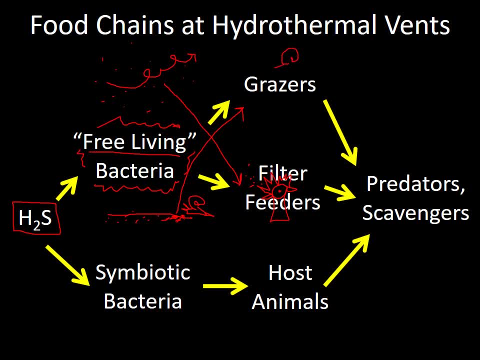 These grazers, like the snail or the anemone. they can in turn be eaten by predators and scavengers, which would be like fish or crabs, and those are going to eat the grazers and the filter feeders. 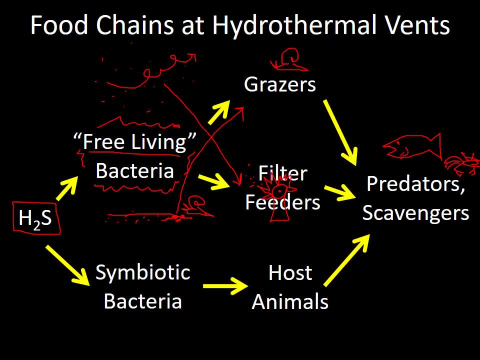 So that would be the top level in the food chain. Okay, so not all bacteria are free-living, though. There are some of what we call symbiotic bacteria. So symbiotic bacteria live inside host animals, So those weird worms with the red lip looking things on them. 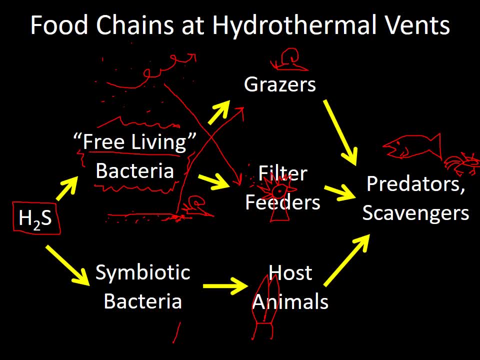 are an example of host animals for symbiotic bacteria, and the bacteria live inside those animals, And so the transfer of primary production is from the symbiotic bacteria to the host animals, but it's happening inside the host animals, So it's a 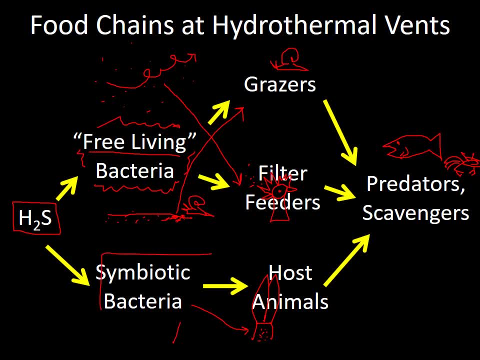 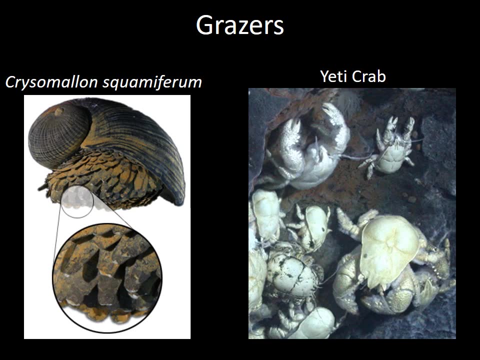 sort of like you've taken these two parts of the food chain and kind of almost combined them into one level, All right, And then those animals can be eaten by predators in turn. so that sort of completes the food chain. So let's give some examples of organisms. 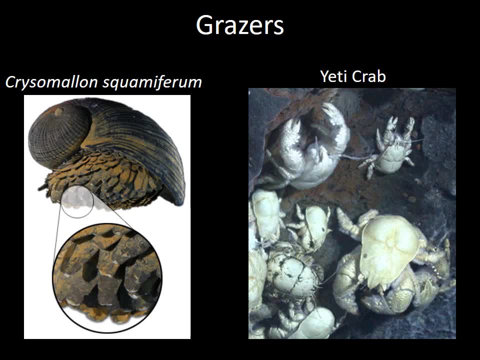 that live at hydrothermal vents, that would be in these different spots in the food chain. So, grazers, These are the organisms that are scraping the chemosynthetic bacteria, the free-living chemosynthetic bacteria, off the rocks or mud. 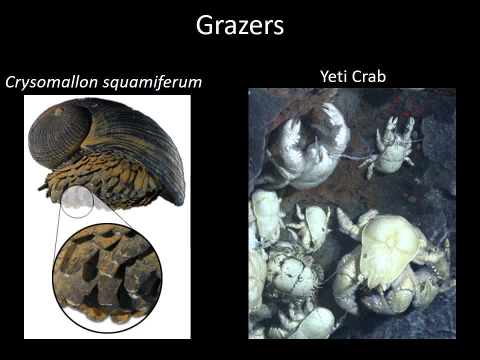 So these Yeti crabs- named because they've got these hairy furry bits on their claws that help them scrape bacteria off of the rocks- and they look kind of like the mythical abominable snowman or Yeti that was covered in white fur. 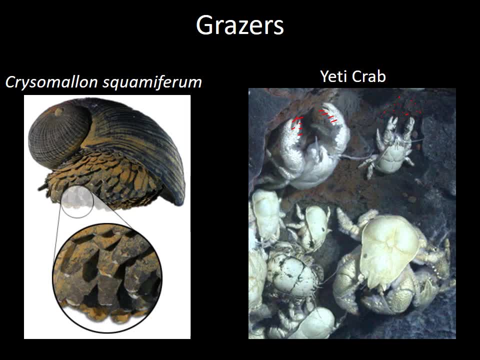 So that's why they're called Yeti crabs, and they scrape the bacteria off the rocks and stuff their faces all day. And then there are a variety of gastropods, like this snail chrysomelon squamiferum. 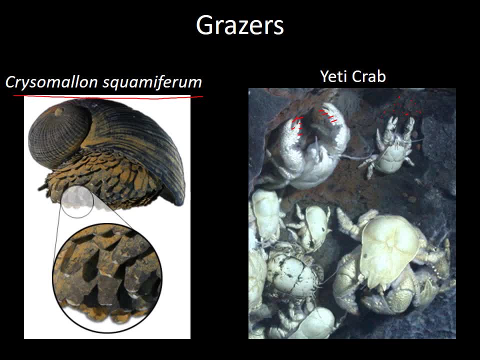 that have rasping body parts that help them scrape the bacteria off of the substrate. This particular snail is unique in the world in that it has iron pyrite, mineral that creates the hard parts of the scraping apparatus on its foot. So most organisms 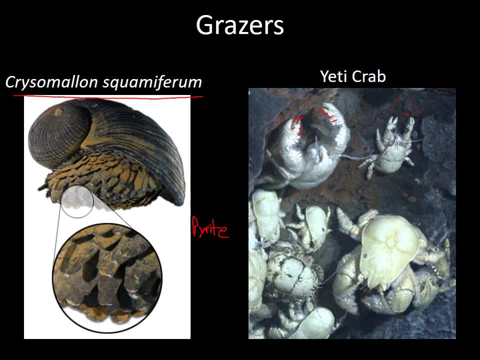 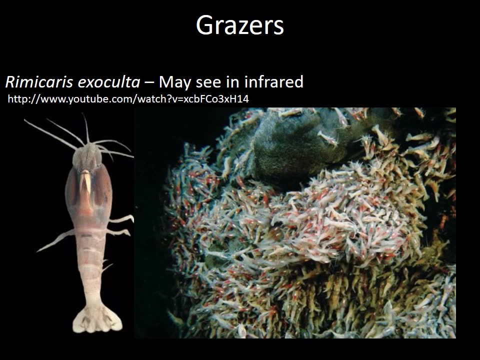 if they have hard parts, they're made of calcium carbonate or silica, but this snail has hard parts made of iron pyrite, which seems to be unique in the animal kingdom. All right, another interesting grazer is this shrimp: Rimicaris exoculta. 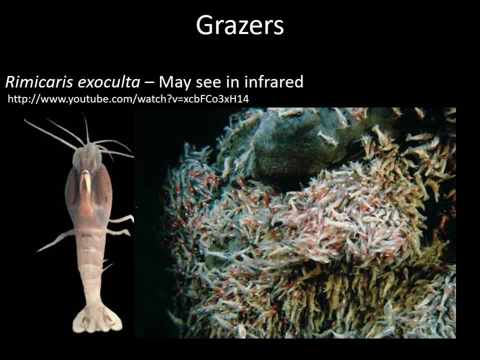 There's a nice video of it on YouTube if you want to go to that link. And these grazers are pretty frisky. They try to swim around and get as close as possible to right where the highlands are, where the hot hydrothermal vent waters are coming out. 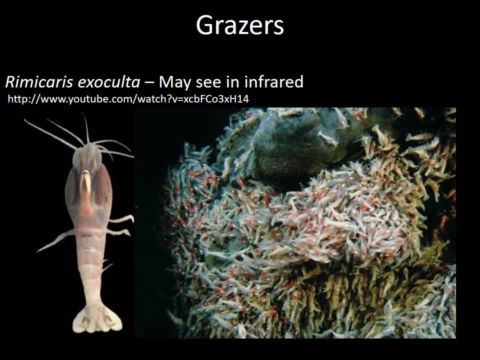 without getting instantly cooked by the hot hydrothermal vent waters. So they need to make sure that they avoid the really hot waters And to do that they have these special eye-like structures that are not actually eyes, but they're able to see heat. 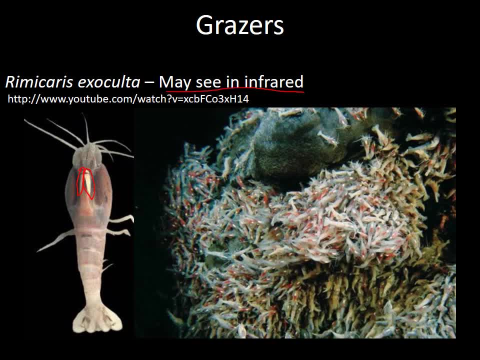 So they can see in infrared, or at least we think they can, And that allows them to see where there's water that's too hot for them to go into and get just close enough to get the bacteria out of it, bacteria off the rocks near those areas. 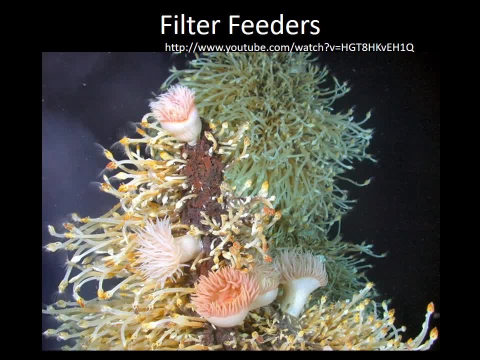 without getting roasted in the super hot water, All right. so there's a huge variety of filter feeders in hydrothermal vent environments, And what type of filter feeders you have really depends on where the hydrothermal vents are. So there's hydrothermal vents. 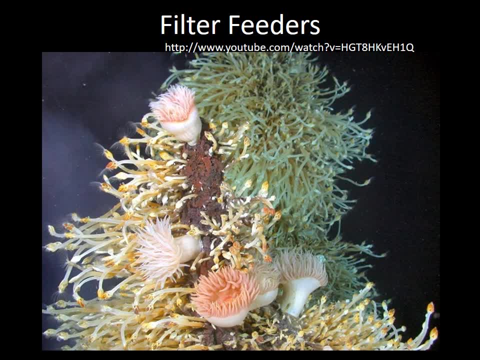 in various places of the seafloor all around the world And because they're separated by long distances, organisms- really different organisms- have evolved in the different hydrothermal vents of the world, So some hydrothermal vents might have a lot of barnacles. 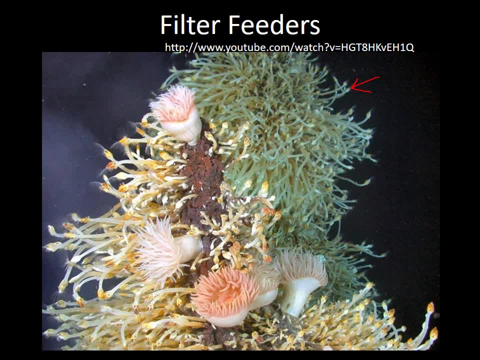 Like these stalked things in a hydrothermal vent off Antarctica are barnacles with long stalks And they're filter feeding the free-living bacteria out of the water. And then these are anemones, obviously, and they're also filter feeding. 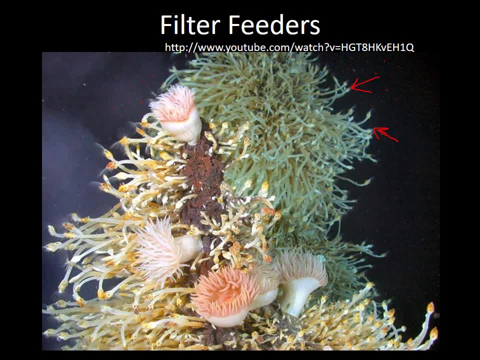 the bacteria out of the water. But at other hydrothermal vents you would have different organisms, like you might have clams or mussels that are the filter feeders, And it just really depends on which hydrothermal vent you're at. So perhaps the most famous, 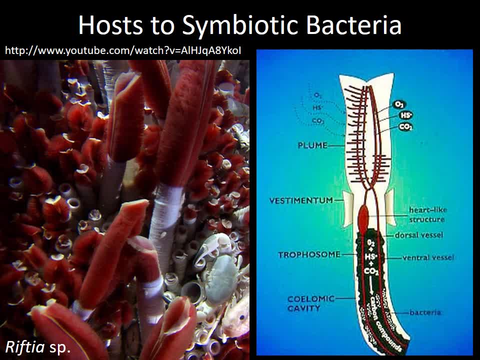 hydrothermal vent organism of all is Riftia species. It's a type of polychaete worm And its ancestors were traditional filter feeders. But this one is not a filter feeder. It doesn't feed on particles from the water. It absorbs oxygen, hydrogen, sulfide. 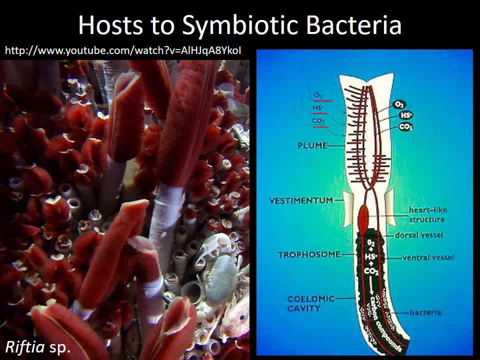 and carbon dioxide into its bloodstream. Through the gills it pumps that into an organ in its body called the trophosome, which is where it stores its symbiotic bacteria And the symbiotic bacteria, the chemosynthetic symbiotic bacteria. 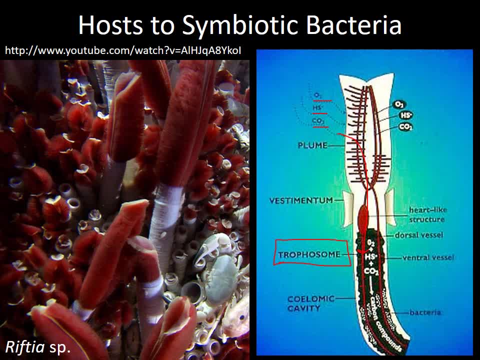 that live in the trophosome are able to convert the hydrogen sulfide, carbon dioxide and oxygen into organic carbon compounds that are then absorbed directly into the bloodstream of the worm. So it doesn't really have to eat in a traditional way, It just absorbs chemicals. 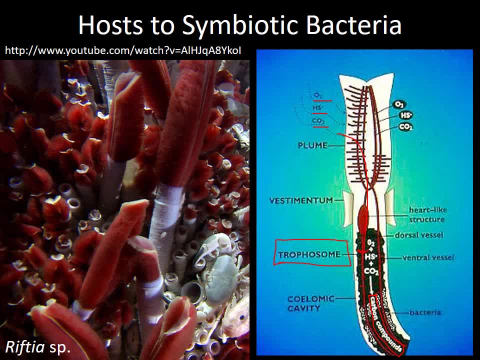 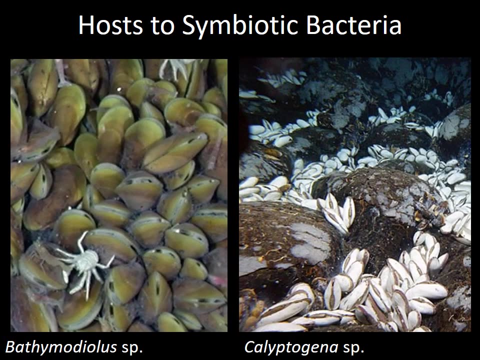 And then the bacteria in its body turn those chemicals into organic matter. And there are other hosts to symbiotic bacteria that live on other hydrothermal vents in the world that use similar systems. Some of those other organisms that also have symbiotic bacteria include bivalves, like the Bathymodialis mussels on the left. 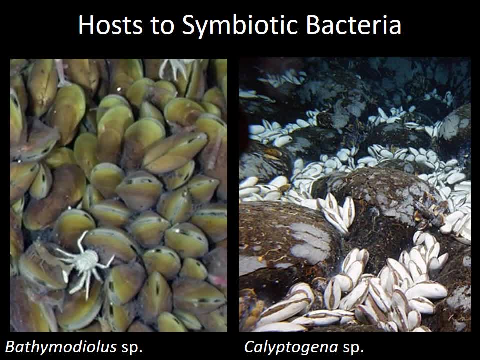 and the Calyptogenia clams on the right. Scientists have tried eating these clams and mussels because they're really big and tasty looking, but apparently because of all the hydrogen sulfide in their bodies, they taste terrible. This is one of those big Calyptogenia clams. 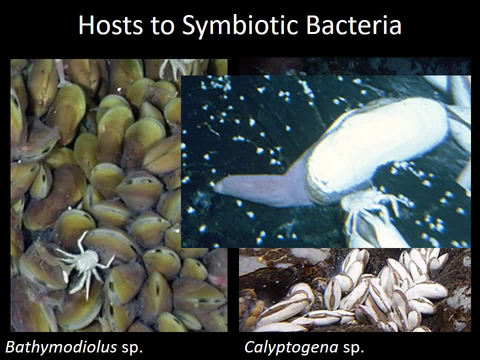 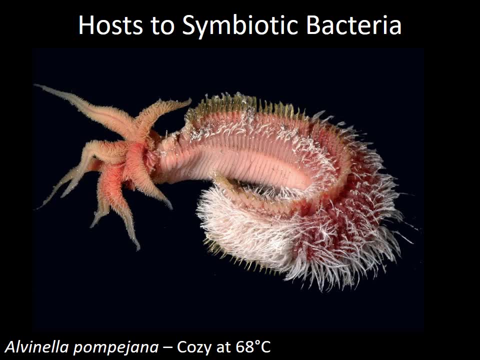 You can see it looks really meaty, but it tastes terrible. Okay, so some of the organisms that live in these hydrothermal vents are remarkable in how tolerant they are of high temperatures on the hydrothermal vents. So this is Alvanella pompeiana, the Pompeii worm. 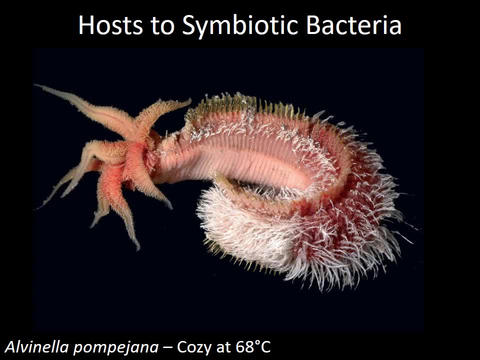 It's a type of polychaete worm that is a filter feeder and a host. Well, actually, I can't- Honestly, I can't remember if this is a filter feeder or a host of symbiotic bacteria, but I'm highlighting it because it's very tolerant. 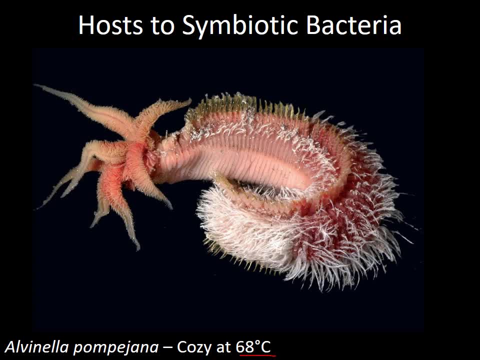 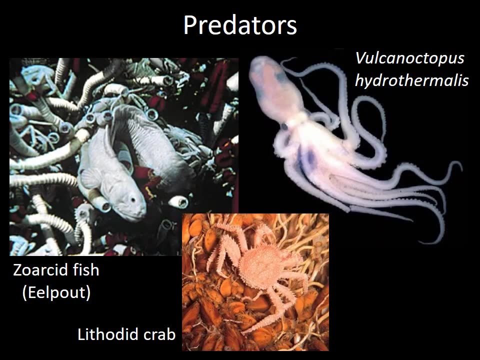 of extremely high temperatures, And it's able to live in the walls of the chimney-like mineral structures that form at these hydrothermal vents. and it can tolerate 68 degrees Celsius, which is high enough that it would cook most organisms. So at the top of the food chain. 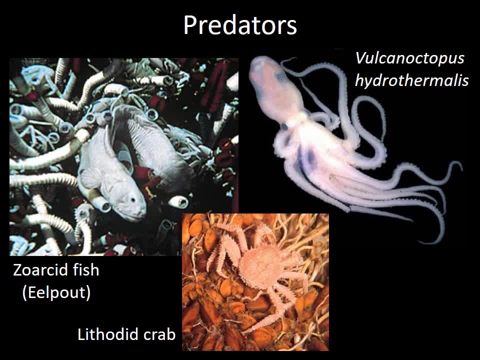 in the hydrothermal vents are various predators and scavengers, So some of these are organisms that would be found in other parts of the deep sea as well, and they just opportunistically visit and feed in hydrothermal vents. So this fish called the eel pout. 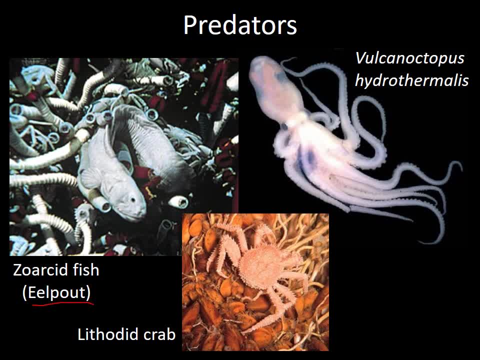 in the Zoarsid family is a fish that's found throughout the deep sea, but they're especially abundant in hydrothermal vents, because there's more food there. There is a species of octopus that is particularly associated with hydrothermal vents, though. 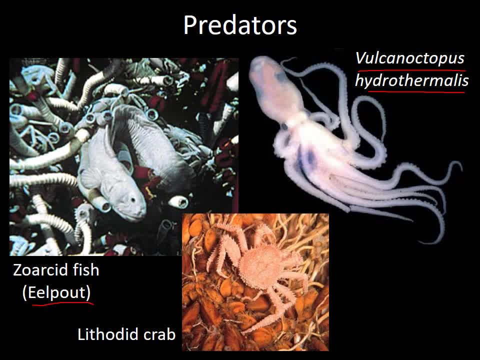 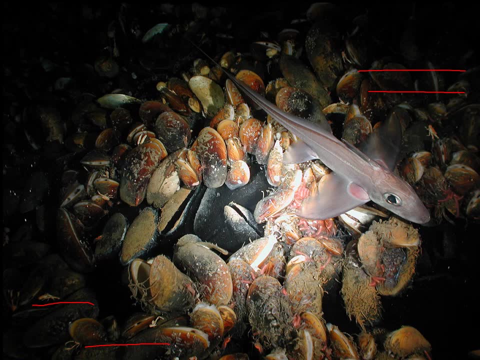 called Vulcanopterus hydrothermalis, and there are some lithodid crabs, a variety of crabs that are scavengers in hydrothermal vent ecosystems. There are some interesting deep-sea fishes that I want to highlight here, called ratfishes. 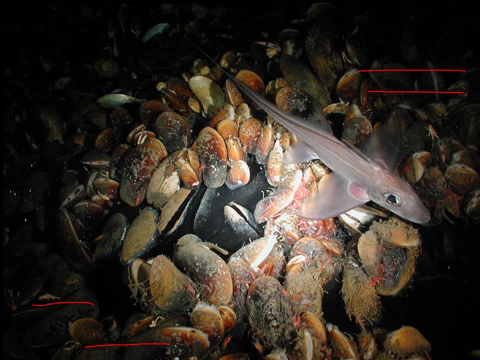 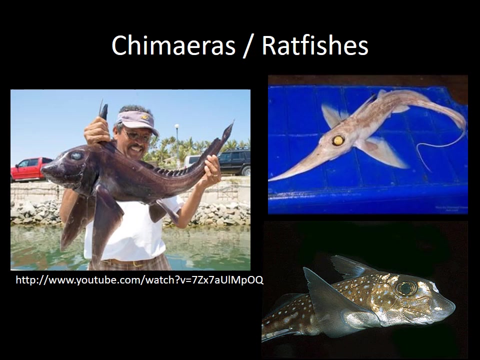 Ratfishes are actually more closely related to sharks and rays than they are to other fishes, and they're really weird-looking and they often live in the deep sea, so I want to say a few things about them. So they're also known as chimeras. 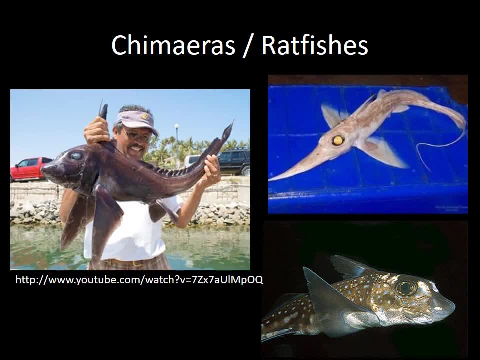 A chimera is an animal that's made from a combination of parts of other animals, so it's a mythological animal, but because these seem to sort of combine odd bits and pieces of different organisms, or at least that's what the people who named them thought- 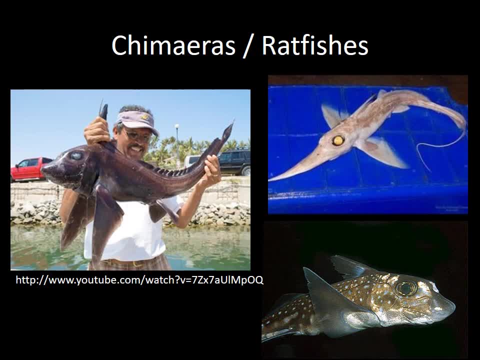 we call them chimeras or ratfishes. Some people think that the face looks like a rabbit or a duck and then the body looks like a snake, and anyways, that's why they're called chimeras or ratfishes. So they're cartilaginous fishes. 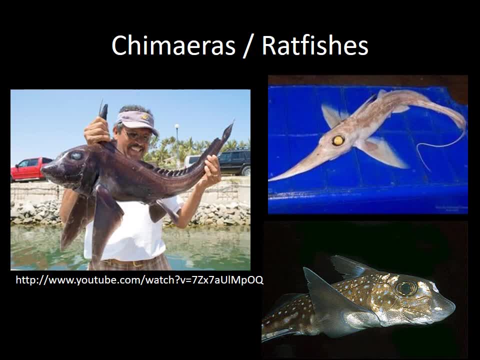 Their closest relatives are the sharks and rays, But unlike the sharks and rays they have, instead of you know, toothy mouths. I guess their mouths are more similar to rays in that their mouths are underslung and they tend to have more crushing mouthparts. 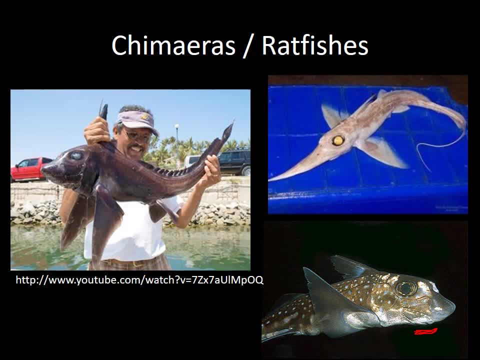 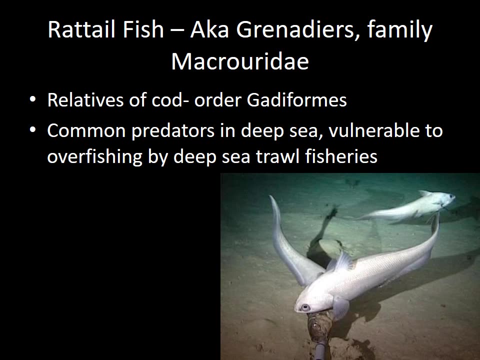 than sharp teeth, So they like to eat clams and mussels in particular. Many species do. Okay, so not to be confused with the ratfishes. are the rattailfish So similar to the ratfishes? they have long, skinny tails. 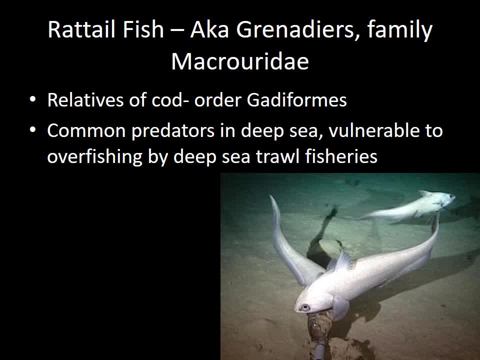 but they're in a totally different, different group of fishes. They are bony fishes, so they have scales and calcium carbonate bones, unlike the dermal denticles and cartilaginous skeletons of the rattailfishes. So they're actually related to the shallow-water cod. 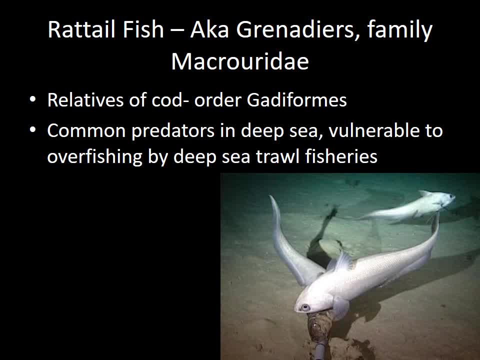 They're in the same order order, Gatiformes, And they're quite common predators in the deep sea. So because they're large and common, they are a target increasingly of deep-sea trawl fisheries. Particularly Russian trawlers are now dragging their nets. 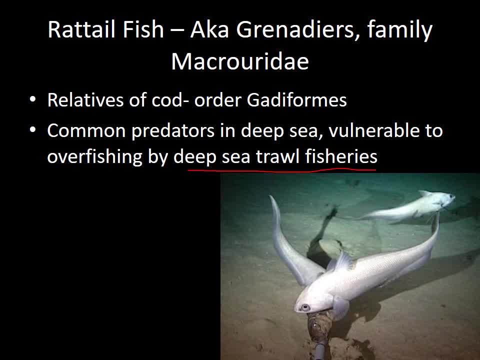 through the deep sea to get these rattailfishes, And they are doing this increasingly as shallow-water codfish are depleted by overfishing. So even though there might be a relatively large abundance of these rattailfishes now, they're very long-lived, slow-growing. 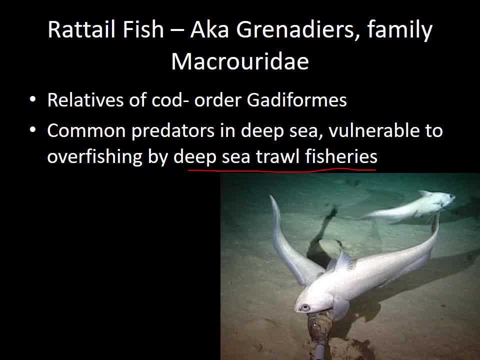 slow-reproducing fishes. That's a characteristic that's common to many deep-sea fishes And therefore their populations are not able to sustain high rates of harvest, And we should avoid the temptation to harvest them just because they seem abundant, because we could very quickly deplete their populations. 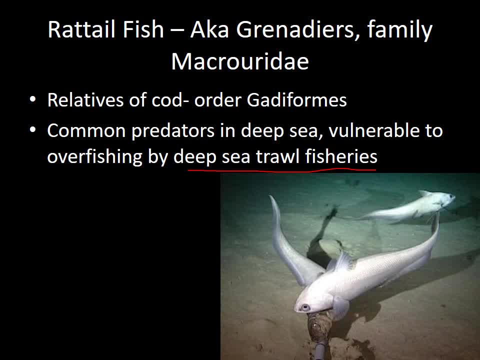 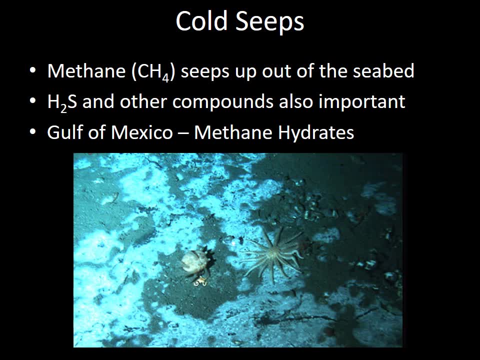 and upset the ecosystem of the deep sea and maybe even make them extinct. All right, So cold seeps are another type of deep-sea habitat where energy-rich chemicals come out of the seafloor, So they're not associated with geothermal activity. 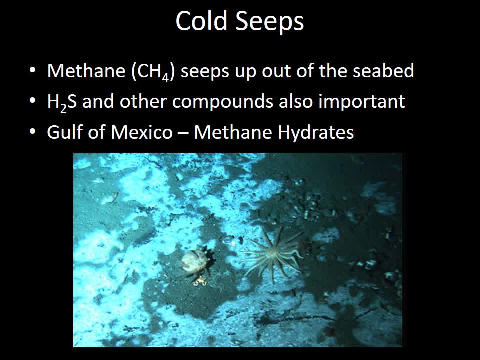 like hydrothermal events. That's why they're cold and we call them cold seeps. But there are energy-rich inorganic chemicals that can seep out of the seafloor even where there's not hydrothermal activity going on. 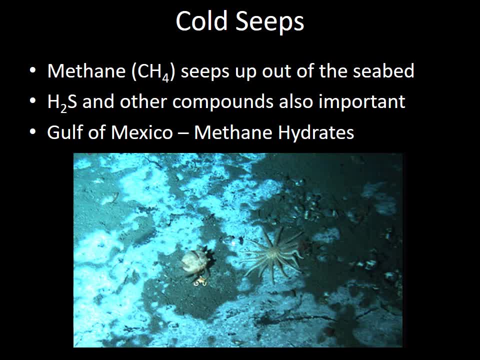 And all those habitats collectively are what we call cold seeps. So a common type of energy-rich compound that seeps out of the seafloor in cold seeps is methane, CH4, also known as natural gas. But other compounds can seep out of cold seeps. 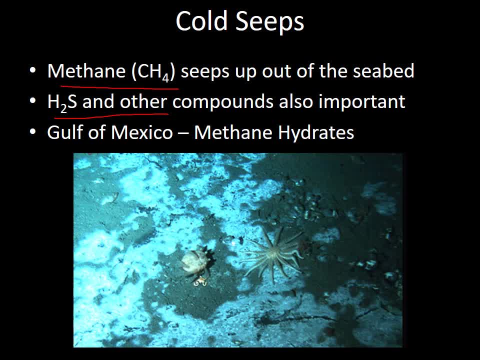 like hydrogen sulfide. It just depends on where you are and what sort of underlying geology and sediments are of that seafloor area. what kind of chemicals are going to be seeping out. So in the Gulf of Mexico there are a lot of places where methane seeps out. 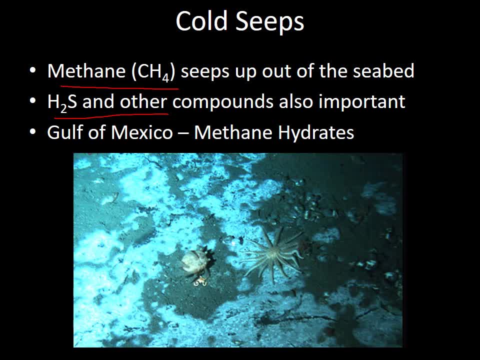 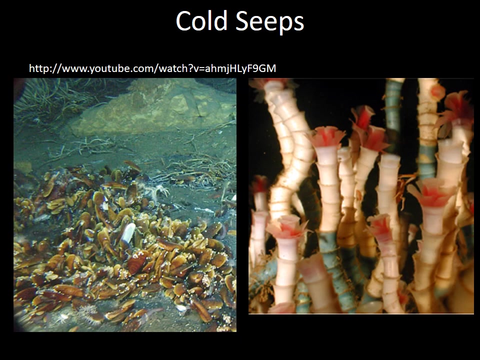 And one of the interesting things that happens when methane comes into contact with cold seawater at high pressure is that it crystallizes into this weird crystal form called methane hydrate, which is sort of a combination of ice-like water, crystals and methane. All right, so some of the types of organisms. 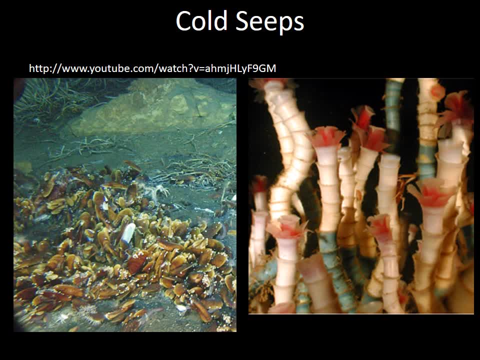 that you'd find at cold seeps are really similar, maybe even the same species that you'd find at hydrothermal vents, because it's a similar ecosystem as far as being based on chemosynthetic primary production. So there are mussels with symbiotic. 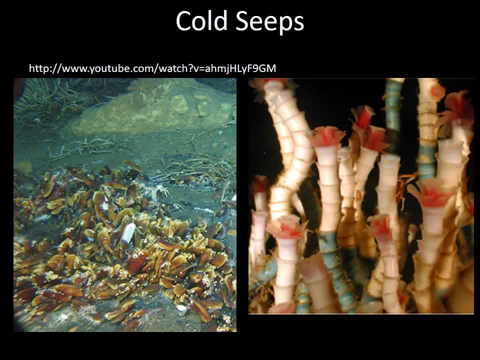 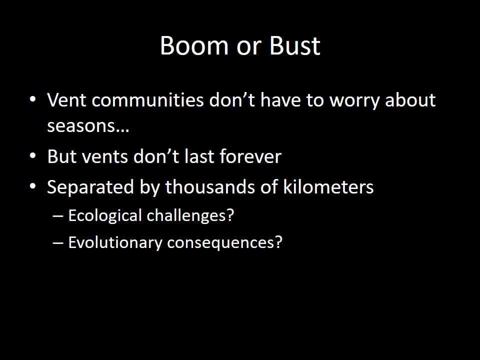 bacteria in them, tube worms with symbiotic bacteria in them, and there's actually quite a bit of overlap between the species found in hydrothermal vents and cold seeps. So hydrothermal vents and to a lesser extent cold seeps can be kind of ephemeral environments. 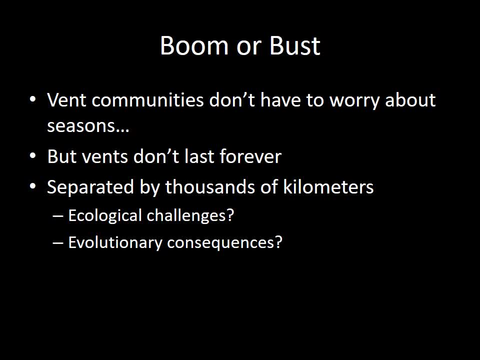 They, although they don't have to worry about seasonal changes like surface environments, do you know? think of how the land is productive in the spring and summer and then it's desolate with everything dying in the fall and the winter. You don't have to worry about that. 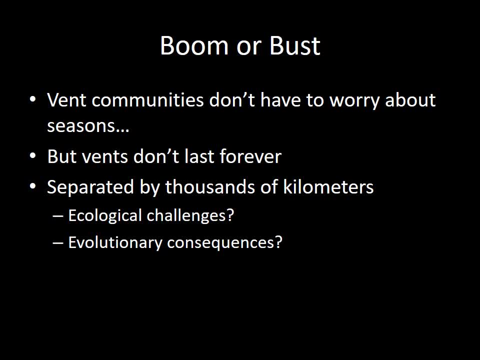 in a hydrothermal vent community, because the hydrothermal vent is just constantly going, whether it's summer or winter. The thing is hydrothermal vents, they don't last forever. They burble out their energy-rich compounds for a while and then, due to geological changes, 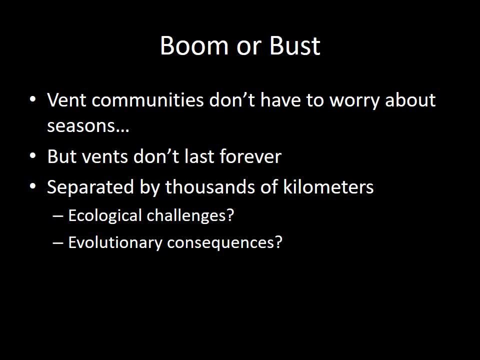 they often shrivel up and stop producing their energy-rich chemicals. So, and at the same time, though, there might be new vents forming in another area. So there's sort of this boom and bust kind of cycle where you could have an area that's really productive. 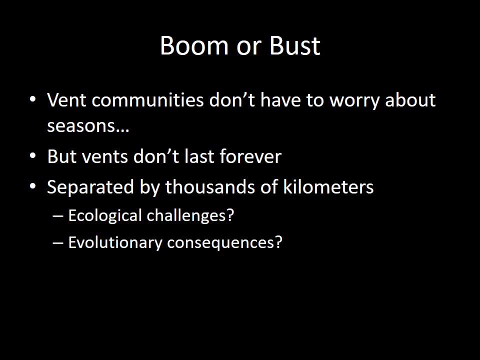 for however many years or decades the hydrothermal vent is active, but then it'll totally collapse once that hydrothermal vent shuts off, And we've actually observed this in some sites that we've visited, and there was abundant life there, but then the vent shut off. 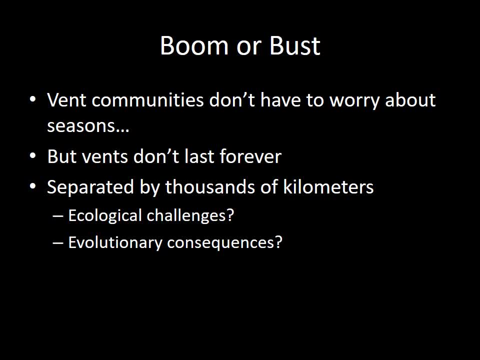 and we went back a year or so later and it was just like a ghost town with no life left there- hardly any life. So this boom and bust cycle is a challenge for the long-term sustainability of life at deep-sea chemosynthetic hotspots. 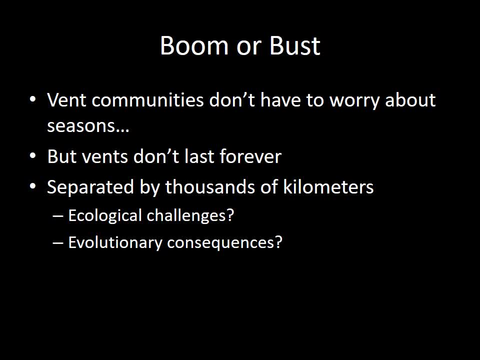 and the organisms that live in these areas have to have some way to have larval dispersal so that, you know, future generations of them will be able to encounter other places that they'll be able to inhabit, because no one deep-sea chemosynthesis hotspot. 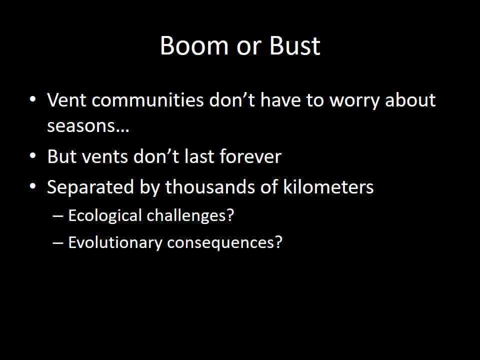 lasts forever. So that's a challenge like: how do you find a new home knowing well? I mean, it's not something that you would think about, since these organisms are not that intelligent, but they need to have some adaptation for getting the next generation. 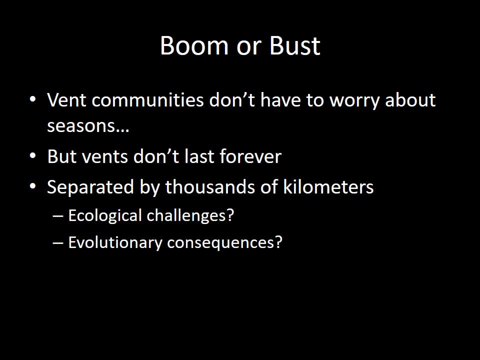 to a suitable habitat, And there's some interesting evolutionary consequences as far as how the isolation of these habitats has led to divergent evolutionary paths in one hydrothermal vent ecosystem versus another. So we'll talk about both of these things, the ecology first. 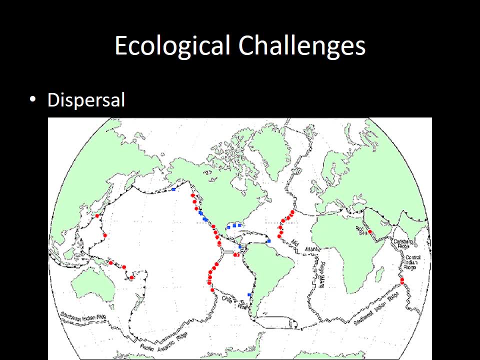 and the evolutionary consequences, So one of the issues being the isolation of these hydrothermal vents. the hydrothermal vents are illustrated on this diagram in the red and cold-seep habitats in blue. As you can see, there's a lot of cold-seep habitats. 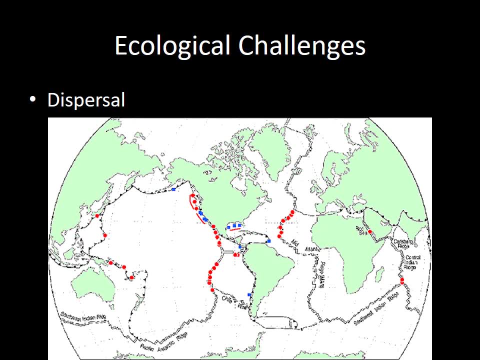 in the Gulf of Mexico. There sort of is a clustered distribution of them, So sometimes there's near neighbors, like within the same tectonic rift system, and in other areas there might be like a large gap with no mode of dispersal. 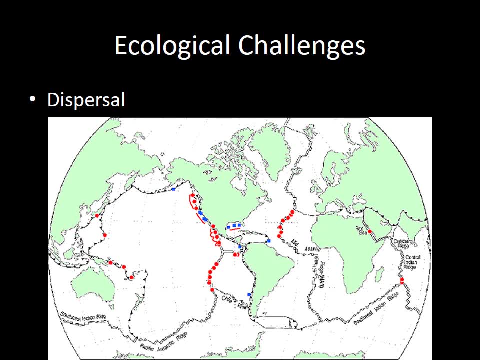 So it would be very hard for an organism to disperse from a hydrothermal vent in the eastern Pacific Ocean to a hydrothermal vent system in the western Pacific Ocean. So you would be unlikely to have species in common between these two systems, Whereas within a single hydrothermal vent system. 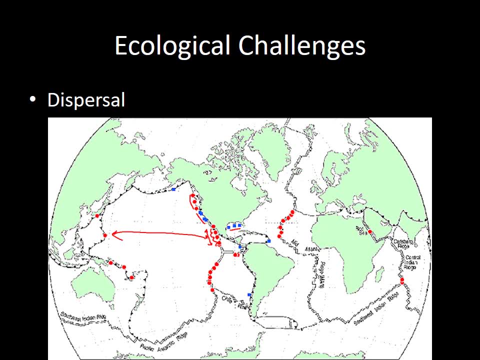 you might have some similarity in organisms that are able to disperse between different vent hotspots that are relatively close on the same system. So you tend to have this interesting biogeographic consequence where you've got these sort of clusters of similar vent communities. 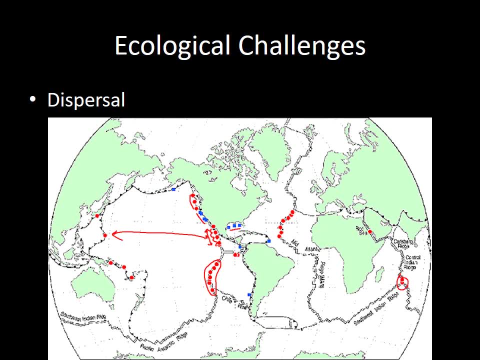 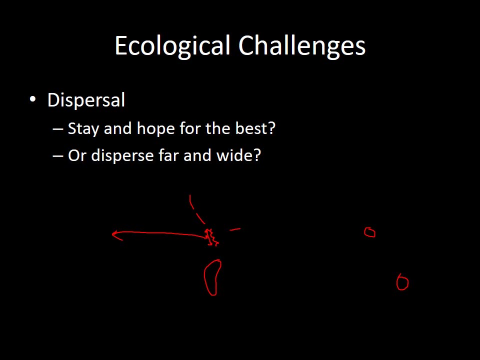 but then the ones that are isolated will have really different kinds of organisms than the ones that than the other ones. So let me make this ink go away. So there's sort of two strategies that you can have if you're an organism on a hydrothermal vent. 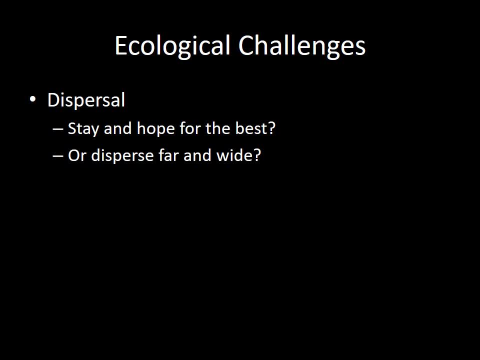 If conditions are good there, your best strategy might be to stay and hope for the best. If you disperse all your larvae far and wide, perhaps very few of them will land in a suitable habitat, And maybe it would be better to just have short-distance dispersal. 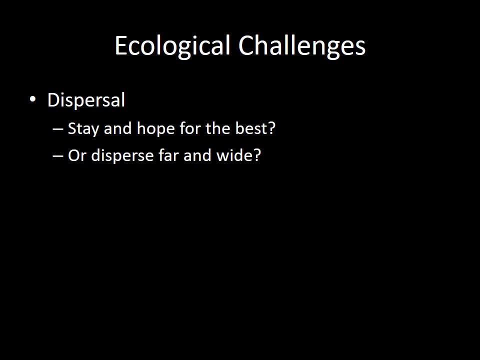 so that they can land in the same hydrothermal vent habitat and survive there. Then again, if you only do that, then when your vent system goes extinguished that's the end of your species. So ultimately that kind of favors the evolution of dispersal far and wide. 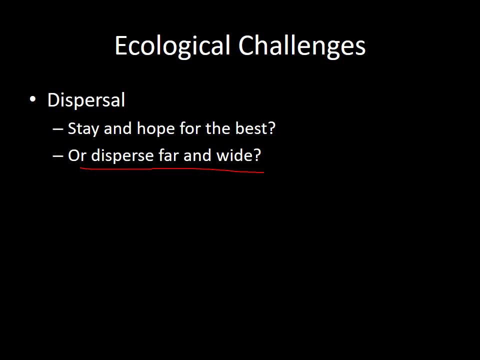 So how do you disperse far and wide, Particularly, if you're a sessile organism like a tube worm, you can't move as an adult. So dispersal at the larval stage is very important. Larval dispersal, All right. 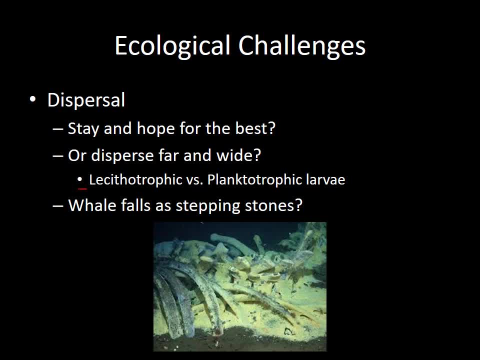 So one way to disperse your larvae far is to have lesothotrophic larvae. Lesothotrophic larvae are larvae that feed on egg yolk, So they are well-provisioned larvae with a lot of fats and proteins in the yolk that's supplied. 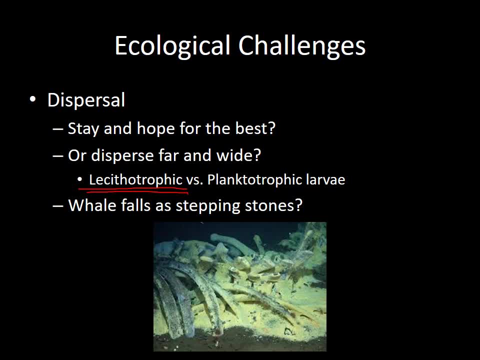 by their parents, And so they can sort of drift for a long time in the plankton, feeding off of their yolk until they find a suitable spot to settle. And then there's another strategy, which is having planktotrophic larvae, which means that you have larvae. 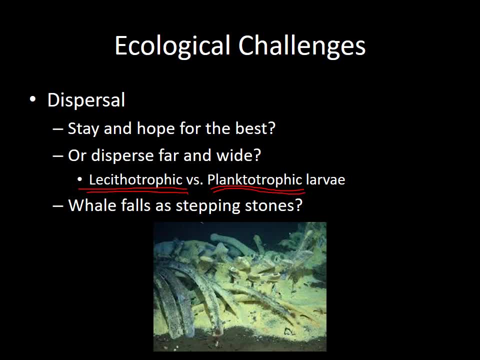 that eat plankton And that keeps the larvae alive for a long time until the larvae hopefully find a place to settle, Sometimes the planktotrophic larvae of deep-sea organisms. so here's a deep-sea hydrothermal vent and it's got some organisms on it. 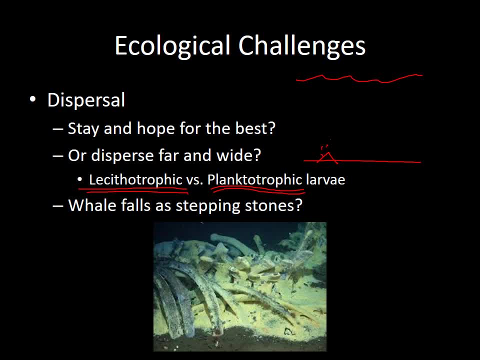 the larvae will be released. and the larvae will go up into the surface waters where there's more plankton for them to eat, and they'll sort of drift through the surface waters as they develop and become big enough to settle and then they'll drop back down. 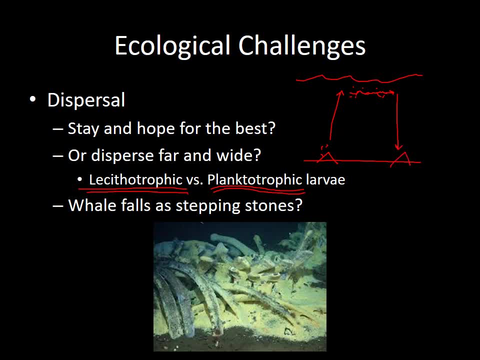 into the deep-sea and hopefully find another spot that's suitable for them to settle and become adult organisms. So that can be a strategy for planktotrophic larvae, whereas for alethysotrophic larvae they might as well just drift through the deep-sea. 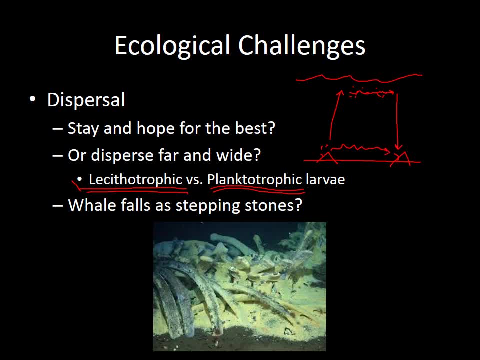 and hopefully find another habitat to settle on. So these habitats may be separated by thousands of kilometers, so the chances of lucking in to finding a new habitat could be pretty low. But one thing that might increase the chances is that you can have these stepping stone habitats. 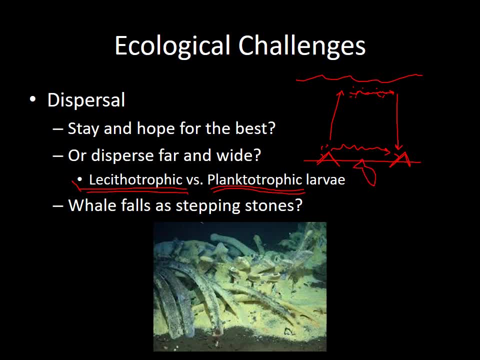 like there's some other place where your larvae might be able to settle and survive and live for a generation or two before the next generation moves on and disperses to another habitat that's more like the hydrothermal vent or deep-sea habitat, And so whale falls. 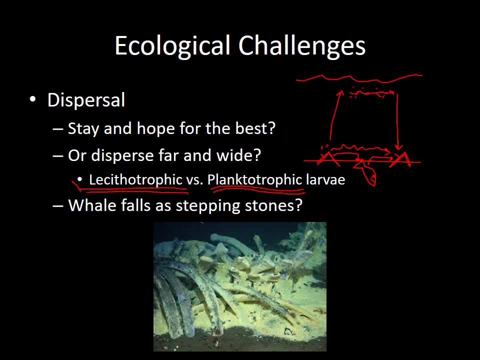 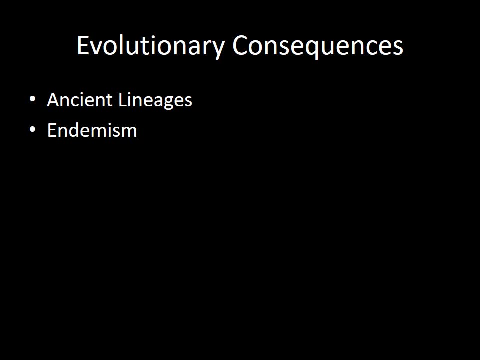 are one of those kinds of habitats. Okay, so one of the consequences of the great separation of chemosynthetic habitats from other chemosynthetic habitats geographically, and their separation from surface habitats, is that there are some ancient lineages on these habitats. 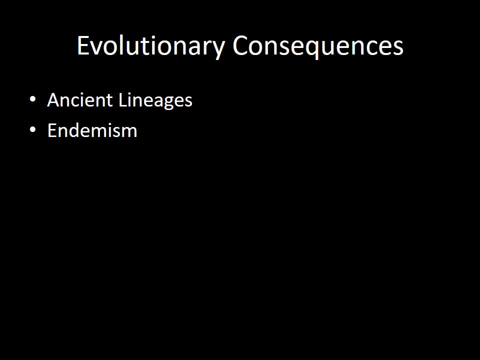 So there may be organisms that their relatives in the surface waters have long since been out-competed and displaced by other organisms, and yet they still persist in deep-sea hydrothermal vents. Another word for these ancient lineages is living fossils, meaning that their 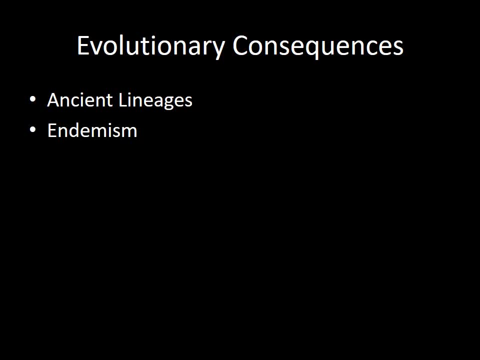 surface-dwelling relatives have gone extinct long ago, but they're still doing their thing down in these isolated habitats of the deep sea. Another consequence is endemism, And endemism means species that are found only in one particular area. So because these areas are isolated, 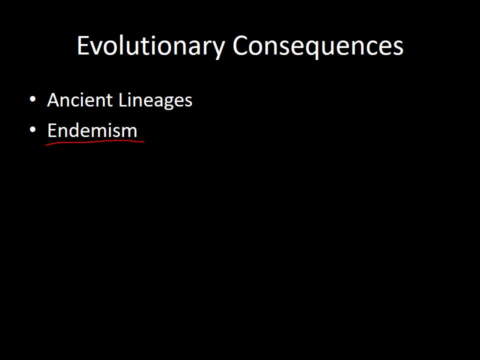 for such long periods of time, they tend to sort of develop via evolution their own unique species that may be found nowhere else. So every time you find a new hydrothermal vent, particularly if it's far away from other hydrothermal vents, there's a strong chance. 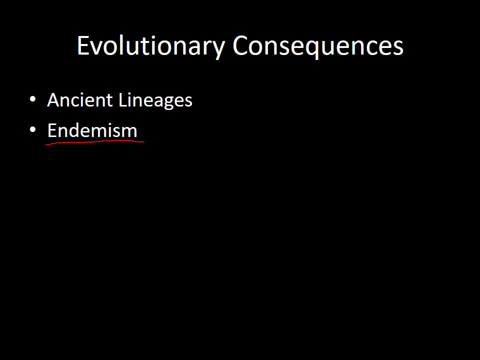 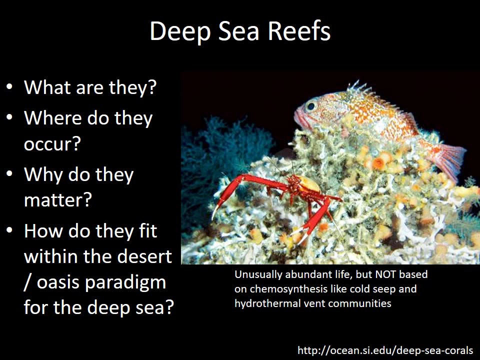 of finding species that are found nowhere else on Earth: endemic species. Okay, moving on to a different kind of structured habitat in the deep sea, we're going to talk about deep-sea reefs, So we'll talk about what they are, where they are found. 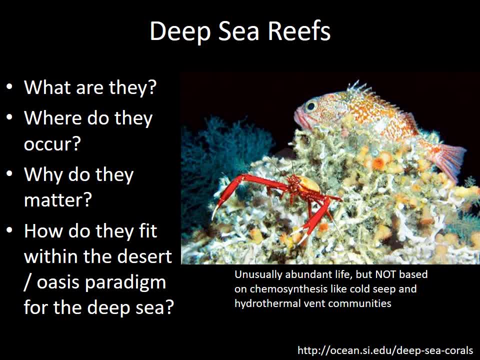 and why they matter and how they fit within this sort of desert environment versus hotspot environment of the deep sea. So the thing about deep-sea reefs is that they do have unusually abundant life, a lot more life than you would find in most parts of the deep sea. 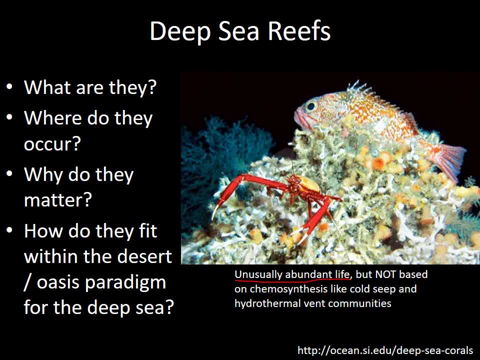 where it's just barren mud plains. The thing is that, unlike chemosynthesis hotspots, they're not based on chemosynthesis, So deep-sea reefs are supported by marine snow from the surface, So marine snow is the thing that reaches them. 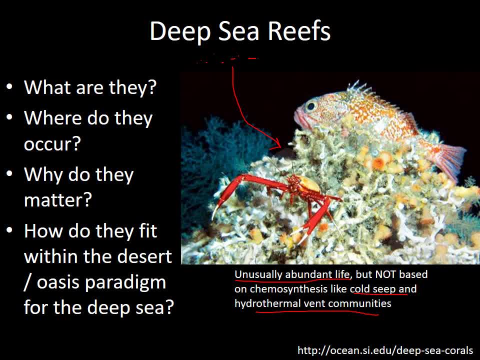 so they are still dependent on that trickle of marine snow down from the surface, but they occur in areas where there's strong currents or large supplies of marine snow that mean that there can be a little more production of benthic life than there would normally be. 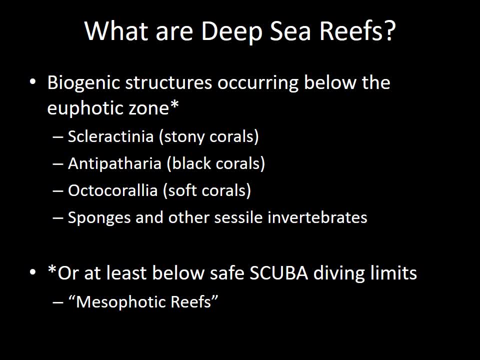 in the deep sea. Yeah, so the definition of a deep-sea reef is: it's a biogenic structure occurring below the euphotic zone, and some of the things that make these deep-sea reef structures are actually pretty close relatives to the things that make. 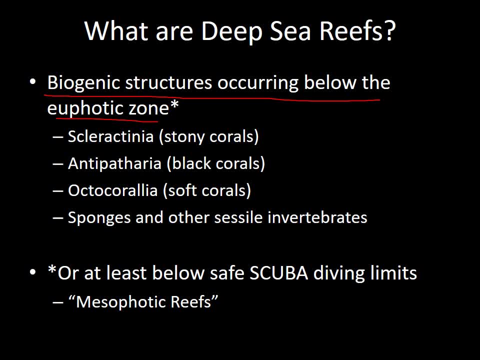 shallow-water photosynthetic reefs, and so there are stony corals in the order Scleractinia that are found in the deep sea, and there are other coral types like the black corals, octocorals, and then there are some other types. 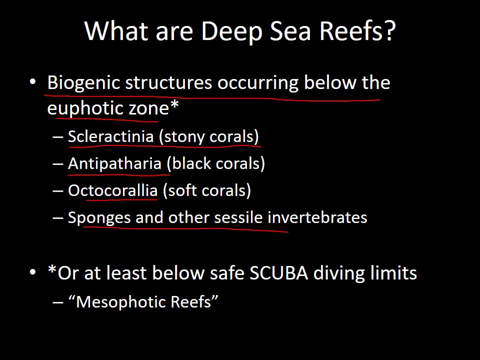 of invertebrates like sponges and other sessile invertebrates that can form biogenic structures in the deep sea and contribute to these reefs. I have an asterisk by deep-sea reefs occurring below the euphotic zone, because there's kind of this. 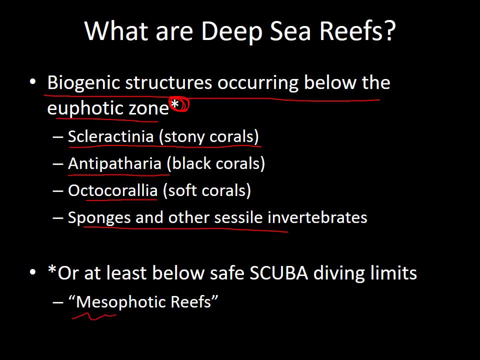 intermediate depth reef, called a mesophotic reef, which is not below the euphotic zone. There is photosynthesis on mesophotic reefs, but the reefs are below safe scuba diving limits, so they're relatively unexplored and we don't know as much about them. 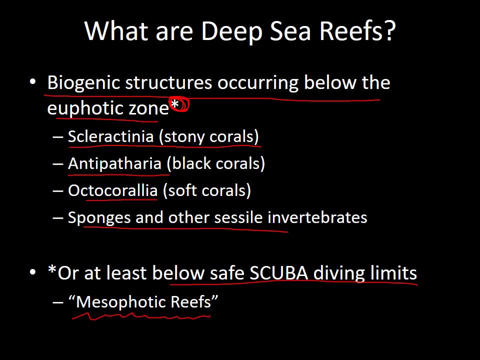 as we do about shallow-water reefs. So before we talk about the really deep-sea reefs, we should talk about these reefs that are in medium-deep water, where there's still some photosynthetic production. Oh yeah, so these corals would be considered. 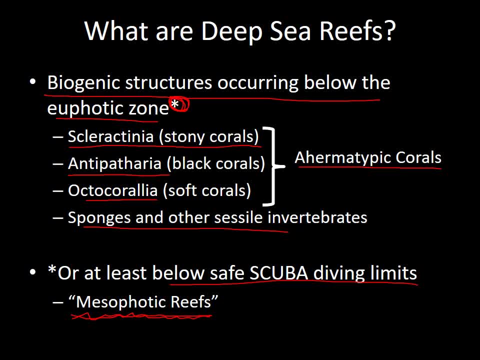 ahermatypic corals if they're on truly deep reefs, meaning that they don't have zooxanthellae, whereas on mesophotic reefs you do have some hermatypic corals, the types of corals that do have. 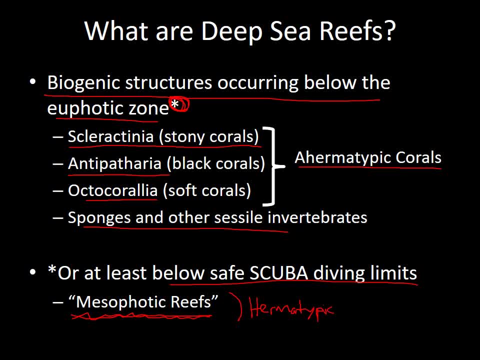 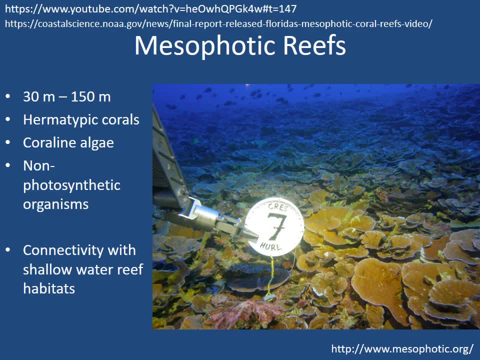 zooxanthellae, and then there's sort of an interesting transition zone where you go from hermatypic corals to ahermatypic corals as you go deeper. All right, so this is a picture of a mesophotic reef. 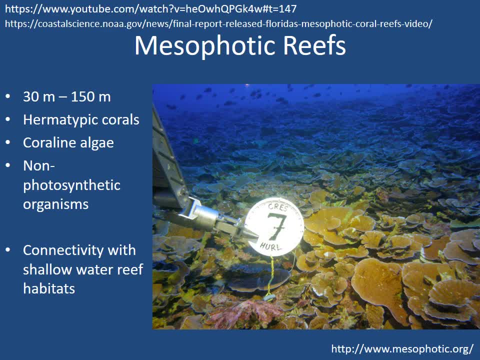 I think this one's in the Hawaiian Islands, but don't quote me on that. I've got some links here that talk and show us about mesophotic reef research, because it's such a growing field, particularly as shallow water reefs are threatened more and more. 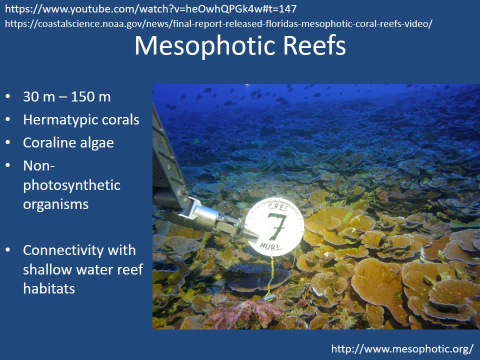 by various anthropogenic destructive forces. We're realizing that these mesophotic reefs in some cases are surviving a little better than the more disturbed shallow water reefs, and we're hoping that they can be kind of like a refuge for organisms that are dying out in shallower waters. 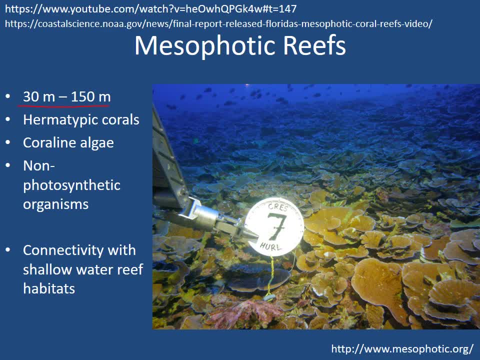 The depth of range that we would consider a mesophotic reef would be about 30 to 150 meters, so the maximum depth that people can scuba dive to is a little over 30 meters. maybe 40 meters, but the lower limits. 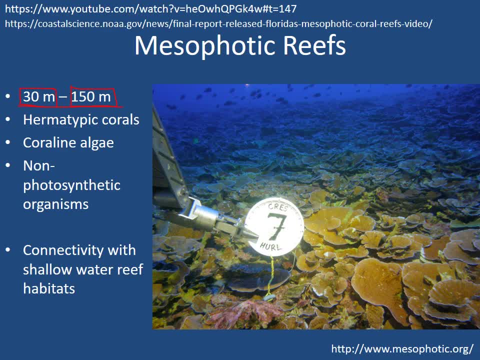 of these mesophotic reefs are quite a bit deeper than conventional diving can go. So they're made by hermatypic corals. so these corals here do have zooxanthellae in them, even though, as you can see, 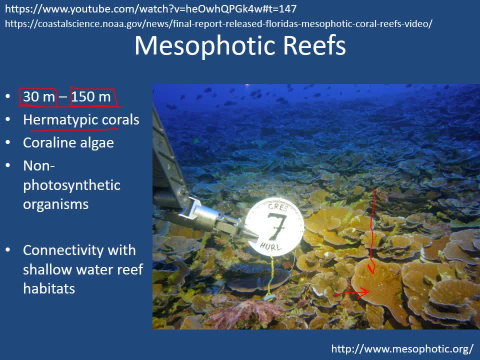 the light is quite dim. It's enough light barely to support the zooxanthellae that are living in these corals. One of the consequences for coral morphology of being in a dimmer light environment is that you need to have more of like. 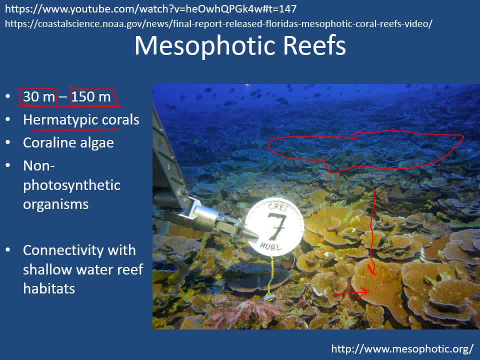 a flat, plate-like structure to try to collect as much of that dim light as possible. So whereas corals in shallow waters might grow more vertically and be like mounds and stuff, corals in deep sea waters would try to spread out horizontally to capture as much light. 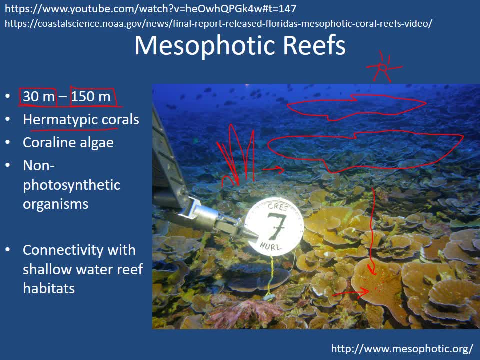 as possible, because light is a more limiting factor. So sometimes even the same species of corals that would be sort of vertically oriented in shallow waters will be more spread out horizontally in deeper waters. So there's hermatypic corals in these areas. 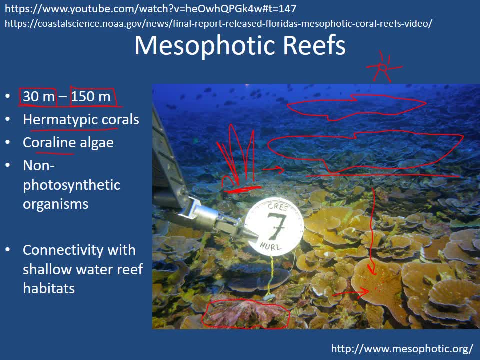 There's coral and algae. You can see some pink crustose coral and algae in this picture here And then there's also non-photosynthetic organisms as well, And the deeper you go, the fewer photosynthetic organisms are still able to survive. 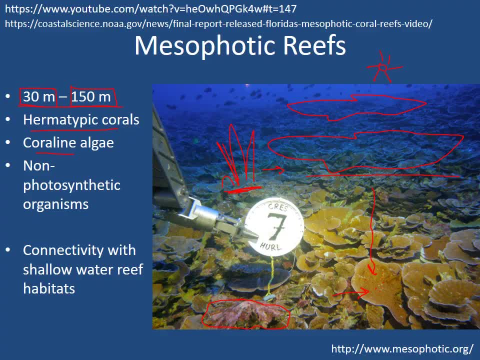 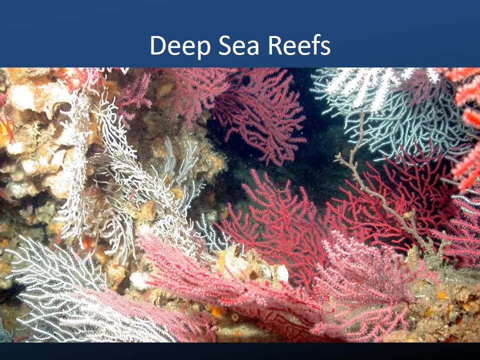 and the more non-photosynthetic organisms you get in mesophotic reefs, All right. so once you get deep enough, there's no photosynthetic organisms whatsoever and you're in a truly deep-sea reef environment where everything is based on. 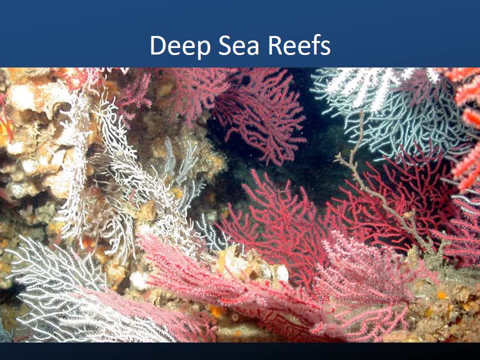 heterotrophic filter feeding. So the It's. I mean shallow water reefs. they also catch particles out of the water with their tentacles, But in deep-sea reefs that's all they do. They Because they don't have. 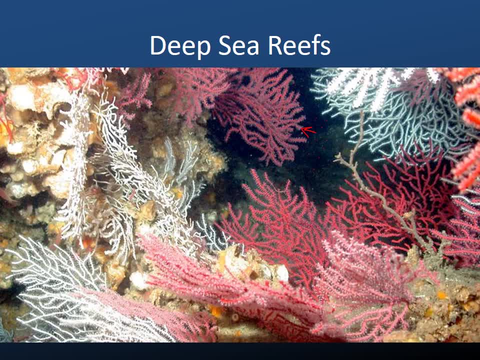 any symbiotic zooxanthellae, But in some areas that's enough, And the deep-sea reefs can be really really lush and diverse in species and high in biomass. They're pretty amazing habitats. As I said here, there's a gradual transition. 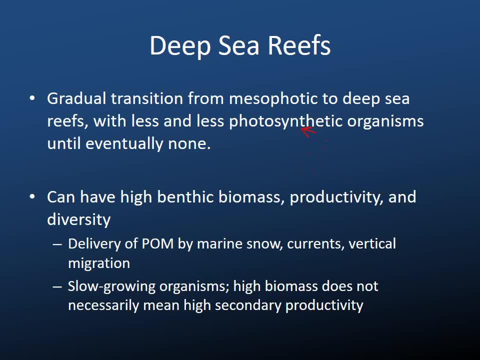 from mesophotic to to truly deep-sea reefs, where there's no photosynthetic organisms And they're supported by the delivery of particulate organic matter, And so where there is a high supply of particulate organic matter. that would be where deep-sea reefs 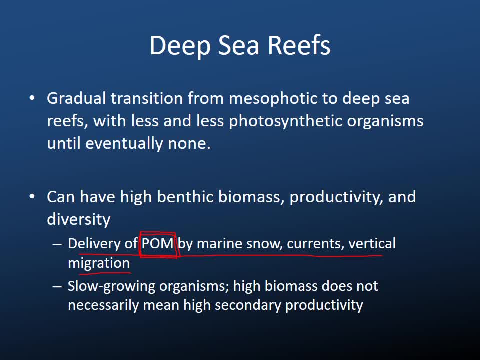 would be most likely to be successful. So where the surface waters are really productive, that could help. the deep-sea reefs, Where there's strong currents that sweep a lot of particulate organic matter into the tentacles of the polyps, that could help. 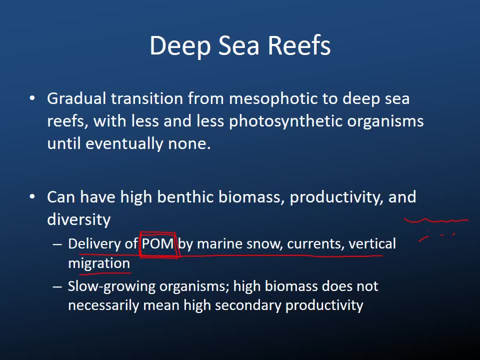 Or where there's vertical migration, so where the plankton communities at the surface are migrating up and down on a daily basis, that could mean that they're. when they migrate down deep, they might be migrating into the tentacles of the deep-sea corals. 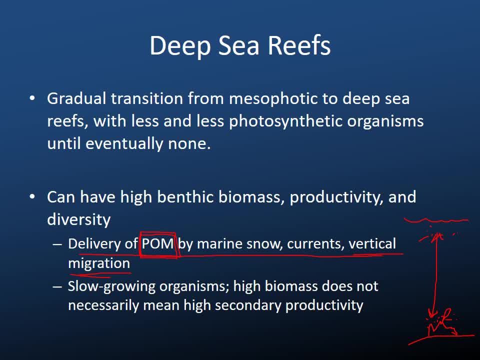 So that could actually. So that's how the vertical migration could help supply plankton to the heterotrophic deep-sea reef organisms. So, even though there can be a lot of biomass on these deep-sea reefs, so lots of coral. 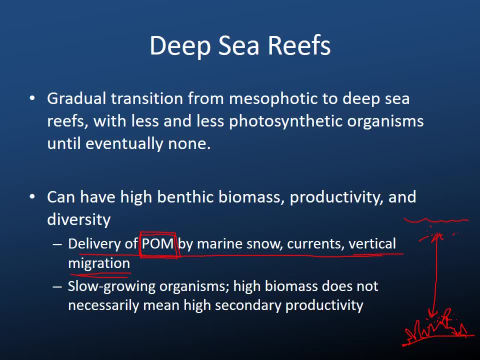 lots of fishes, that doesn't necessarily mean that there's high secondary productivity. These can be environments where species grow really, really slowly, So it takes them hundreds or thousands of years to build up that high biomass. And so, even though it looks like, 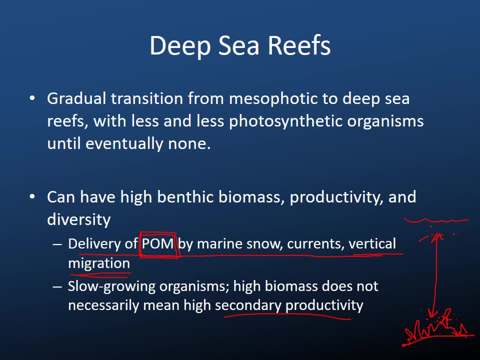 a lush productive environment. it's actually an environment that took a very, very long time to develop that biomass and biodiversity and thus it's very vulnerable to disturbance because it's not going to be able to quickly grow, to recover and regain its biomass and diversity. 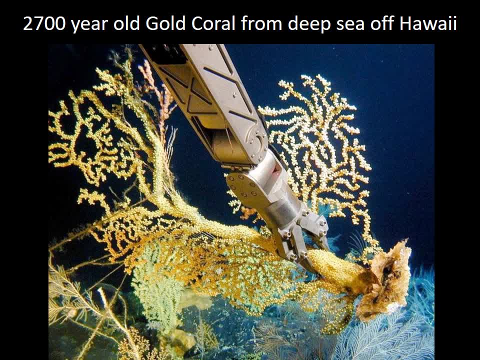 As an example of how slow-growing these deep-sea organisms are, we know by taking core samples from the corals which end up having, If you looked at like a cross-section of a coral, like if you cut this and looked at it. 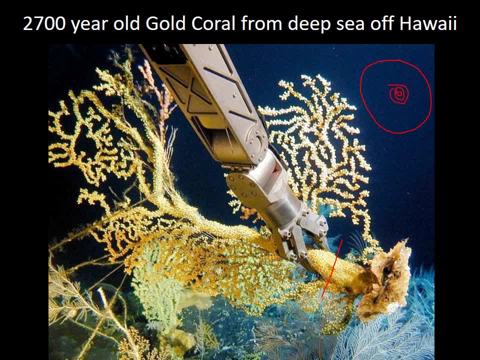 you'd see that it has rings in it and you could count the rings. You'd need a microscope to do it and you would see, Because there's seasonal differences in how fast the corals grow, due to seasonal differences in how much marine snow there is. 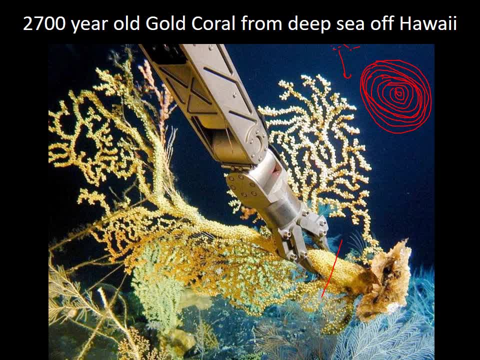 due to seasonal changes in phytoplankton productivity. at the surface. that's what means, That's what creates the differences in the yearly differences in growth rate that lead to yearly rings in the deep-sea corals, And you can sort of count the rings. 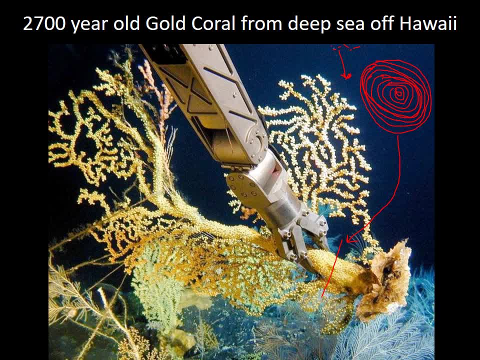 and do different kinds of chemical or isotopic analyses to analyze them, and we know from those methods that some of these corals are extremely old. like this one was 2,700 years old, So I hope the scientists didn't take too many of these. 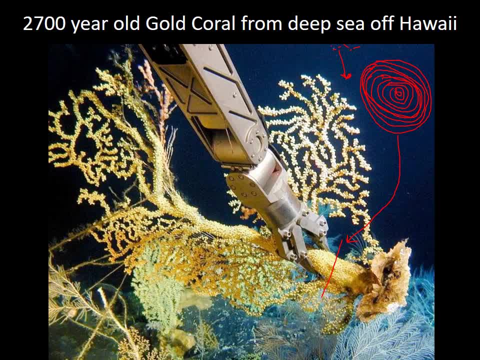 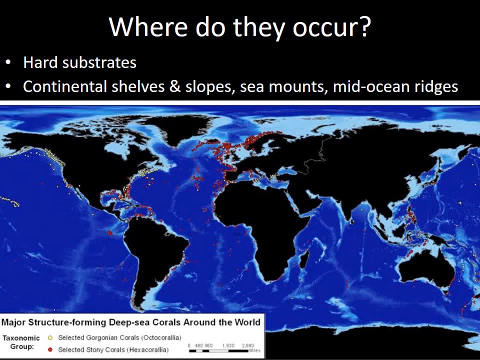 because it'll take 2,700 years for them to regrow. All right, so where are these? These deep-sea reefs are not just found over the entire deep-sea floor. They're only found in suitable areas, so they definitely need a hard substrate. 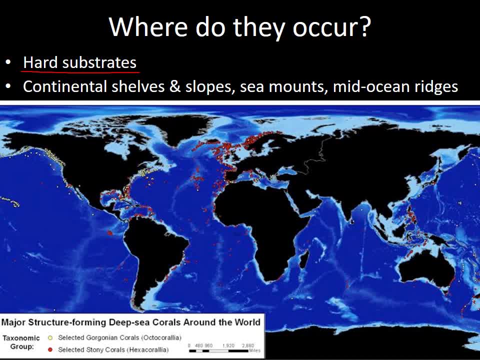 And since most of the deep-sea floor is mud substrate, that rules out most of the deep-sea floor They are found. Where the hard substrates are found oftentimes is along the continental shelves and slopes where the continental shelves drop off into the deep sea. 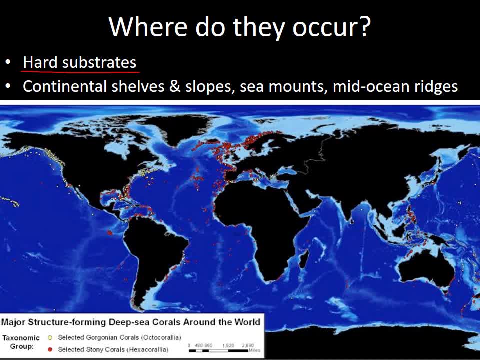 Sea mounts, where there's underwater volcanoes and mid-ocean ridges. These are areas that have steeper slopes, where there's less sediment accumulated, and oftentimes they have strong currents that sweep by those areas and help deliver particles of food, so that helps the deep-sea reefs. 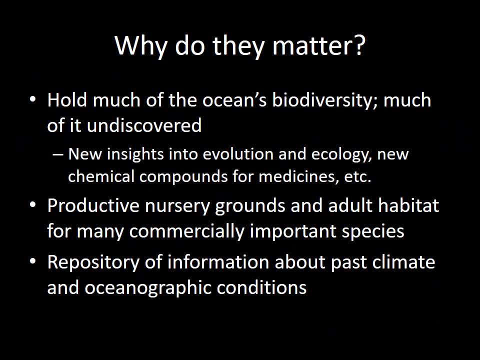 survive and grow in those areas. So who cares about deep-sea reefs? The reasons that we care are because they hold a lot of the ocean's biodiversity. So the diversity of the ocean and the diversity of deep-sea reefs is actually similar to the diversity. 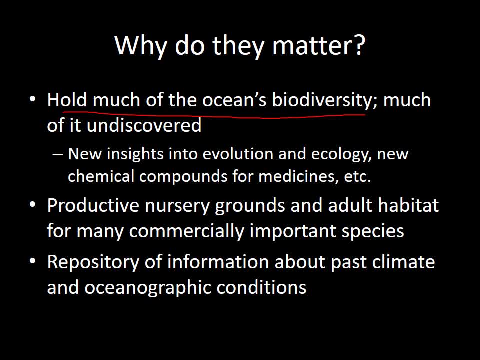 of shallow-water reefs, meaning it's really high And it's a lot of species that are unknown to science currently. Every time we explore these deep-sea reefs, we seem to discover new species, And this means that it's sort of a repository. 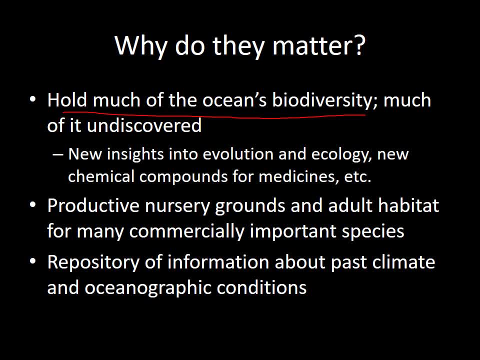 of biological diversity of the Earth, and some of the diverse organisms that live in these habitats could at some point supply us useful chemical compounds for medicines to treat cancer and to come up with all kinds of other potential benefits for humanity. Also, we can learn a lot about 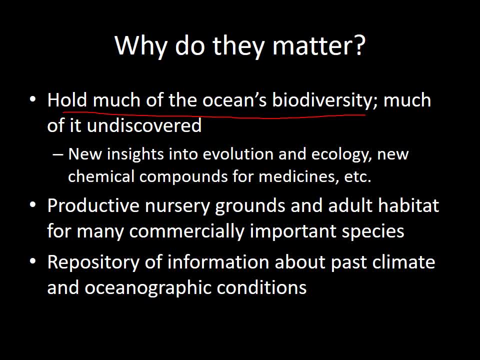 the evolutionary history of life, from what's going on in the deep sea, about the connections between deep-sea communities and shallow-water communities. So there's a lot of scientific insight, some of it just interesting out of a curiosity standpoint and some of it potentially 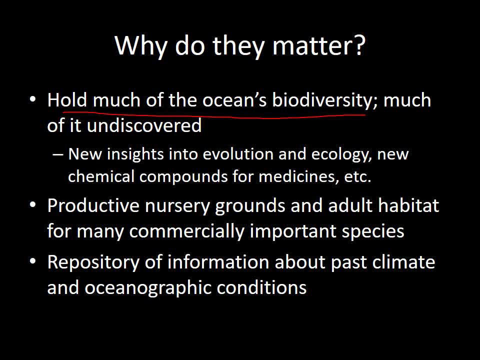 life-saving for humans That we could learn from deep seas, Deep-sea reefs. Also, a lot of these deep-sea reefs are nursery grounds and adult habitat for commercially important species, So lots of fish and crabs that we eat are dependent on these deep-sea reefs. 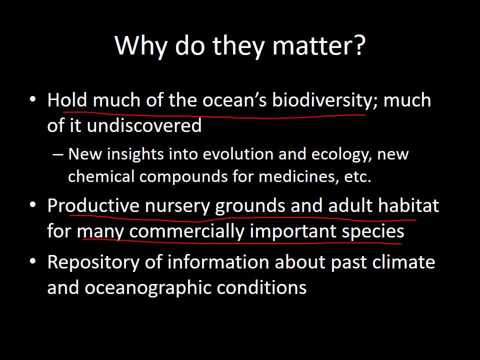 for their breeding grounds And the deep-sea reefs. because of the way they've been there for so long, slowly growing and recording in their rings information about the ocean conditions or the past. We consider them to be a repository of information about past climate. 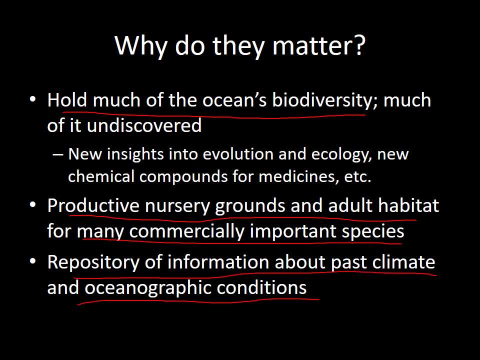 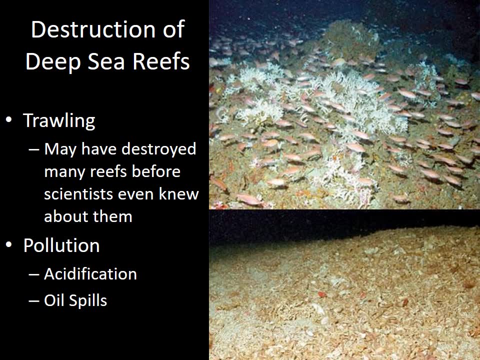 and oceanographic conditions that can help us predict and understand how ocean ecosystems may change with future climate and ocean changes. So it's really sad, then, because of all these values of deep-sea reefs, that deep-sea reefs are being destroyed going from this to this. 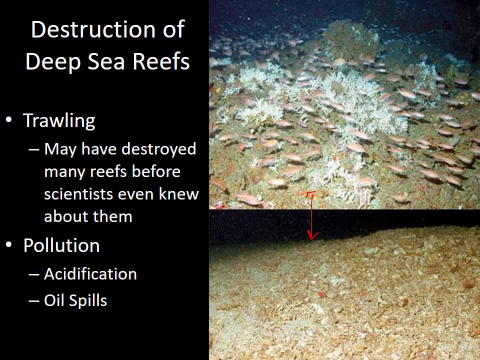 at a shockingly rapid rate, And one of the main disturbances is trawling. So because deep-sea reefs are full of fish, trawler fishermen will drag their nets over them and that destroys all the coral, and the coral does not grow back fast at all.